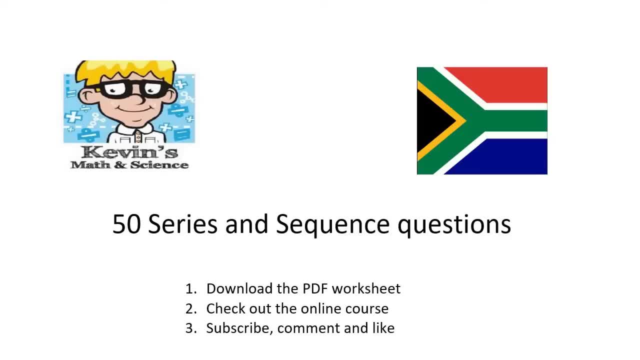 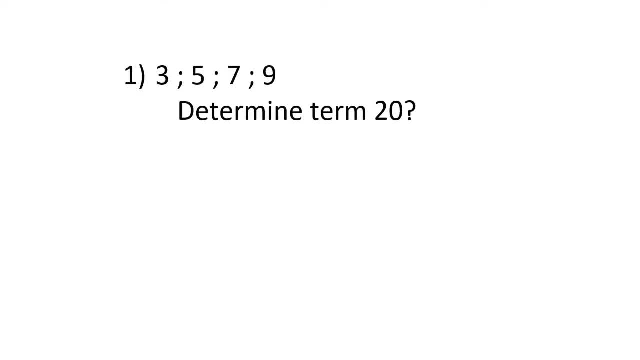 algorithm pays attention to these types of things And it starts promoting the A, the common difference, which is 2, because you can see we're plussing 2 each time. Your answer is 41.. For number 2,, you need to realize that this is also an arithmetic sequence. 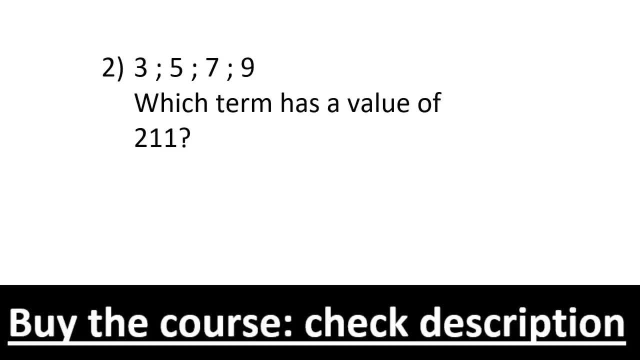 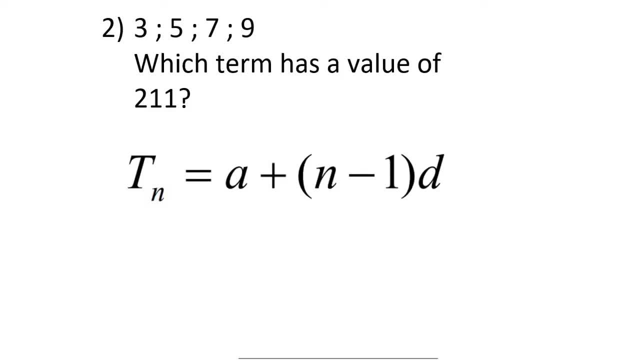 In fact it's the same arithmetic sequence from question 1, but now they're saying which term has a value of 211.. So now we know the answer. So we put the 211 over here, A we don't no. 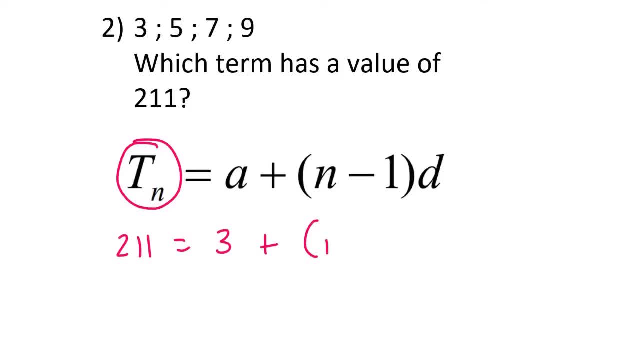 we do know. sorry, We don't know the term, which term number we have. So we're going to just say n over there, and then the common difference is 2.. Now what I would do is I would take this: 3. 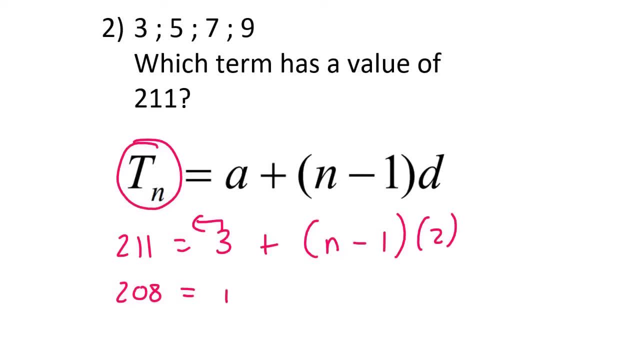 over to the left, so it'll become 208 equals to n minus 1 times 2.. Now, of course, you can multiply the 2 into the bracket, but what I like to do is divide by 2.. So we end up with 104 on. 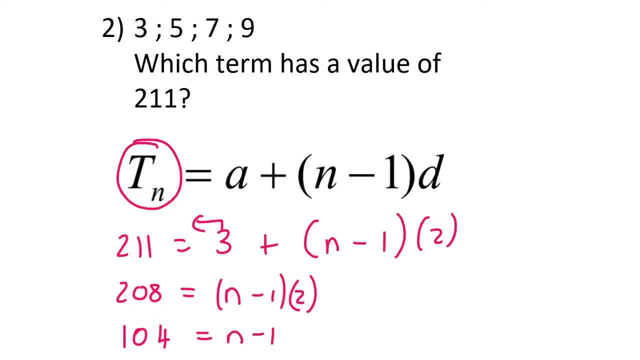 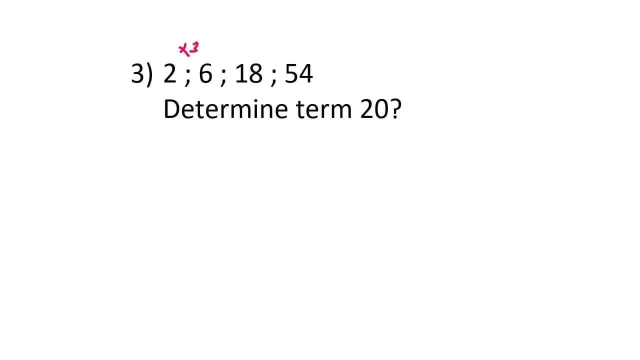 the left-hand side equals to n minus 1.. Then to get n alone, you take the minus 1 over, and so therefore we should end up with n equaling 105.. Question 3 is a geometric sequence. We can see that we are multiplying by 3 to go from each term or from one term to the next, So we need to. 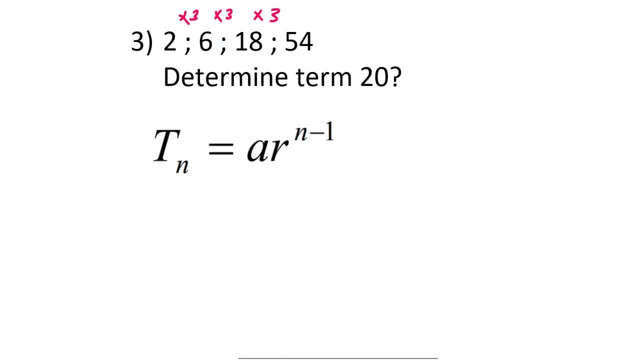 use the geometric formula, And so we're looking for term 20.. So we can say t20.. A is always your first term, which is 2.. R is the common ratio. If you battle to figure R out, you can always say: 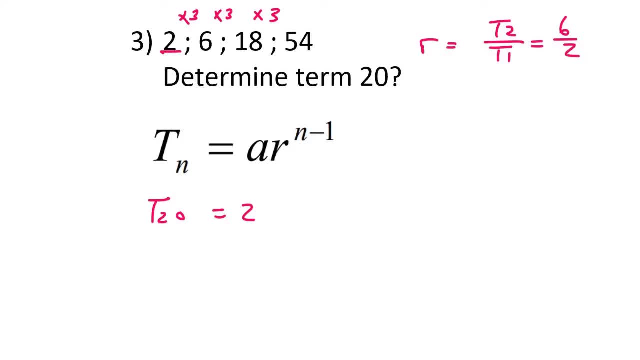 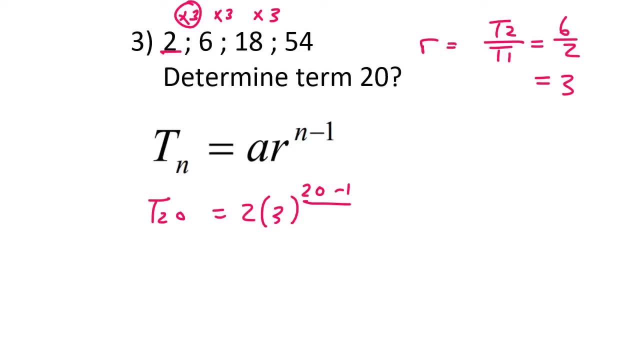 that's not correct. That 3 has an exponent, And so you rather just want to go ahead and type this on the calculator exactly as you see it, And this will give an answer. Oh, it's quite a big answer. 9, 3, 4.. There's the answer for that one In question 4, we have the same sequence that we. 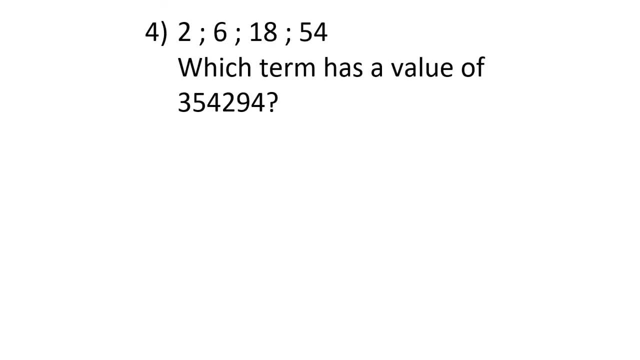 saw in question 3.. So we know that it's geometric. But now they're saying which term has a value of, and then they give us a big number. So we use the geometric formula And we already know the value. So what we do is we say 3, 5, 4, 2, 9, 4 equals 2.. Now A is your first term, which is 2.. R is 3.. 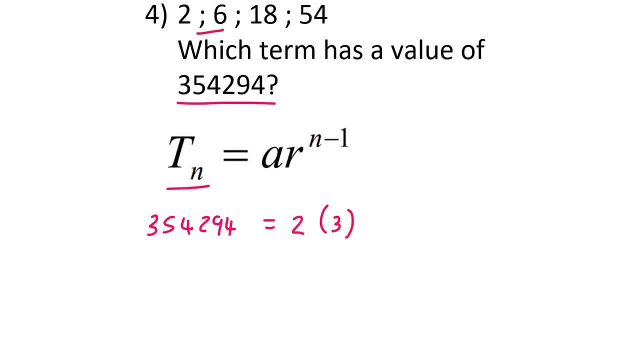 How do I know that R is 3?? Because I can see that they are multiplying by 3 when going from one term to the next. If you battle to find that you can just say t2 over t1, which is going to be equal to 6 divided by 2,. 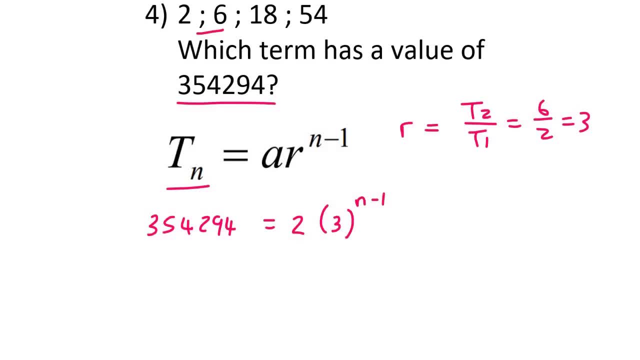 which is 3.. Then n? we don't know, So we do that. Now, what a lot of students do is they multiply these two together and they call it 6. That is not correct, because this n minus 1 is only an. 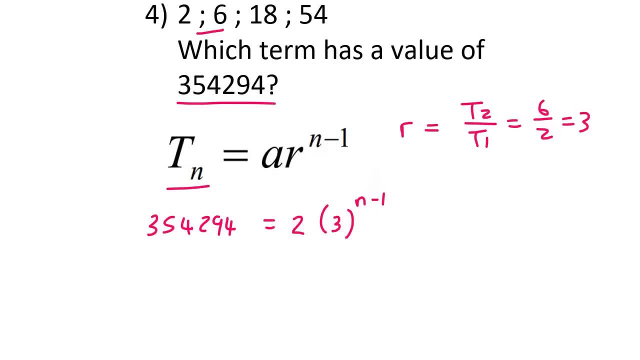 exponent for the 3.. So what we can do now is we need to try to get n minus 1.. And we can do that with n by itself. So what I like to do is I divide by 2 first, on the left-hand side, because that 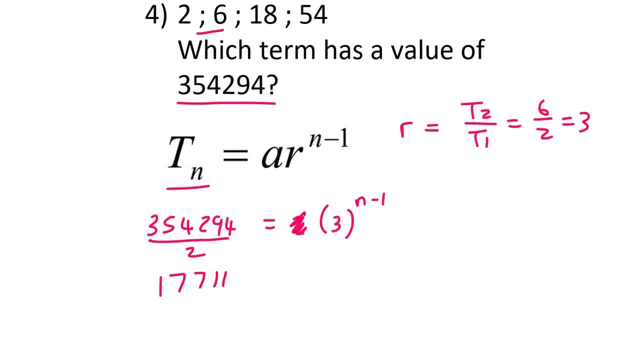 gets rid of this, And so that's 177147 equals to 3 to the n minus 1.. What you do then with this number here is you break it up into its prime numbers, Or you can use logs. Any approach will give you the same answer. So I'm going to actually show you both methods. I'm going to use the prime. 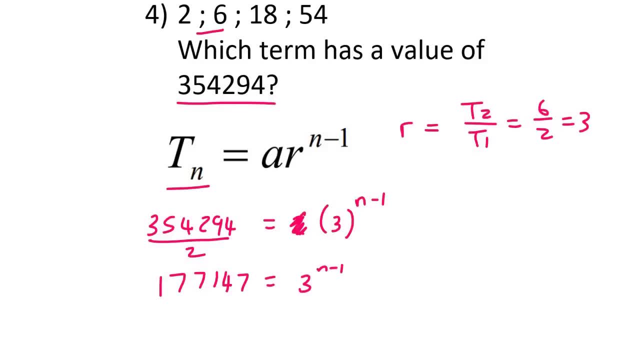 factor method first. So if you have a Casio calculator, you just type this number in on your calculator, the 177147.. You then say equals, You then push the button shift And then you look for the button that says fact And that gives you 3 to the 11, equals to 3 to the n minus 1.. Now these 3s are the same. 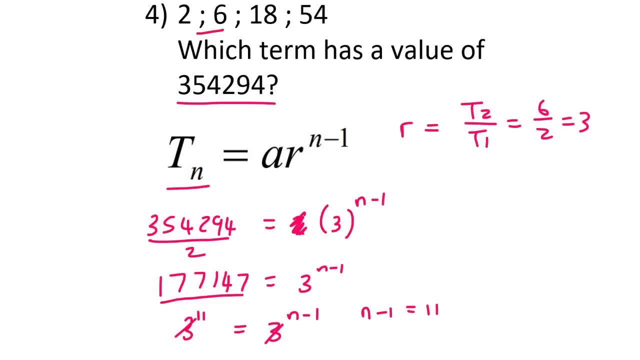 so they cancel out. And so we would say n minus 1 equals 11.. If you had to get n by itself, you should get 12.. Let's use the log method. With the log method, you would come up to here and you would say: 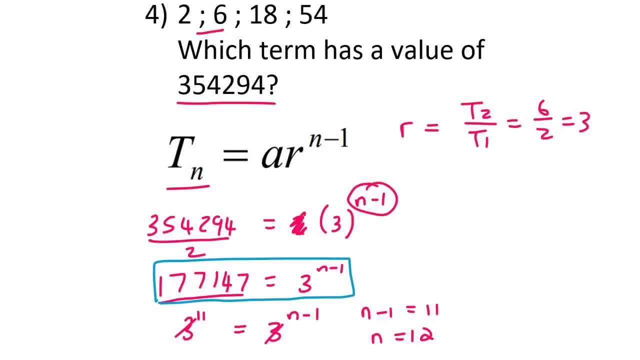 the exponent, which is n minus 1.. Actually, let me do this in a different color. So you would say n minus 1 equals to the log. Now the number that was with the exponent comes first and then the other number comes next, So it's 177147.. Go ahead, type that in. 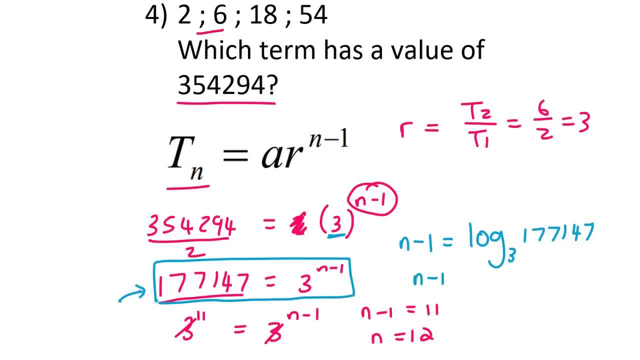 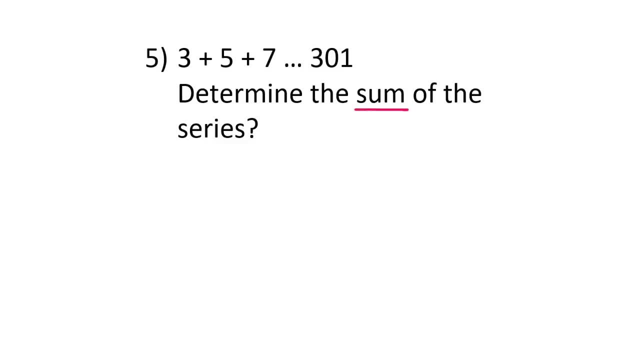 and that gives us 11.. And then, of course, if you take the minus 1 over, you get 12.. Question 5 asks us to determine the sum of the series. By the way, does it ever bother you why sometimes we call it a sequence and sometimes we call it a series? 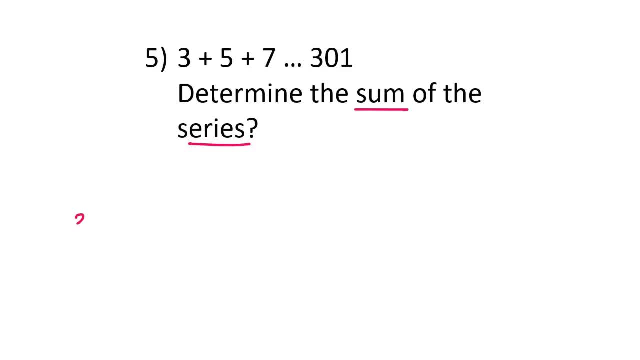 Well, actually what is happening is the following: If I write the numbers like this- see how I separate it with a semicolon- then we call this a sequence. If, instead, I plus the numbers together, then I just call it a series. That's all. So in this question, they want us to. 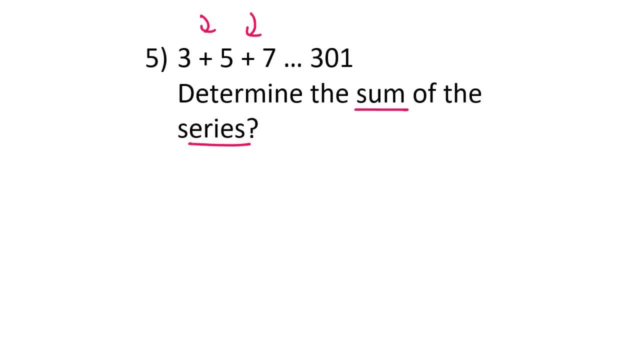 calculate the sum. We can also see that it's an arithmetic pattern, because you are plussing 2 each time. So we would use the sum formula for an arithmetic pattern. However, we do not know how many terms we have. We don't know n. So what you do in a question like this? 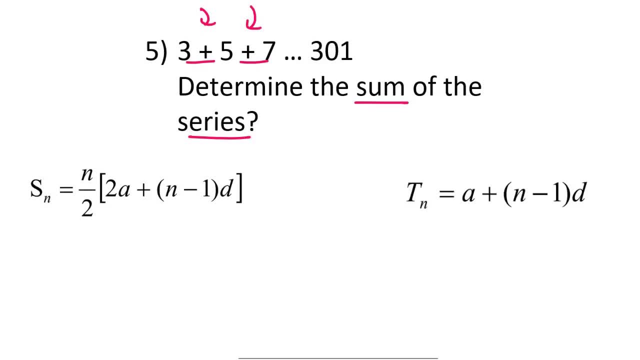 is. you use the tn formula and we know that the last term is 301. So we put the 301 over here, and then a is 3.. We don't know how many terms there are, and then the common difference is 2.. We can then solve this by moving the 3 over to the left hand side, which will become 298. 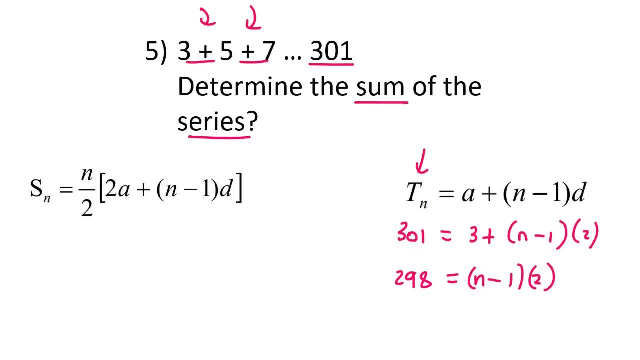 equals to n minus 1 times 2.. Now you could multiply the 2 into the bracket, but what I like to do is divide by 2 on the left instead, And so that'll give us 149 equals n minus 1.. And so, if we solve for n, 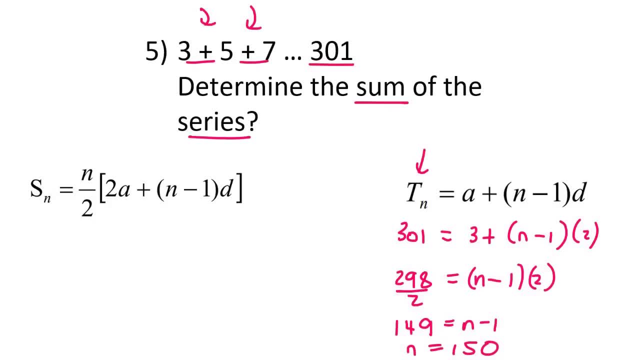 we will find that n is equal to 150.. This means we have 150 terms, Because we were using the last term and we found out that it's at position 150, it means that there should be 150 terms. Now we can come back to this formula. 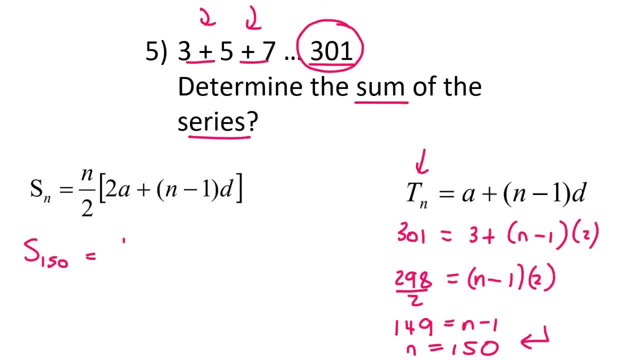 And so we can say: s of 150 terms is 150 over 2. 2 times a, which is 3, plus 150 minus 1. And then our common difference is 2.. Go ahead, type that all in on the calculator and you get an answer of 22,800. 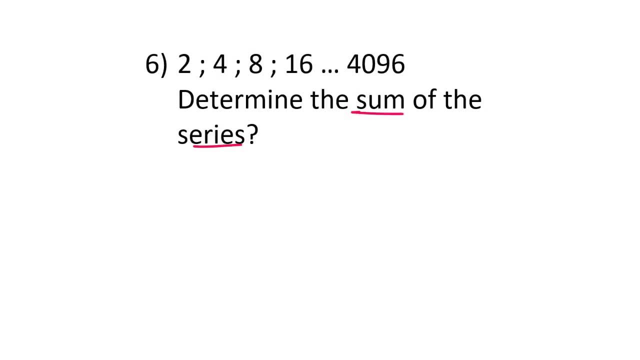 Question 6 asks us to determine the sum of the series. Now we should realize that this is a geometric sequence. You might think that it's arithmetic, because you probably don't know the pushing 2 over here, But then it doesn't plus 2 when you go to the next one. 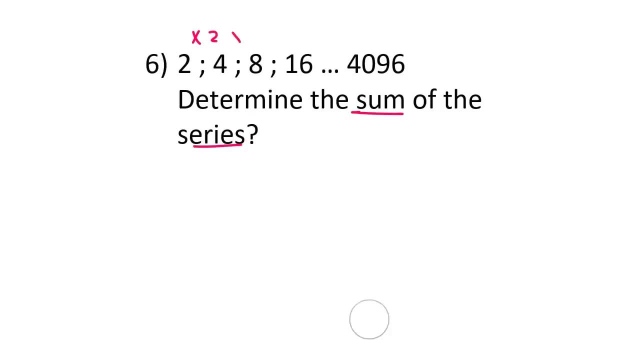 However, can you see that we are multiplying by 2?? Can you see that If you are unsure how to work your ratio number, all you do is you take term 2 divided by term 1, and so in this case, that would. 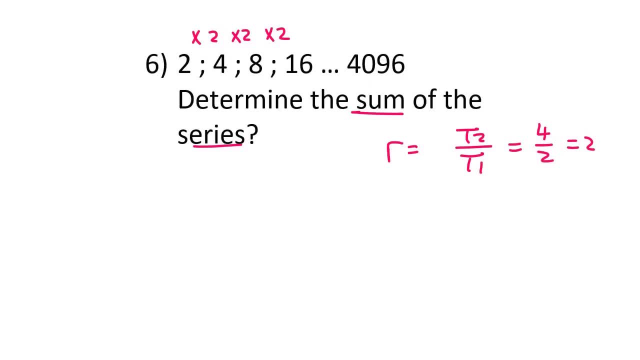 be 4 divided by 2, which is 2.. So because it's geometric, we need to use the geometric sum formula. However, there is one problem: We don't know how many terms we buy. So we take the programmes of the series and we add, including numbers of thirdادом and when that's settling, so it would. be 4,, which is 7, and we add two on top of that, and so on, until we reach the problems we have in therico我覺得 that we don't know how many terms there is worth, And so if it can't, be increases. 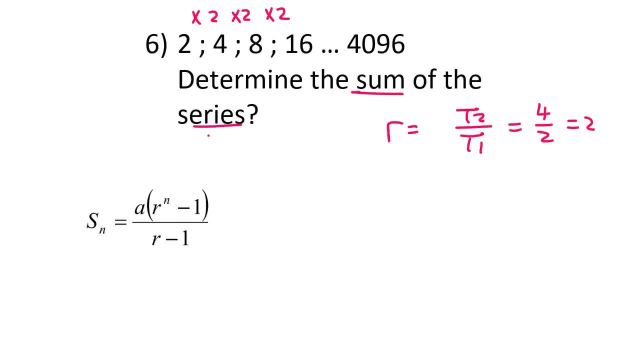 don't know how many terms we have, but what we do know is that the last term is equal to 4096.. So we can use the TN formula and we could put the last term as 4096, then A is 2, your common. 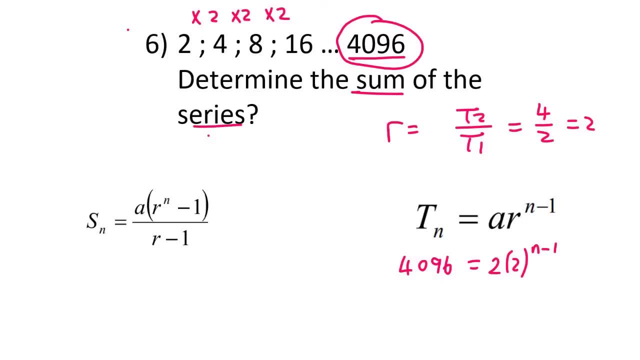 ratio is 2, and then we don't know what N is. Now remember: what some students like to do here is they multiply these two together, but that is not correct because of this exponent. So what we do instead is we rather divide this two on the other side, then 4096 divided by 2, 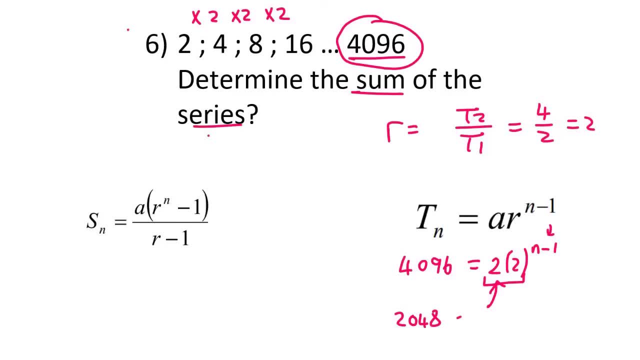 is 2048.. Now here is where you have two options. You can either break the number 2048 up into its prime numbers, or you can use logs. I'm going to use the prime number method. So what I do is I type this number in on my calculator, I then push equals. I then push. 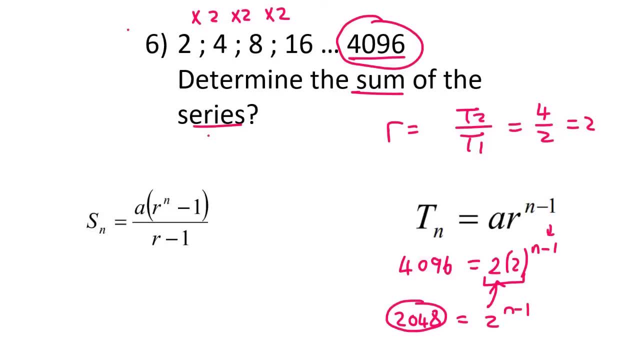 shift, and then I look for the button that has fact, And if you do that, you should end up with 2 to the power of 11.. Now the twos cancel out. so we can cancel those out, and so we have N minus. 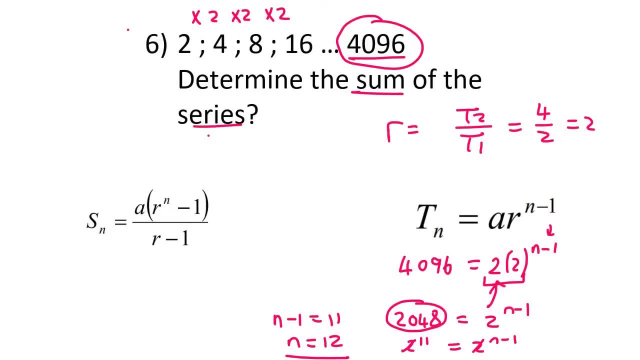 1 equals 11.. If you solve for N, you get 12.. That means that this 4096 is at the top of the number. So what I do is I type this number in on my calculator, I then push equals, I then push shift. 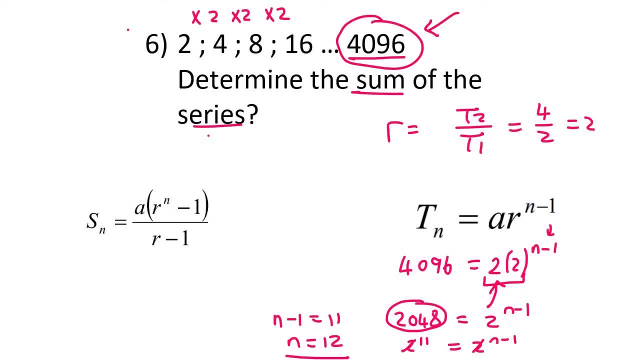 position 12.. But because it's the last term in the sequence, it means we have 12 terms. Now we can use this formula here, And so the sum of 12 terms is going to be A, which is 2.. The common ratio was: 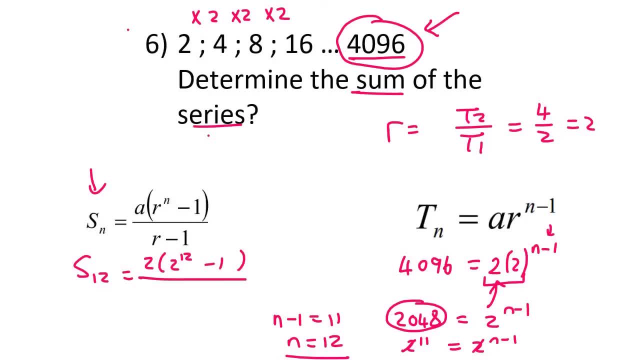 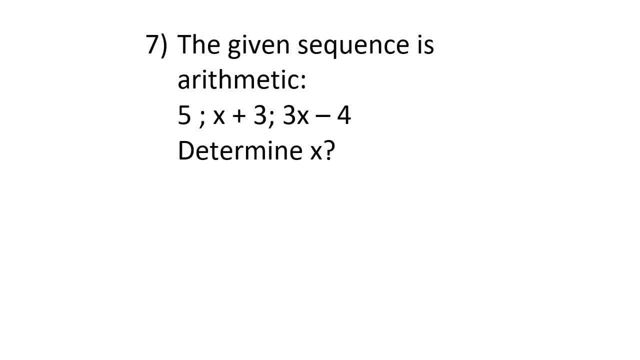 So whenever we get a question like this, all that you need to do is you need to say: term 3 minus term 2 is the same as term 2 minus term 1.. Do you understand what that even means? though Let me show. 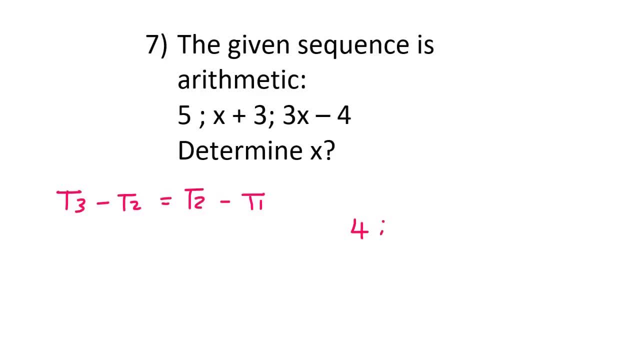 you, If we have an arithmetic sequence like 4,, 7,, 10, and yeah, let's stop there, So that's a 10.. What is term 3 minus term 2?? Well, that's 10 minus 7,. 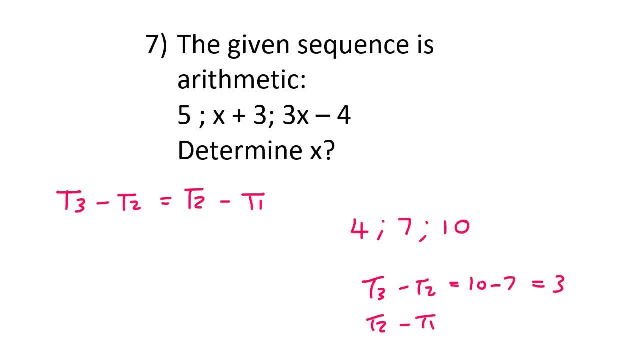 which is 3.. What is term 2 minus term 1?? Well, that's 7 minus 4, which is 3.. So what we are trying to say is that this is a property of all arithmetic sequences, because the difference between the terms stays constant. Can you see how we got 3 and 3?? And, of course, 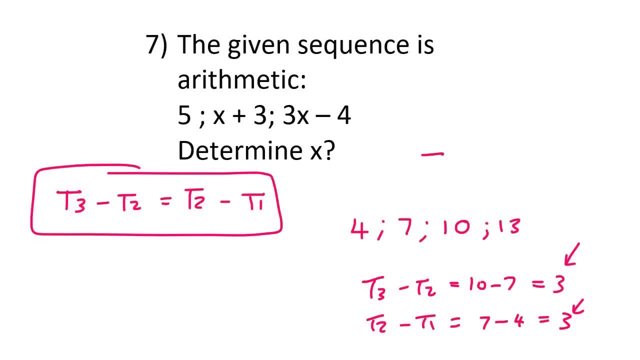 if we had to keep going, this would be 13.. So we could say term 4 minus term 3 would be 13 minus 10, which would also be 13 minus 10.. So we could say term 4 minus term 3 would be 13 minus 10,. 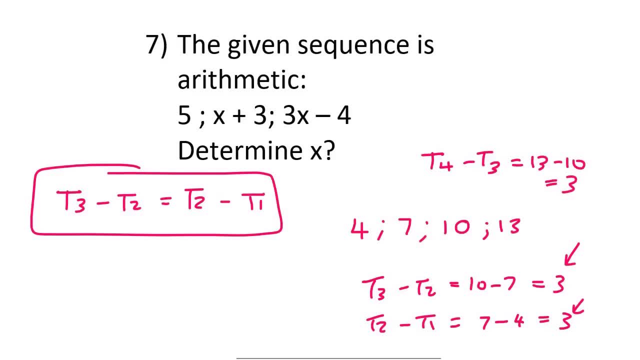 which would also be 3.. So it's actually a very easy to understand concept. Now what we do is we just say term 3, which is 3x minus 4 minus term 2.. Because term 2 is more than one term and we're putting a minus. we should use a bracket. 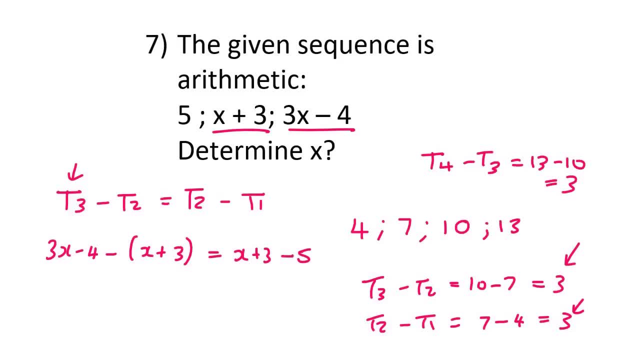 Now term 2 is x plus 3 minus 5.. We can now go ahead and solve: On the left we would eventually have 2x minus 7, and on the side we'd have x minus 2. If we then solve this, we should end up with x equals 5.. 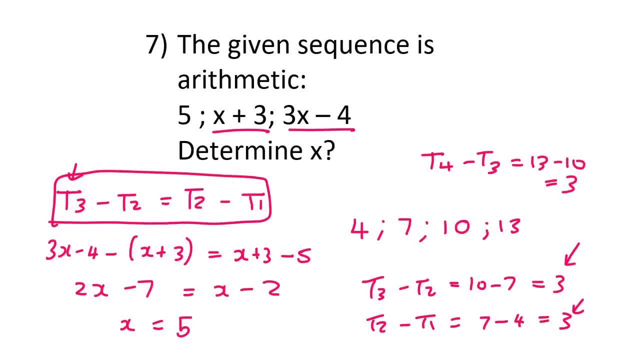 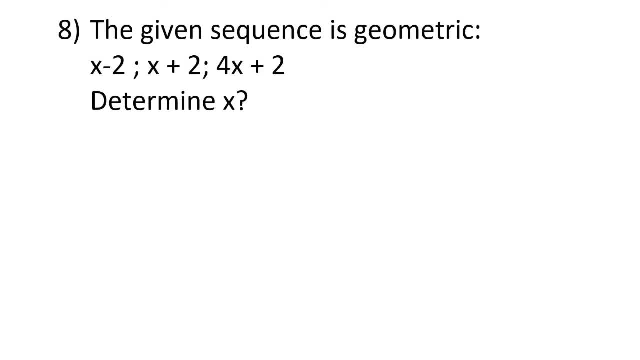 Over here, by the way, when I did this. you can also say t2 minus t1 first, It doesn't matter. In question 8, we are told that this sequence is geometric, and they give us a whole lot of x's. 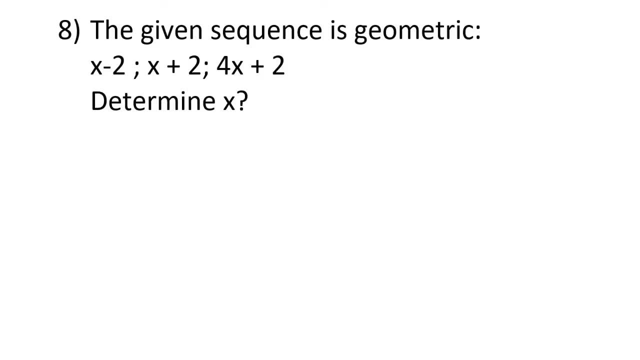 and they say: determine x. Well, the trick that we do for geometric is we say: t2 over t1 equals to t3 over t2.. remember, when we did the arithmetic one in question seven? because it was arithmetic, we rather said something like this: Okay. but when it's geometric, we rather say this: Do you know why? Well, let me. 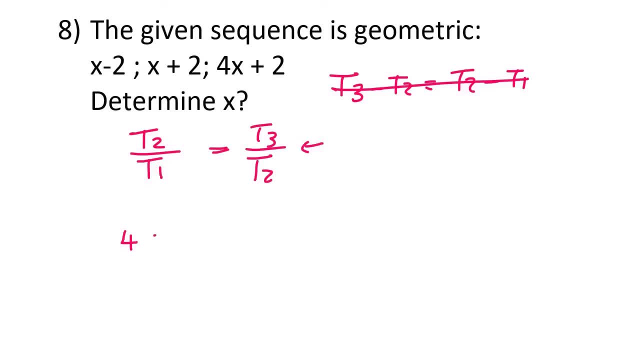 show you. If we have a simple geometric pattern like 4,, 12,, 36, where I'm multiplying by 3, if I take term 2 divided by term 1, that'll give me 12 divided by 4, which is 3.. If I say: 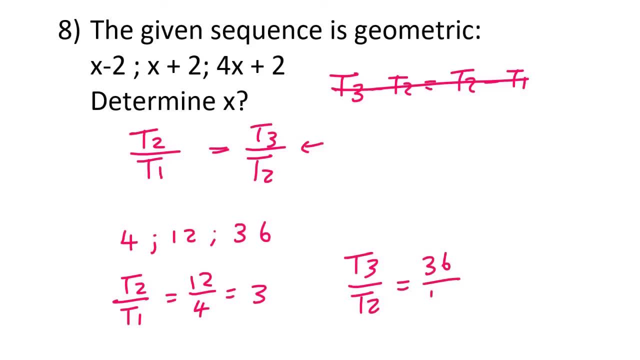 term 3 divided by term 2, that would be 36 divided by 12, which is 3.. Can you see that it carries on producing a 3?? So the ratio stays constant. So for any geometric pattern you can say this: Now, all you do is you go fill everything in. So term 2 is x plus 2,, term 1 is x minus 2,. 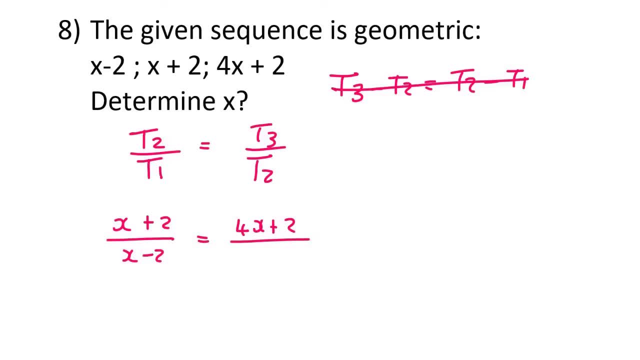 term 3 is 4x plus 2, and term 2 is x plus 2.. What you now do is cross multiplication. So on the left, you're going to have x plus 2 and x plus 2.. And on the right, you're going to have 4x plus 2 and x minus 2.. Now we're just going to multiply. 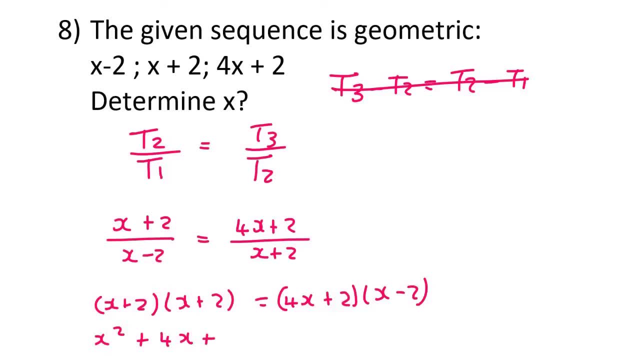 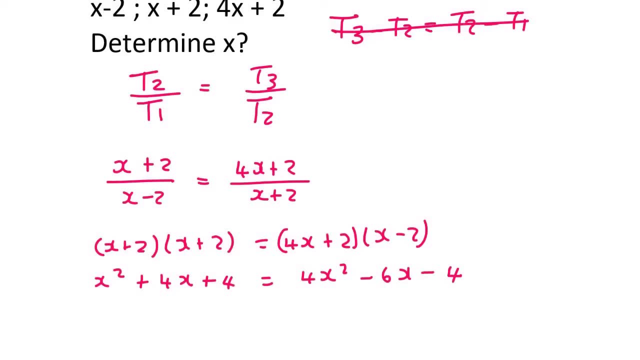 everything out. I'm just going to do this fairly quickly because you guys should be comfortable with minus 6x minus 4.. I'm going to take everything to the right-hand side because I would like to have a positive x squared, just because I find that more comfortable. You don't have to do it. 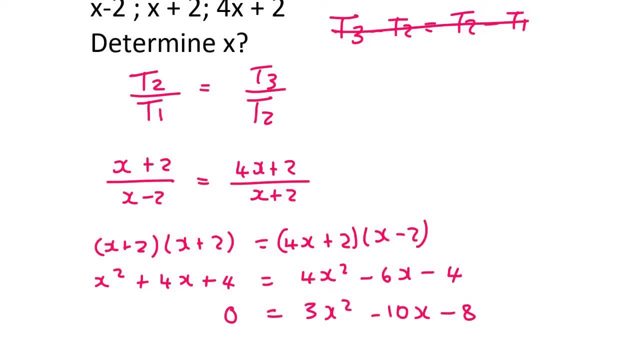 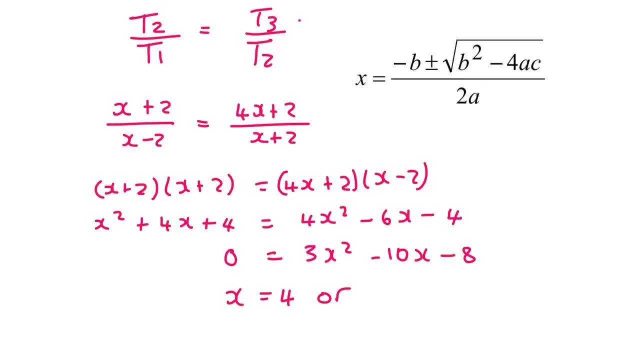 that way, And so this is what you should end up with Eventually. Now you can try factorize this if you would like. I'm just going to use the quadratic formula, And once you use the quadratic formula, you should end up with x equals to 4 or x equals. 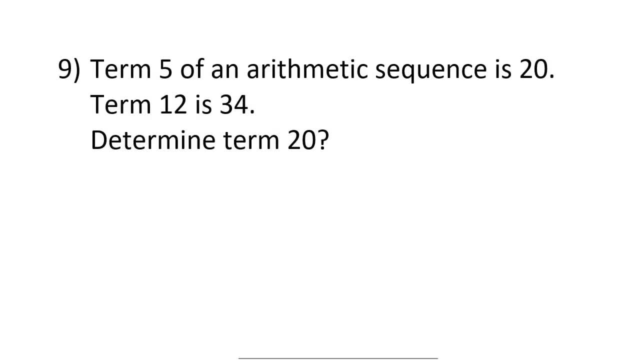 to negative two-thirds. Question 9 tells us that term 5 of an arithmetic sequence is 20, term 12 is 34, determine term 20.. Now I find a lot of students. they try to work this out. They literally like I don't know. they say x, y, z, w, And then they're. 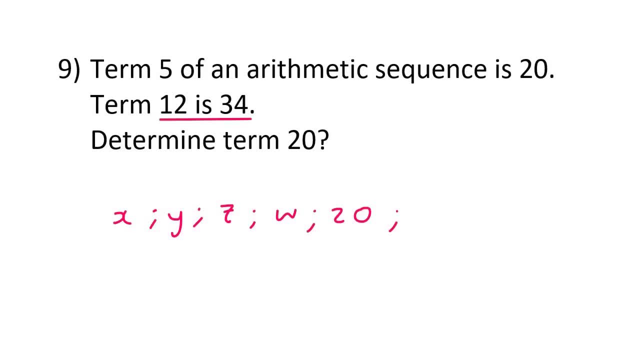 like: oh, term 5 is 20.. So we'll put a 20 there, And then they go all the way up to like term 12.. Guys, this doesn't work. There's a much better way to do this. They're telling you it's arithmetic. 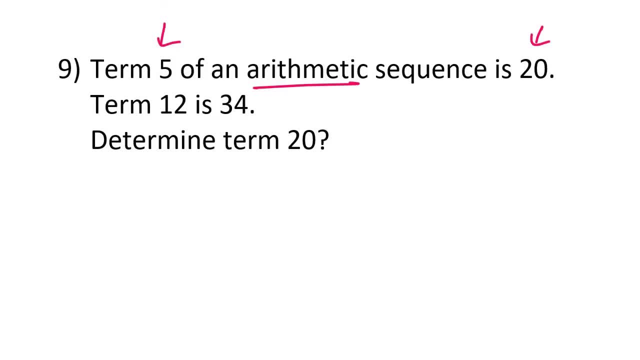 and they're telling you that term 5 is 20.. So I'm going to fill in as much as I can. So they're telling me that term 5 is 20.. So I say 20 equals to a, which I don't know. 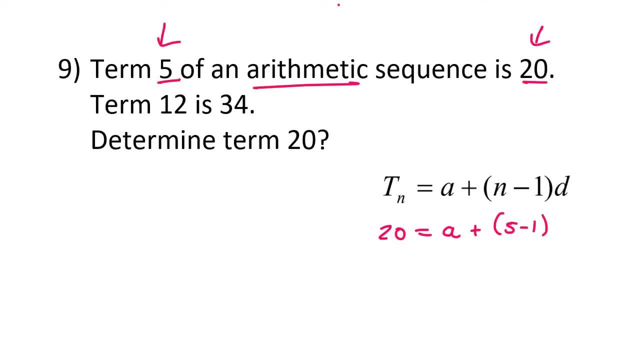 n is 5, because that's the term number or the position number, And then the common difference, I don't know. So then that just becomes a plus 4d. Now I can't do anything more with that, But they've given us another piece of information So I can do the same thing. I can say 34. 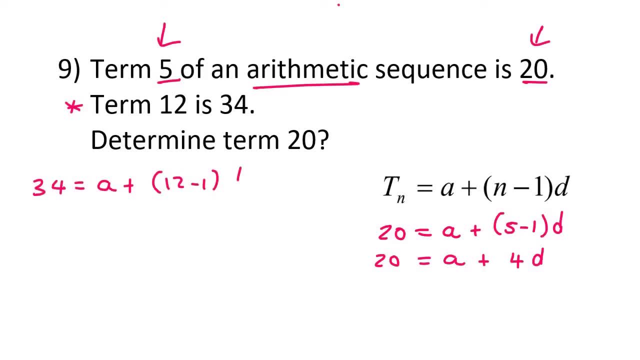 equals to a plus 12 minus 1 times d, And so that becomes 34 equals to a plus 11d. Aha, Now what we can do is we take this equation and this equation and we simply solve simultaneously. Now you can do. 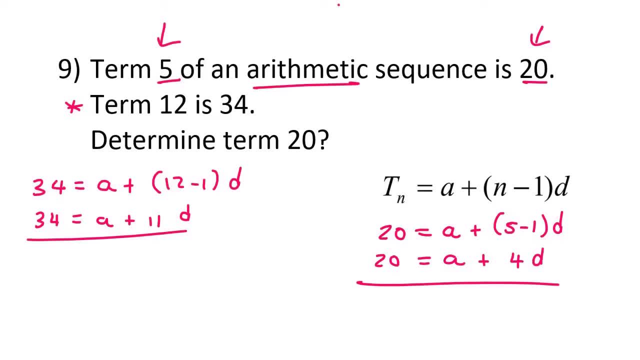 this in so many different ways. So if you don't follow what I'm doing, try it your own way. Just make sure you get to the same answer. So what I'm going to do is I'm going to take this equation and I'm going to get a by itself. If you do that, you would get 34 minus 11d. I'm then going to 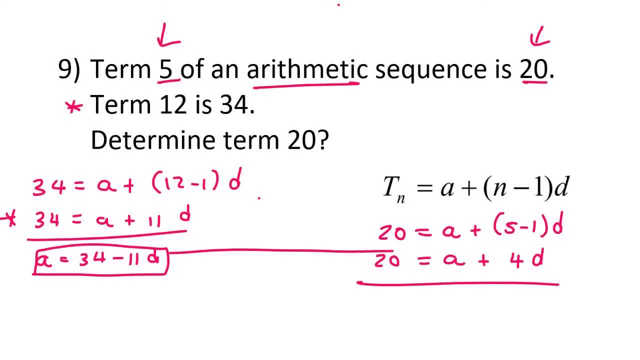 substitute that into the place of a over there. So that means we're going to get 20 equals 2. And then in brackets I'll just say 34 minus 11d plus 4d. Now I can go solve for d. 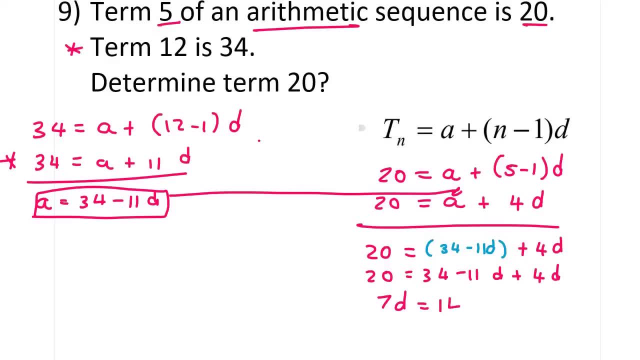 You would eventually find that 7d is equal to 14, which means that d is 2.. I can then plug that back over here as a 2.. And then, if you have to solve that, you'd find that a is 12.. Now they said find term 20.. Now it's easy, We just use. 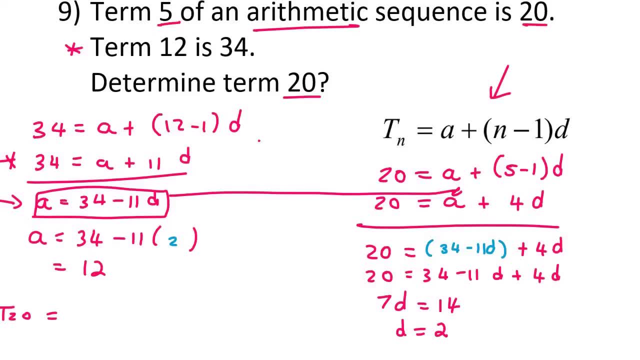 this formula where we say term 20 is a, which is 12, plus 20, minus 1, times d, which is 2.. And so that will be 50.. So, guys, something very important that I want you to understand is that when they give you this information like this, just put it into formulas and it usually 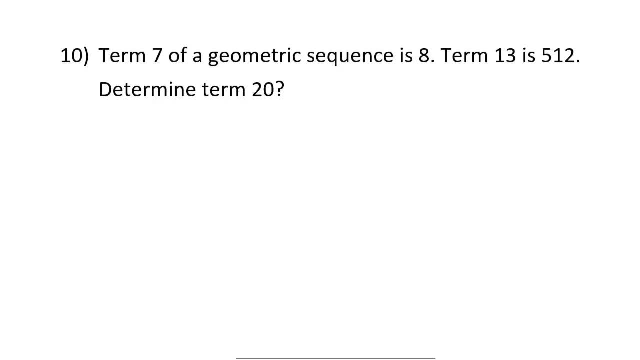 turns into a simultaneous Question. 10 tells us that term 7 of a geometric sequence is 8 and term 13 is 512.. Determine term 20.. Now, if you watched my previous question on question 9, I said how a lot of students do. 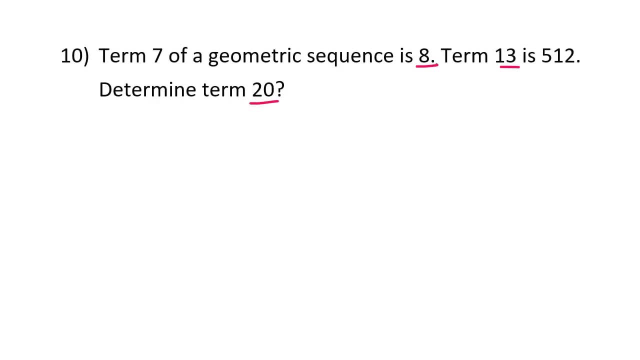 sometimes struggle with these questions because they try to figure it out in their head and they do all these weird kind of stuff. But all you need to do is use the formula. So they say that it's geometric, And then you just fill everything in. So they say: term 7 is equal to 8.. So you say 8 equals to a. 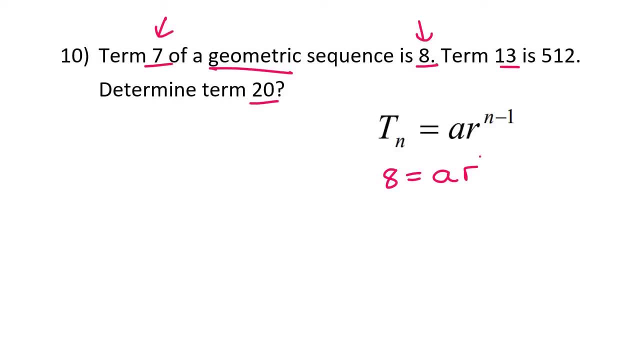 we don't know r, we don't know It's term number 7. So we say 7 minus 1.. And so we can just neaten this up a little bit: 7 minus 1 is 6.. There we go. We can't go any further. So then what we do is we: 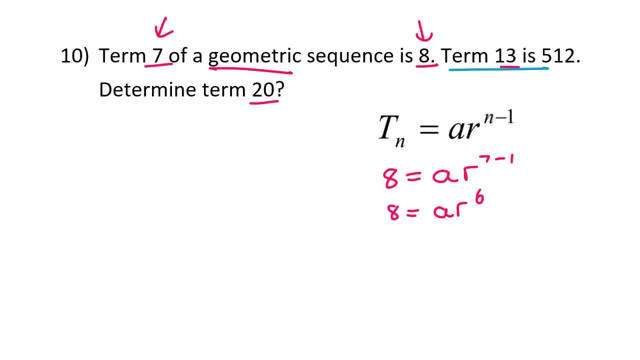 go to the next piece of information, which tells us that term 13 is 512. So we say 512 equals to a r 13 minus 1.. And so I'm just going to simplify That to become 12.. There we have two equations with two unknowns. Now some students battle with 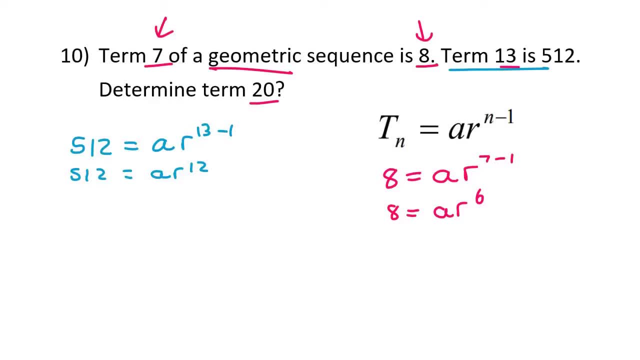 this part, But all you need to do is get. what I would advise you to do is get a by itself, either using this one or using this one. You could get r alone, but it wouldn't be nice, So I'm going to get a alone here by saying 8 over r to the 6.. Now I'm going to take this: 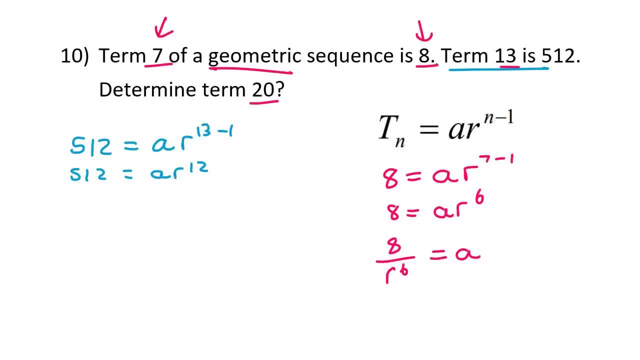 and plug it into the place of a over here, And so that's going to be 8 over r to the 6.. So that's going to be 8 over r to the 6.. And so that's going to be 8 over r to the 6.. 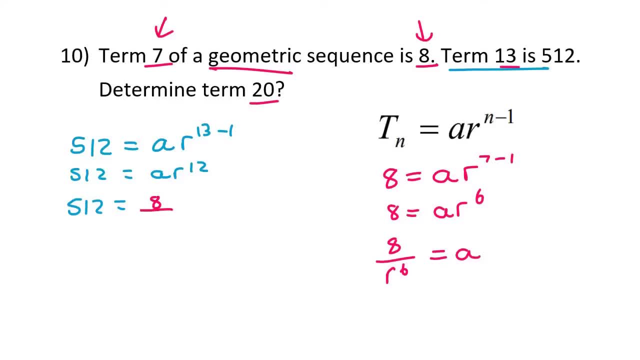 So I'm going to say: 512 equals to a, which is now 8 over r to the 6. You can put it in a bracket, if you want, multiplied by r to the 12.. Now students always ask me: OK, Kevin, what do we? 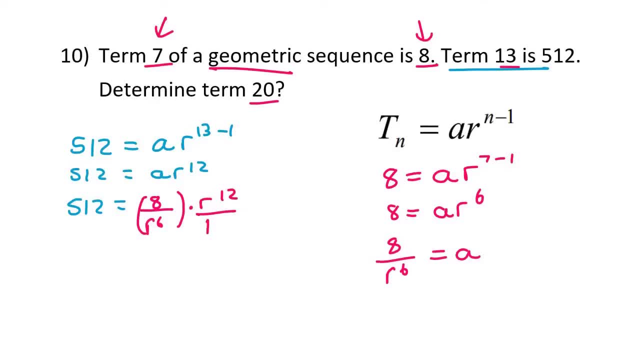 do now? Well, what I tell them to do is just pretend that this has a 1 over it. Now we don't really need these brackets. Now. what you're doing is you're just multiplying across, So it just becomes 512 equals to 8.. Sorry, I'm rewriting the same thing. It just becomes 512 equals to 8.. 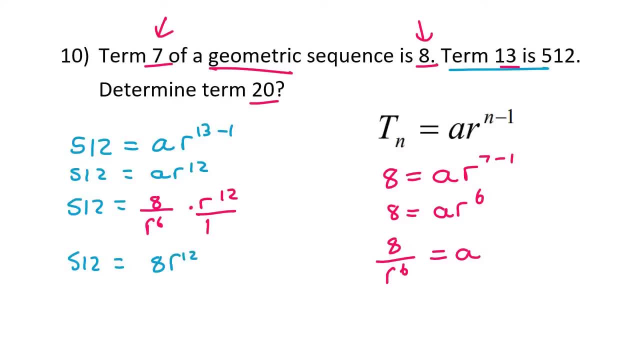 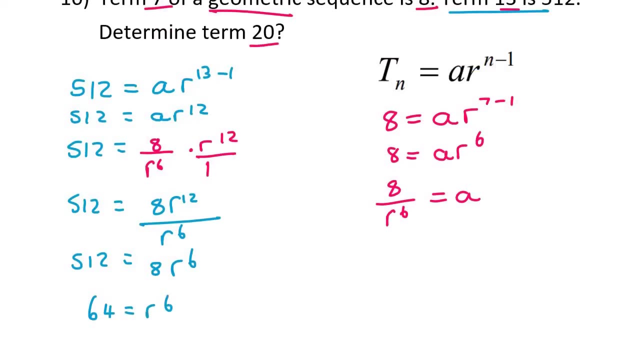 It just becomes 8r12 over r6. Now r12 over r6 just becomes r6. So we have 8r to the 6. Then we can divide by 8, which is 64. You then take the sixth root like this, And so: 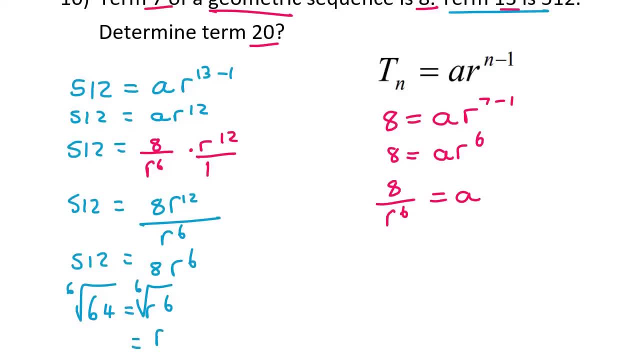 r would eventually equal 2.. Now we can get a by plugging that answer back into here. So a is going to be 8 over 2 to the power of 6. And that'll be 1 over 8.. Now the question says: 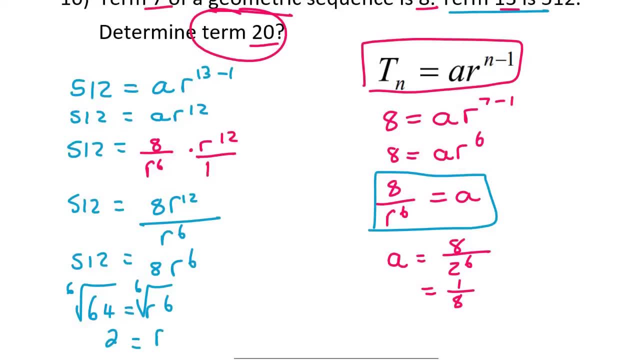 find term 20.. So we just use this formula And we say that term 20 is equal to a, which we've now found is 1 over 8.. r is 2. And n is 20.. Go ahead, type that in And we get an answer of 6.. 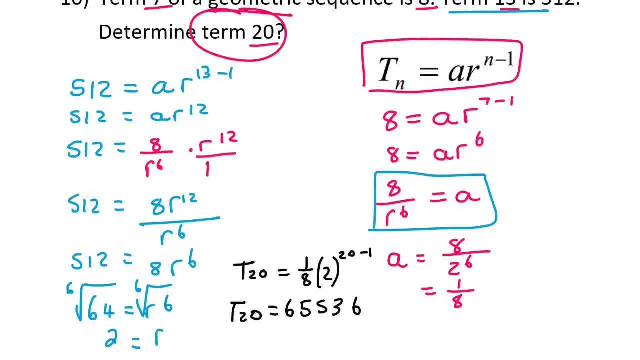 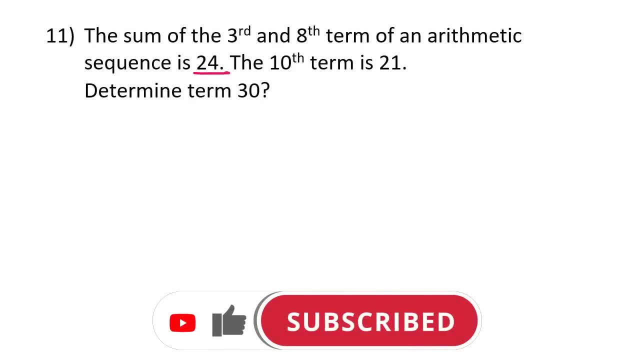 5,, 5,, 3, 6.. Question 11 says the sum of the third and eighth term of an arithmetic sequence is 24.. Now what often happens is students see the word sum and they instantly want to go for the sum. 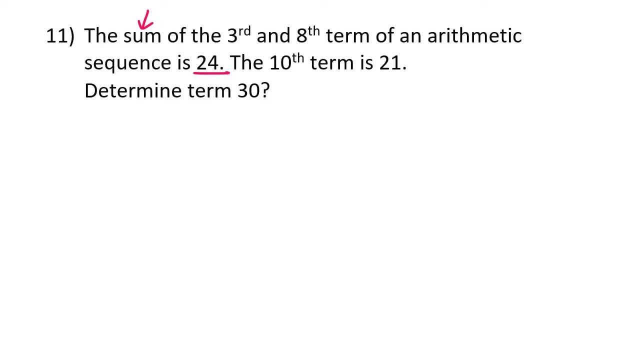 formula. But I'll show you why this is incorrect. If you had to use the sum formula for three terms, what that actually means is term 1 plus term 2 plus term 3.. They didn't say that The sum of all the first three terms. they're saying the sum of only the third term and only. 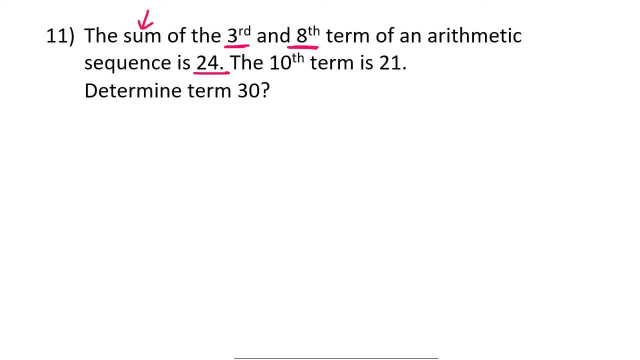 the eighth term. So what this actually means is that term 3 plus term 8 will be 24.. They also tell us that the 10th term is 21.. So we can say: t10 equals 21. So now all we do is we just fill. 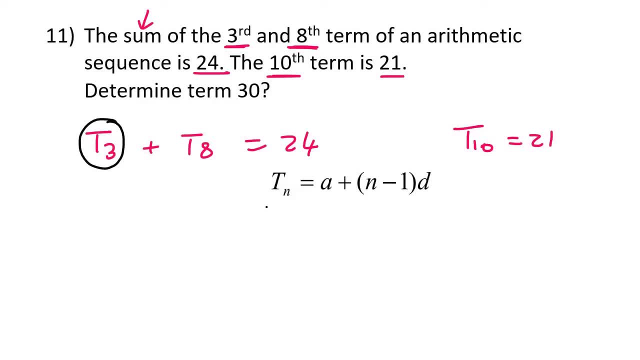 in as much as we can. So term 3,, if we use this formula, is the same as a plus. now n would be 3 because it's term 3, and then the common difference, we don't know. Then it says plus, that's this plus. Then term 8 would be a plus 8 minus 1 times d. 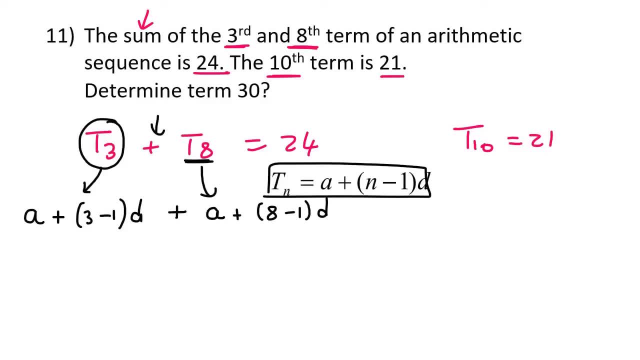 Can you see what I did there? I just used this formula on term 3 and then on term 8.. We then say that that is equal to 24.. I'm then going to use this piece, which tells us that 21 is equal to a plus. now it's term number 10.. So we say 10 minus 1. 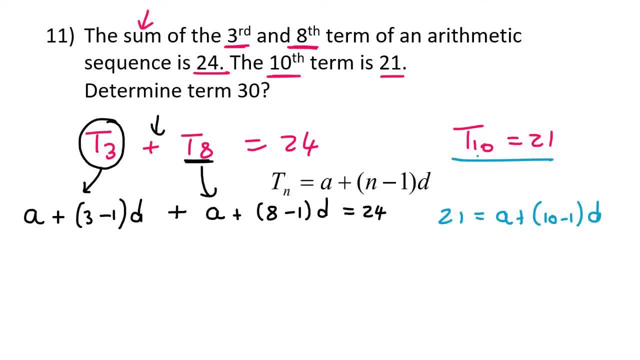 times d. Now we're just going to neaten up. So for this side it's going to be: a plus 2d plus a plus 70 equals 24.. I can neaten that up even more: 2a plus 9d equals to 24.. And then on this side, 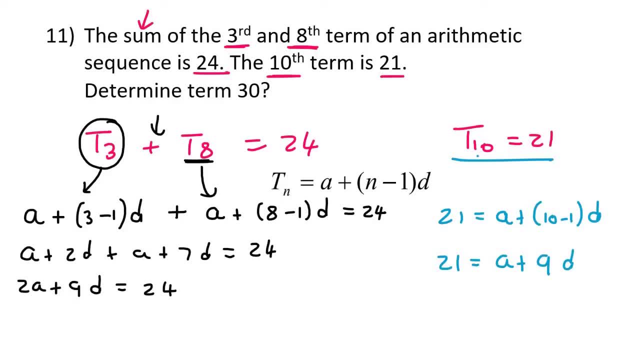 it will just be. 21 equals to a plus 9d. Now it's a simultaneous scenario, So you can do this however you want. What I'm going to do is I'm going to try to use this equation and I'm going to get a by itself. If I do that, it would be 21. 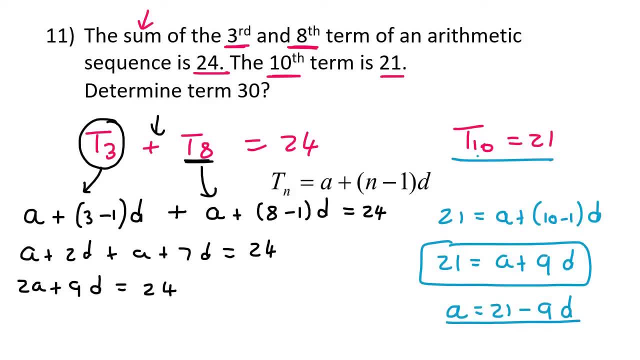 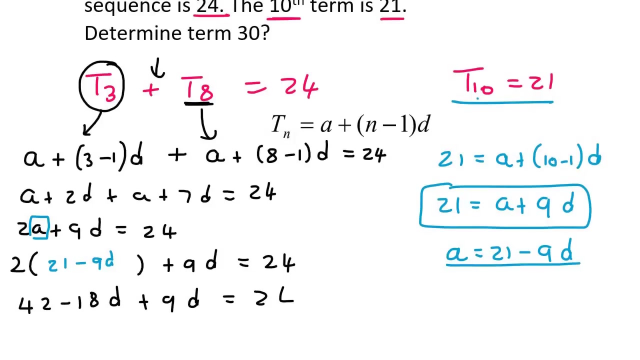 minus 9d. I'm then going to plug that expression over here, So it's going to be 2, and then in brackets we're going to put 21 minus 9d plus 9d equals 24.. And then multiply in. that will be 42 minus 18d plus 9d equals to 24.. You would eventually get. 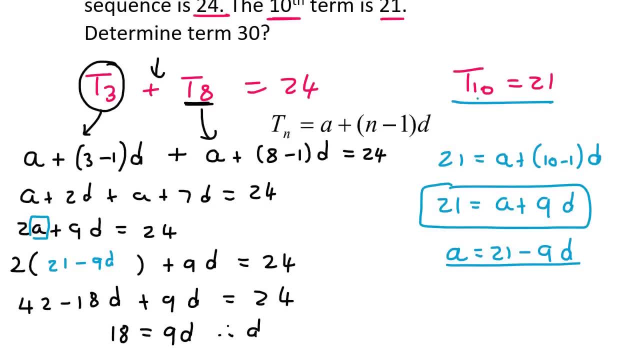 18 is equal to 9d. Therefore, if you divide, d is 2.. You could then plug that over here to find a and we'd see that a is 21 minus 9, and then we said d is 2.. 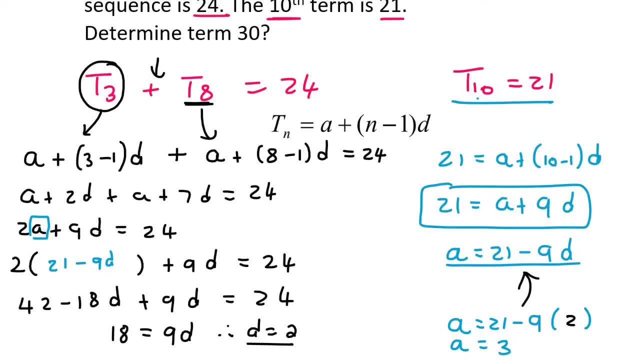 And so a would end up being 3.. The question then says: find term 30. So we can then go to our normal formula and find term 30,, because we now have a as 3, term 30, and then d is 2., And so we should. 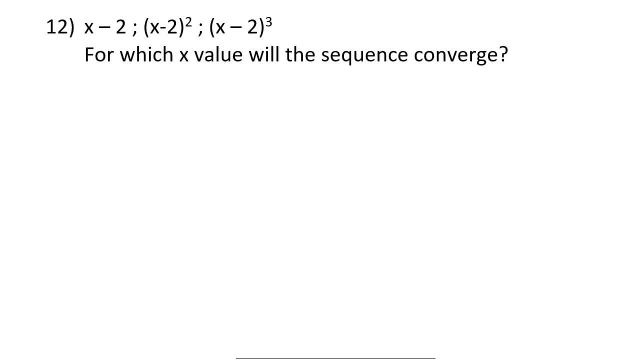 end up with 61 as our answer. In question 12, they ask us for which x value will the sequence converge? We should know that converging sequences are when the ratio is between minus 1 and 1.. So what you do is you find r. Now, if I gave you a normal geometric pattern like this to find r, you would 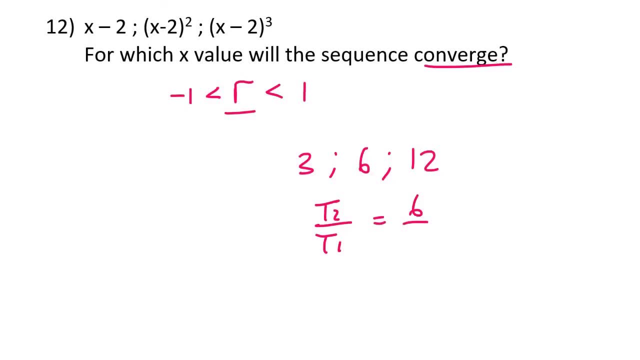 say term 2 over term 1, because that would be 6 divided by 3, which is 2.. Sometimes you can also see it, but if you don't, then you use this method. So I'm going to use the same approach here. I'm 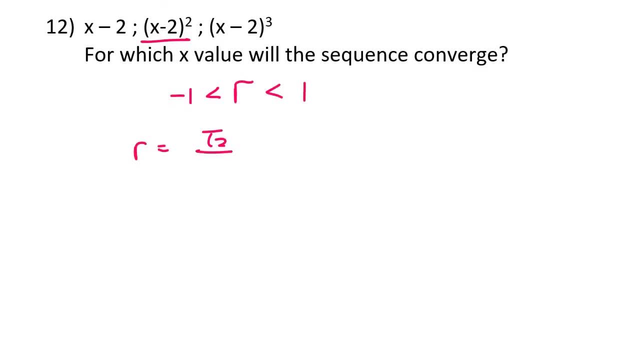 going to say t2.. I'm going to say r is equal to t2 over t1.. Now, term 2 is x minus 2 squared, and term 1 is x minus 2.. Now, depending on how comfortable you are with this type of maths, you might see this quite. 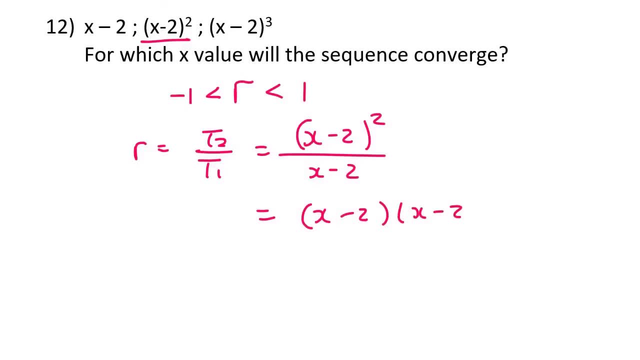 easily. But what I'm going to do is I'm going to write the x minus 2 out twice, because that's what this 2 means, And then you can cancel one of them, And so r is x minus 2.. What I then do is I take 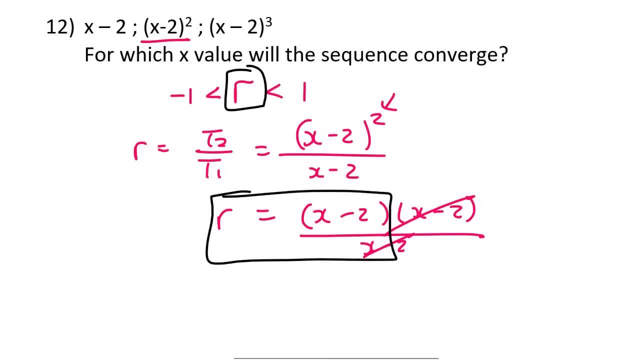 this r, which is x minus 2.. I replace it over here, So I say x minus 2 is smaller than 1 and bigger than negative 1.. I then solve by taking this minus 2 there and I also take it over to the left, And so there is our. 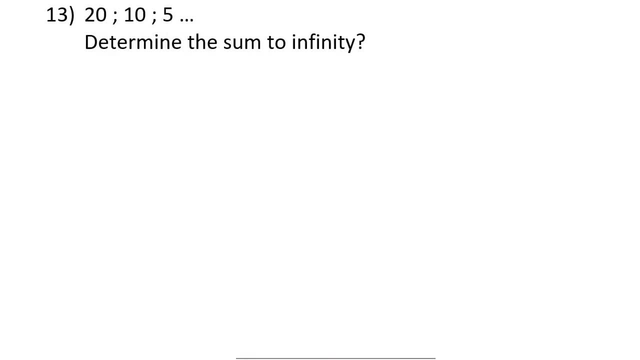 answer With number 13,. they've asked us to determine the sum to infinity, So we use the sum to infinity formula. And so to use the sum to infinity formula, we need a, which is term 1, and then we need r, which is the ratio. Some students tell me that the ratio for this is 2,. 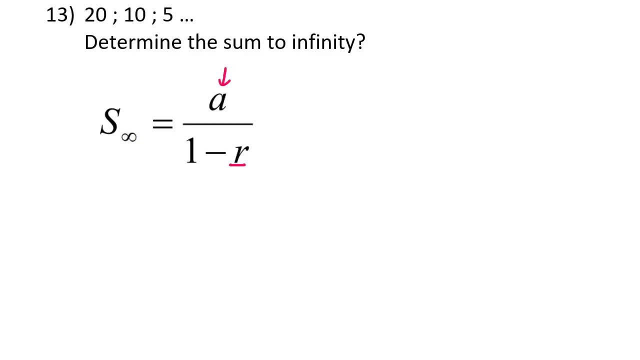 which is 1.. I understand what they're saying. It's because we're dividing by 2.. But remember that your ratio is how much are you multiplying by? So your ratio is actually going to be a half. But if you struggle with that, remember that to find your ratio you can say term 2 over term 1.. 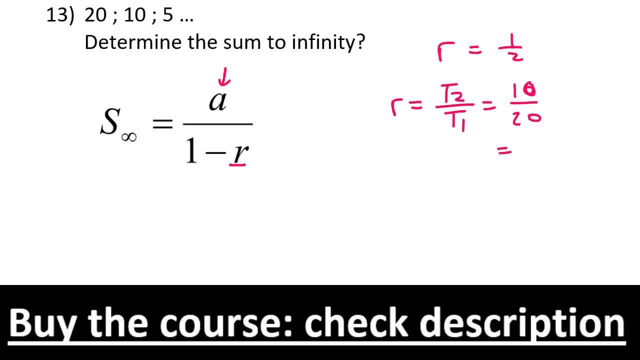 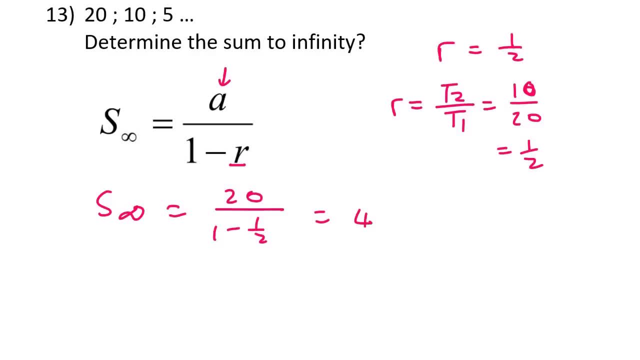 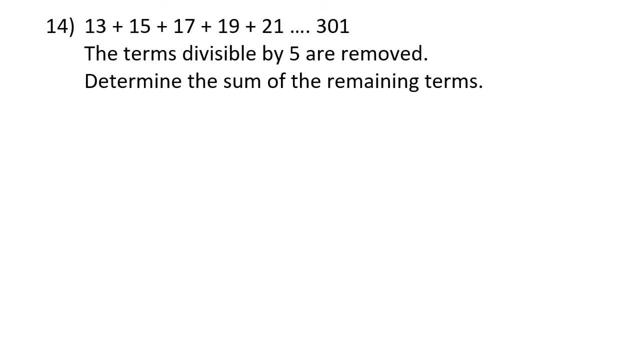 So that'll be 10 divided by 20, and that's going to be a half. So then what we do is we go full everything in and that'll give us 40.. Question 14 does confuse students, but if you just stick around and see how we do it, 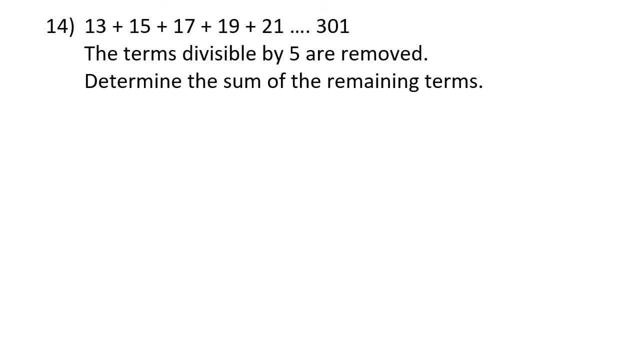 there is a method to how to do a question like this And once you understand it, it's very easy. So they're saying that all the terms that are divisible by 5 are going to be removed determine the sum of the remaining terms. So pretty much, we've got this long sequence over. 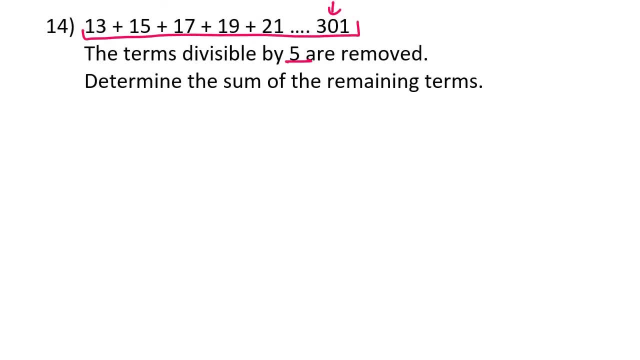 here that goes all the way up to 301.. And they want to know what is the sum of all the remaining terms once you remove the divisible by 5s. So my approach is to do the following. I completely ignore this part. What I do is I work out the sum of the sequence first. 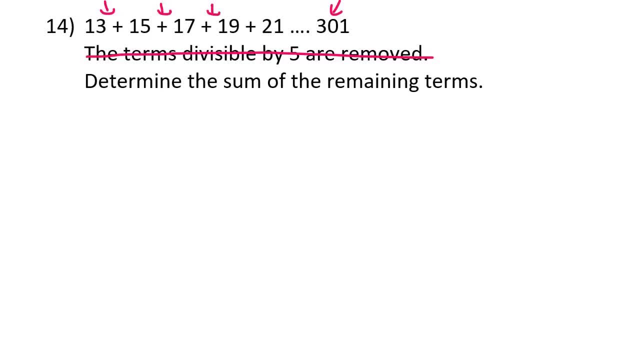 So we can see that it's arithmetic, because you're plussing 2 each time. So we can use the sum formula of an arithmetic pattern. The issue is is that we don't know the number of terms. So what we do, we have a little trick: We know that the last 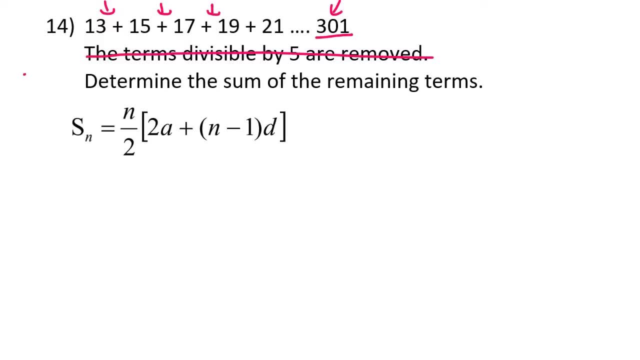 term is 301. So we use the TN formula, And then what we do is: we know that the last term is 301. So we say 301 equals to A, which is 13, plus N- we don't know- And then D is the difference of 2.. 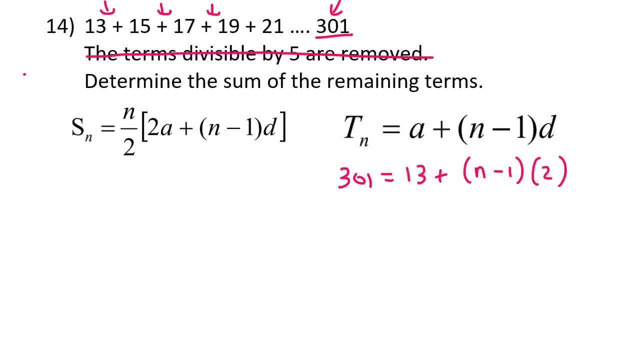 Now we can just go ahead and solve this. I'm going to move the 13 over to the left, which gives me 288, equals to N minus 1 times 2.. You can multiply the 2 into the bracket. I like to rather divide it on the left. So we end up with 144 equals to N minus 1,. 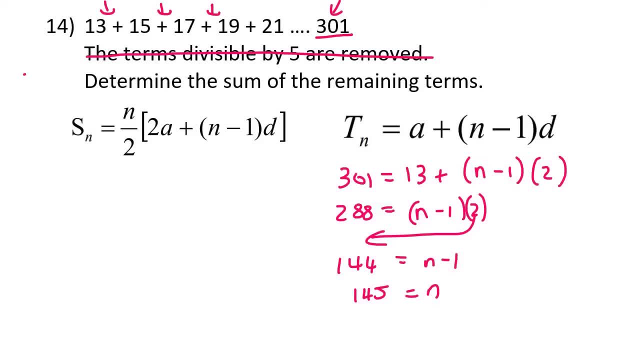 solve for N and we get 145.. So what that technically means is that 301 is at position 145. But because it's the last term, that also shows us how many terms we have. So in this original sequence we have 145 terms. 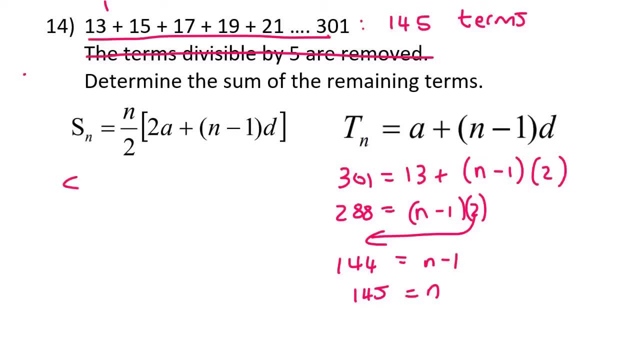 So we can go work out the sum of all of those numbers now by saying: sum of 145 terms equals to 145 over 2, 2 times. now A is 13,, 145 minus 1, and our common difference is 2.. And so we end up with: 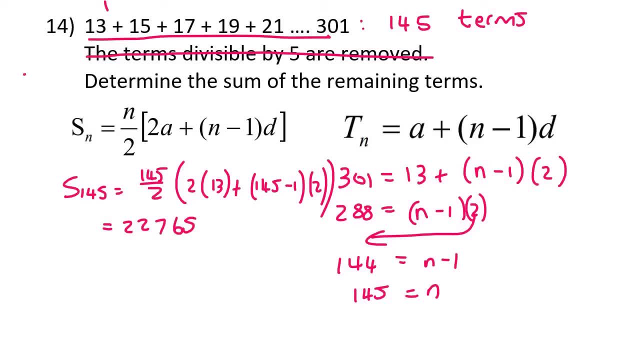 22,765.. So that's what the sum will be if you add up all of these numbers: 22,765.. All right, so now we're going to move on to the next part of the question, which is to look at the. 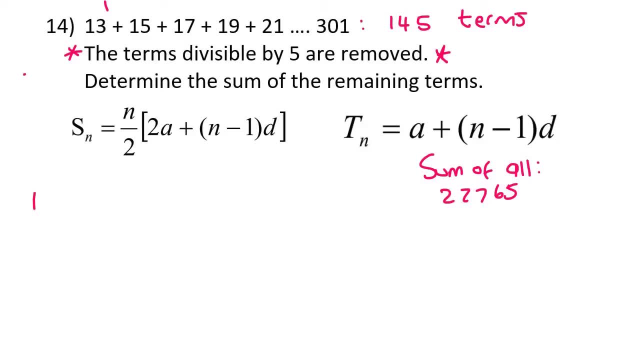 terms that are divisible by 5.. So let's go find them. I'm going to write out the first couple of terms And I recommend you find the first three terms that are divisible by 5. And let's see if they make a pattern. And sometimes it does actually take quite long until you find the first three. 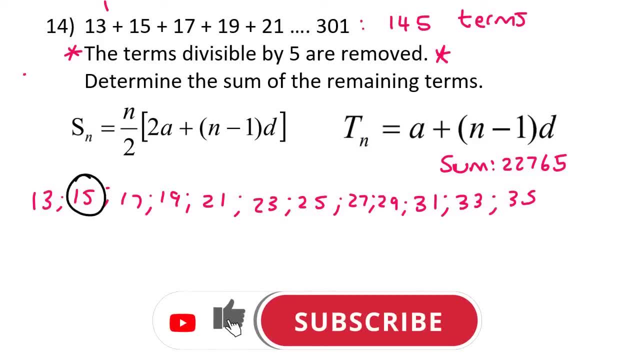 But here they are. The number 15 is divisible by 5,, 25, and the number 35. Guess what? Those numbers form their own pattern, And it always will work out like this: 15, 25, 35. Look at that, It's its own little pattern. So what we need to do now? 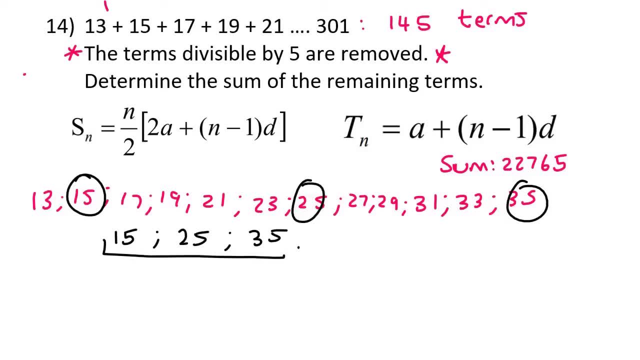 is, try to work out the sum of this pattern. The problem is, we don't know where it stops. However, we do know that in the original sequence the last term is 301.. So we can't go past that. So then Kevin does that. 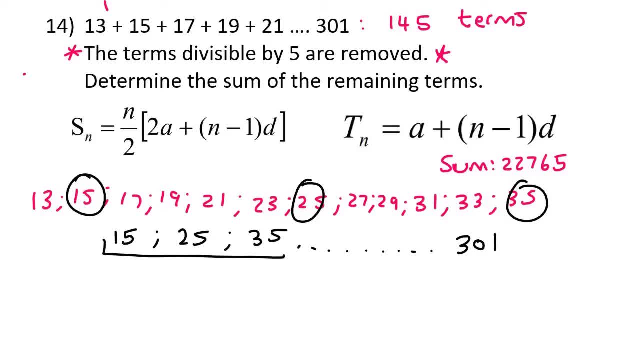 Does this mean that our last term on this one should be 301?? Well, no, because that's not divisible by 5.. But what we can do is we can try imagine what the last term would be in this sequence that is divisible by 5.. So we can work backwards. This would be 299,, 297, and 295.. That. 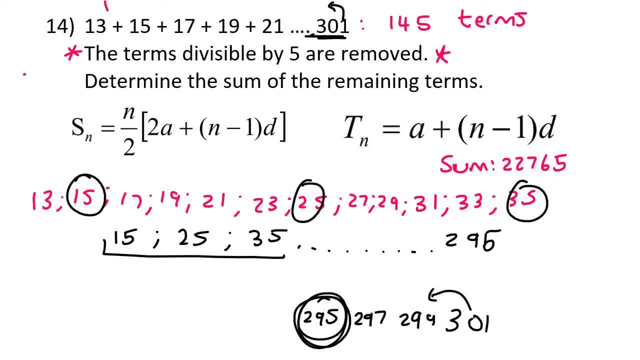 is divisible by 5.. So that'll be the last term in this pattern. So now our goal is to find the sum of all of these terms. So we're going to do that, So we're going to do that, So we're going to do. 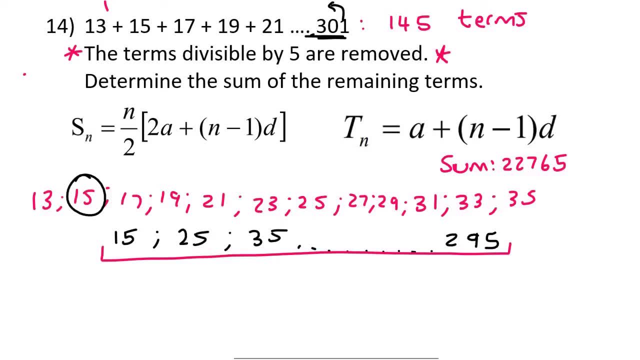 these terms Once again. we don't know how many terms there are, but we can use our TN formula to work out the term number of 295.. So we're using this formula over here once again And we can say: 295 equals to A, which is 15, plus now N, we don't know. Now the common difference is not 2,. 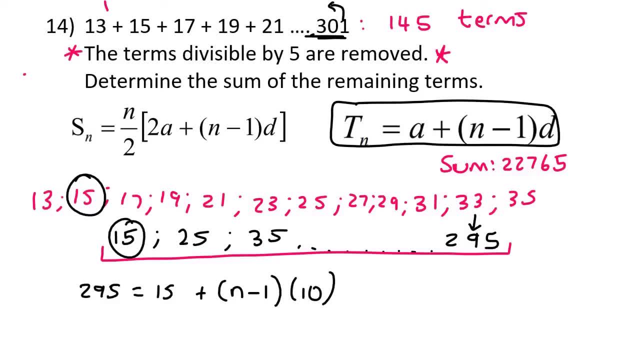 because we're busy with a new sequence now. So that's going to be 10.. Now we just move stuff over. I'm then going to divide by 10, which gives me 28.. Now I move the minus 1 over. So that means 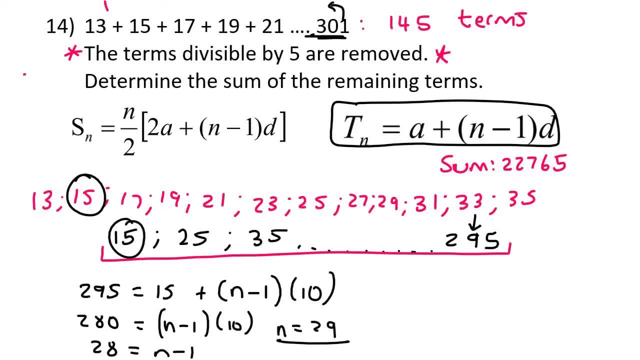 29.. So we have 29 terms in our divisible by 5 sequence. So now what we can do is use this formula to work out the sum of those 29 terms, which would be 29 over 2, 2 times Now A for that. 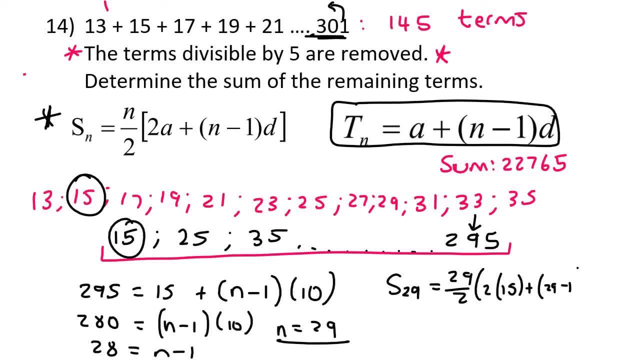 sequence is 15, 29 minus 1.. And then the common difference in that sequence is 10.. And that gives us 4,495.. All right, guys. So here's where it all comes together. When we added up all of these terms, we got 22,765.. We then looked at all the numbers that 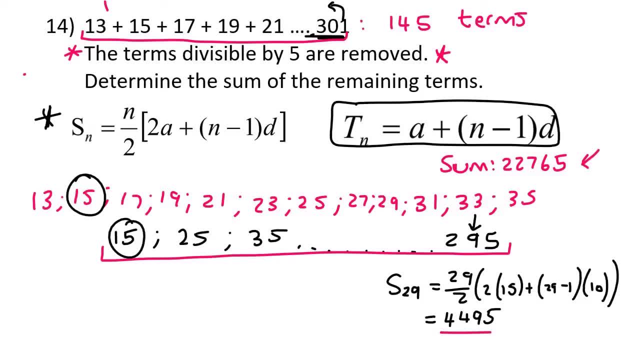 are divisible by 5, added them together and got 4,495.. So the question says: determine the sum of the remaining terms. if you take away the divisible by 5s You would end up with. I'm going to say sum of remaining would obviously be the total. 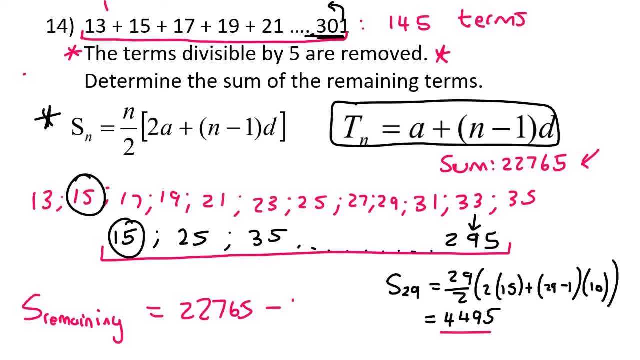 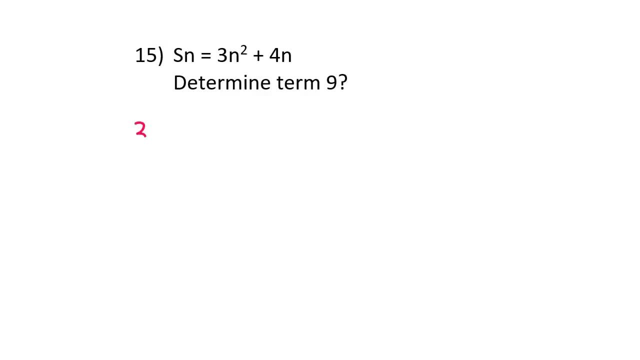 minus the divisible by 5 sum And that'll give us a value of 18,270.. This is quite an interesting question. I'm going to show you something quite interesting. Let's say we have the sequence 3,, 5,, 7, and 9.. 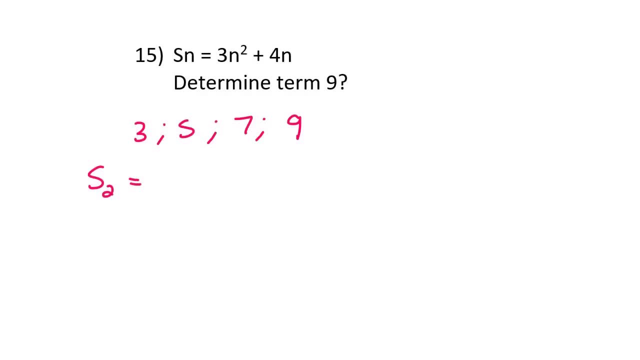 What would the sum of the first two terms be? Well, that would be 8.. And what would the sum of the first three terms be? Well, that would be 3 plus 5,, which is 8,, plus 7,, which is 15.. 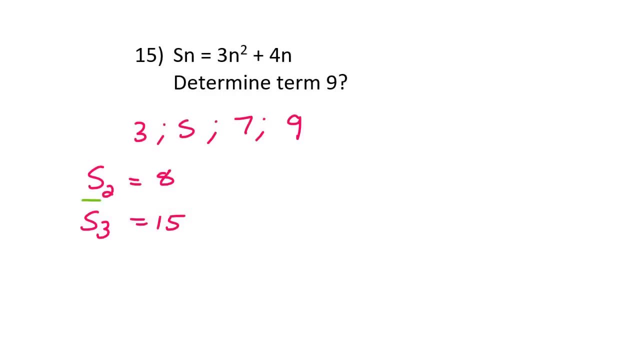 So think about this carefully. If you add up the first two terms, you get 8.. So I'm going to say a T1 plus T2 is 8.. If you add up the first three terms, you get 15.. Would you agree with me that that means term 3 would have to equal 7?? 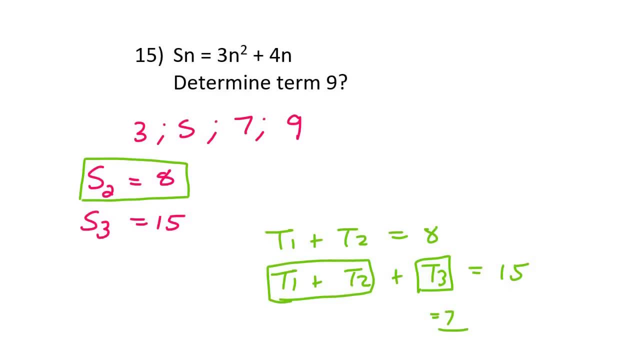 Because if the first two terms are already equal to 8, then the third term must be 7.. And we can see that it is. So there is a general property. If you want to find a specific term number- let's say you want to find term 8, then you sum up the first eight terms and then you minus the. 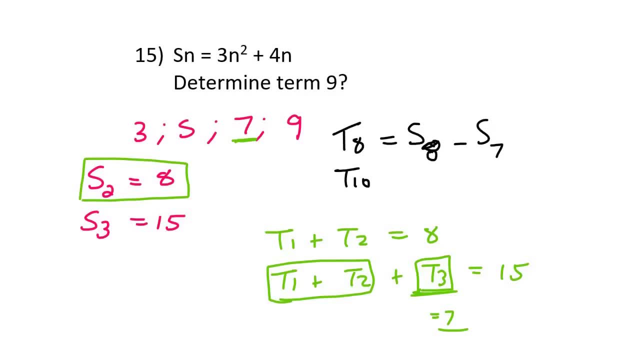 sum of the first seven terms. If you want to find term 10, you sum up the first 10 terms and you minus the sum of the first nine terms. So we want to find term 9.. So what you do is you say term 9 is the same as the sum. 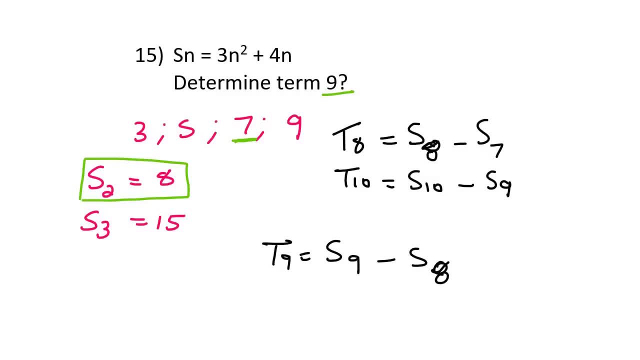 of the first nine terms minus the sum of the first eight terms. So let's find the sum of the first nine terms. Well, they've given us the formula for Sn, so you literally just plug it in. So it's going to be 3 times 9 plus 4 times 9.. 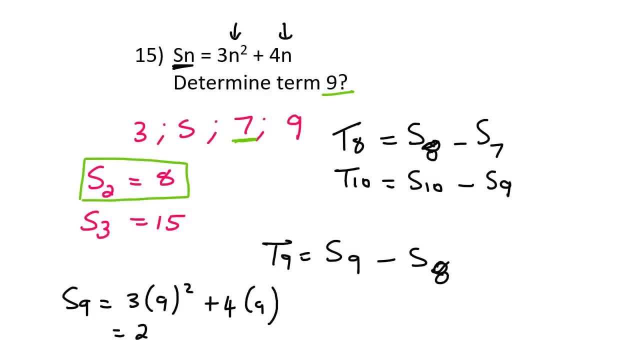 And that would be 279.. Now we can find the sum of the first eight terms. Why do I keep wanting to write that as an infinity symbol? It's really weird. Can't write an eight anymore. Oh, there we go. Sum of eight terms. Well, you would just say 3 times 8, squared plus 4 times 8. And that's 224.. 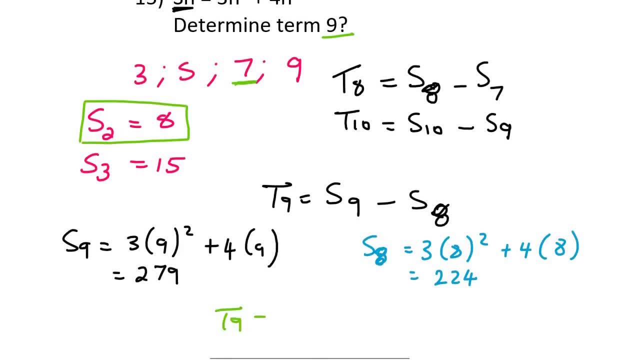 So we now say that term 9 will be the same as the sum of the first nine terms minus the sum of the first nine terms, minus the sum of the first eight terms minus the sum of the first nine terms, And that's 55.. Let me explain this quickly. What does S8 stand for? S8 means what is the sum of the first. 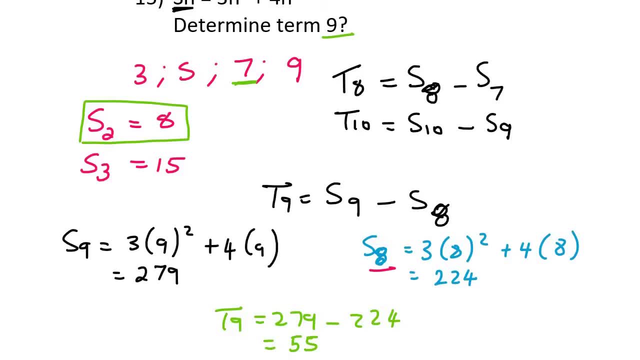 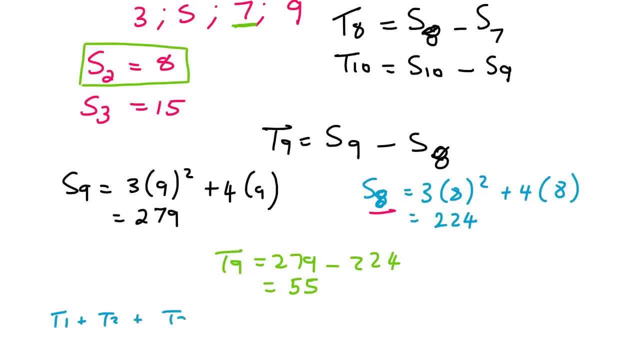 eight terms. So if you add up all eight terms, I'll actually show you. If you add up all eight terms, T1 plus T2 plus T3 plus T4 plus T5 plus T6 plus T7 plus T8 plus T9 plus T10 plus T11 plus T12. 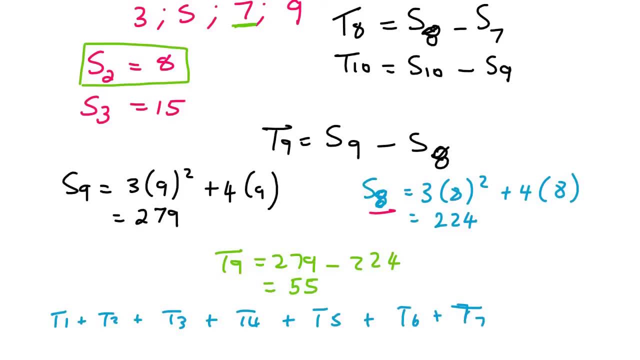 plus T12 plus T13 plus T14 plus T15 plus T16 plus T17 plus T18 plus T19 plus T20 plus T21 plus T21 plus T22 plus T23 plus T23 plus T24.. If you sum up the first nine terms, let's see what that would. 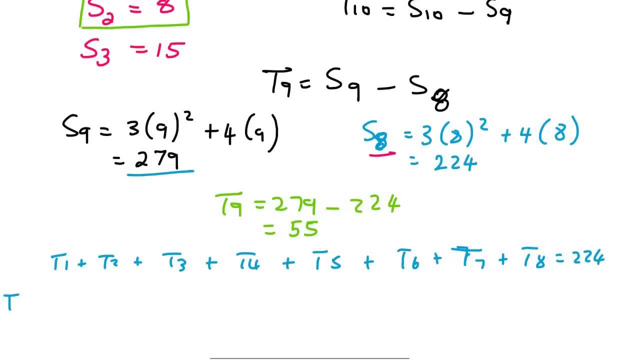 look like. So that would be T1 plus T2.. Well, that gives us 279.. But, guys, what we can see is that the sum- well, let's do here the sum of this first eight terms- is already 224.. So it's almost like 224 plus term nine must give us 279.. So then to find term nine, 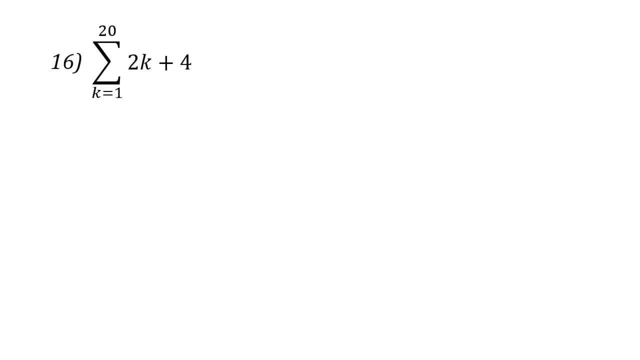 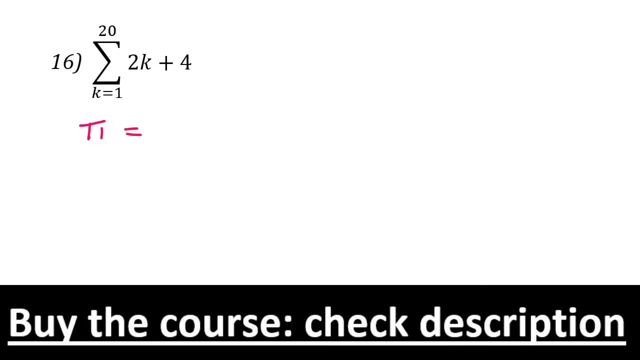 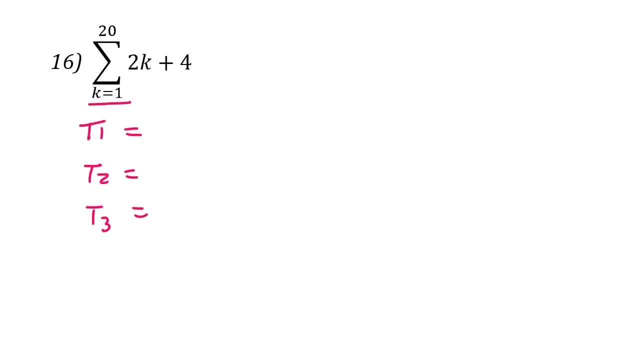 you would just minus them And that's how we got 55.. Question 16 has to do with sigma notation. So what you do with sigma notation is you find the first three terms, term one, term two and term three. How do we do that? Well, you plug whatever this number is into there to find term. 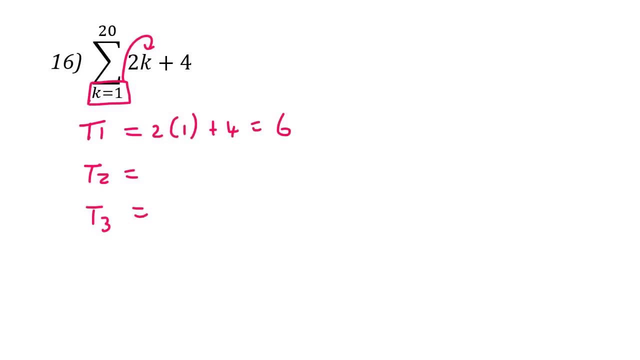 one. So it'll be two times one plus four, which is six. Then you let this number go up by one, And that'll be for term two. So it'll be two times two plus four, which is eight. And then you do the last. 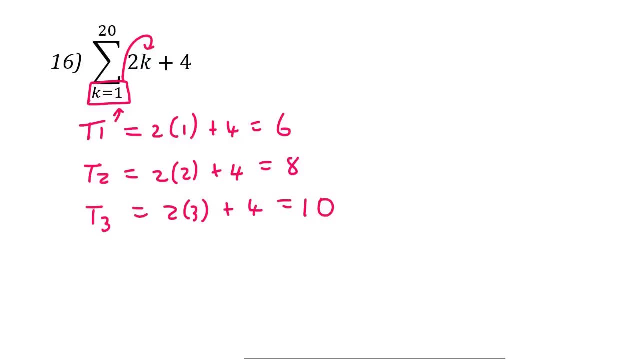 one. So what I want you to realize is that this number will not always be the same as this number. Okay, so term one isn't always going to have a one there, Term two isn't always going to have a two there And term three isn't going to have a three there, Because sometimes, 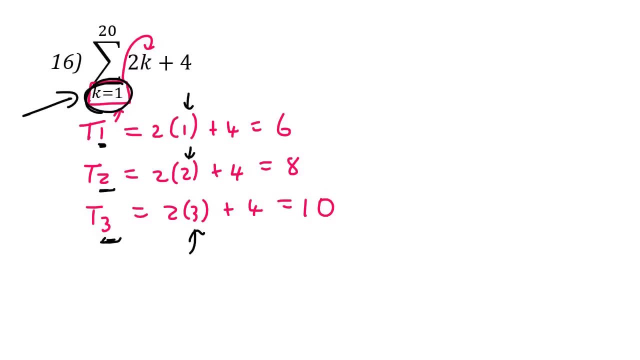 this number at the bottom is not a one, And we'll look at examples like that just now. Now, Kevin, why did you say the first three terms? Because if you do the first three terms, you will be able to see what kind of pattern you have. You have six, eight and 10.. That is. 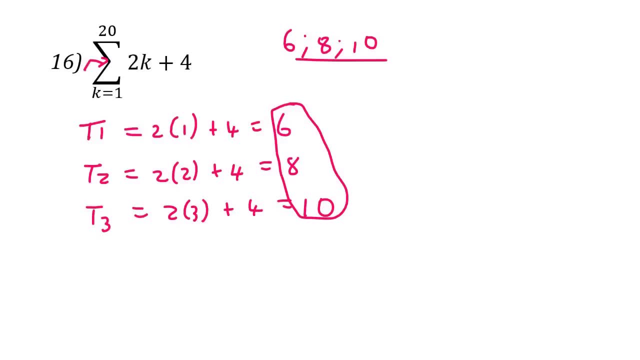 arithmetic. Now, did you know that this symbol, sigma, actually stands for the sum? So it's actually saying: find the sum of all the terms. Kevin, how many terms are there To find the number of terms? please don't just always look at that number, Because once again, when they change this number, 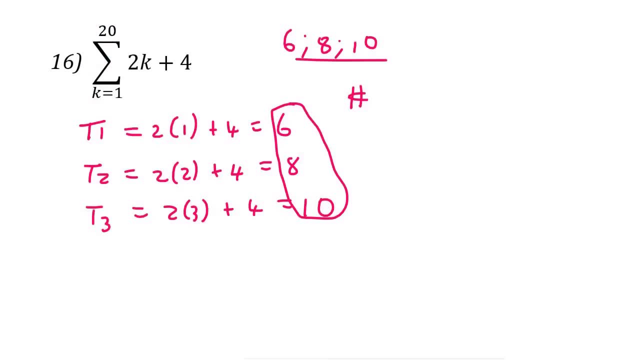 at the bottom, then all of that changes. So what you do instead is you take the top number minus the bottom number, and then you plus one. So the top number is 20.. The bottom number is one, and then you plus one, and that gives you 20.. So, yes, it is a 20 now, But that's just because. 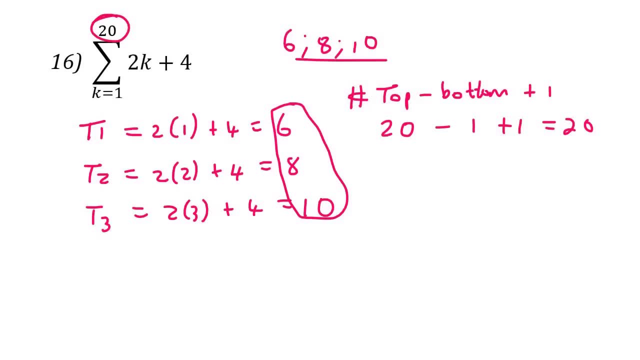 the number at the bottom is a one, So just look out for that. All right, so we have 20 terms, We have an arithmetic pattern, And so we can use the sum formula for an arithmetic sequence, And so we're finding the sum of 20 terms. So we say 20. 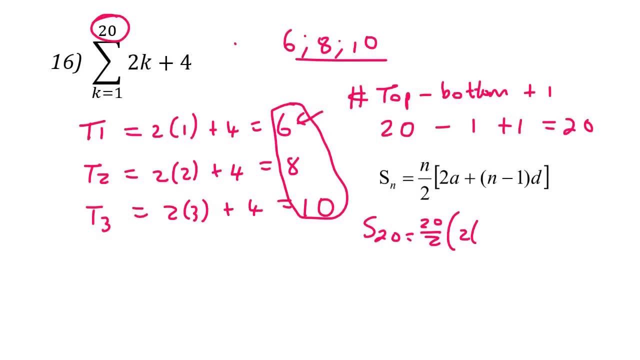 over two. A is term one which we found as six, And then 20 minus one, And now the common difference: we're plussing two each time, So you can just say two. Oh, it gives us quite a nice. 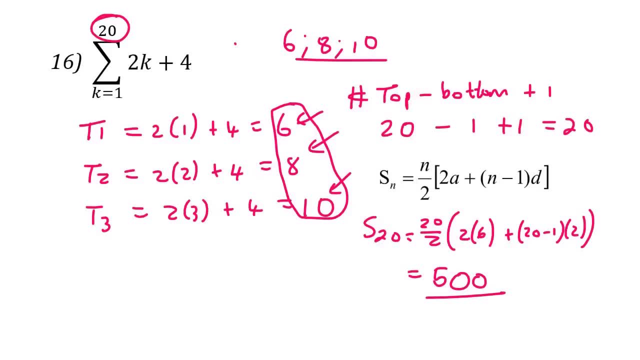 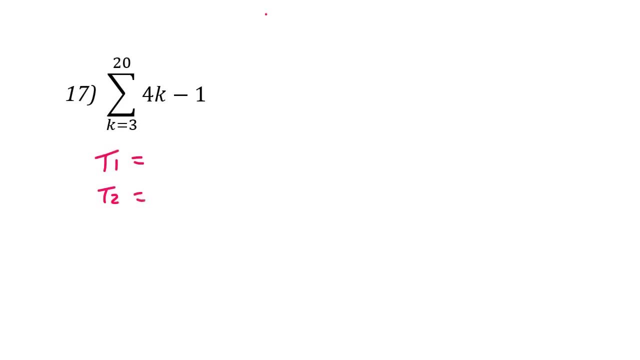 number 500 is the final answer, And then we're going to do another sigma notation. So remember: step one is just find the first three terms. People are always like Kevin. does this mean term three? Not at all. To find term one. 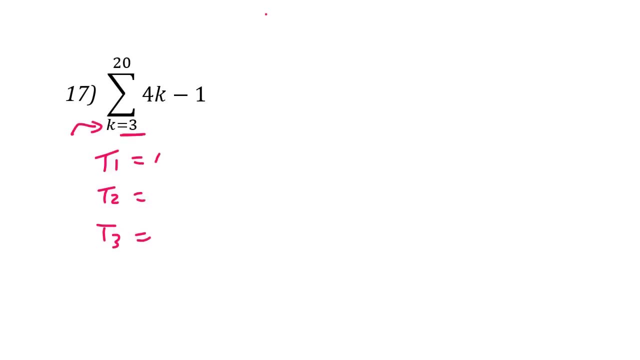 you are simply going to start with whatever number you have here, So it'll be four times three minus one, which is 11.. Then you just increase by one each time, And that'll be 15.. And then four times five minus one, and that'll be 19.. 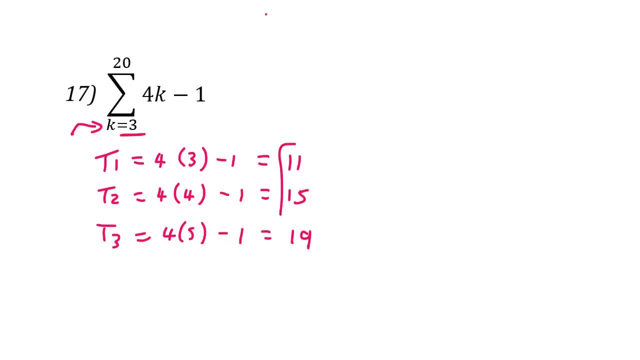 Here we have the first three terms. From that we can see that it is arithmetic. So we can use the sum two formula for an arithmetic pattern. But you've got to be careful. This 20 is not the number of terms. Remember, in the previous question we said that to work out the number of 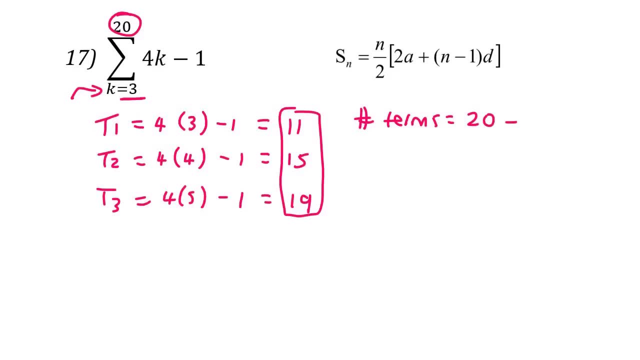 terms. it's the top number minus the bottom number, which in this case is a three, and then plus one. That'll give us 18.. So there are only 18 terms, not 20.. Why am I writing my eights as an infinity sign? So we're going to say 18 over two, Then A is term. 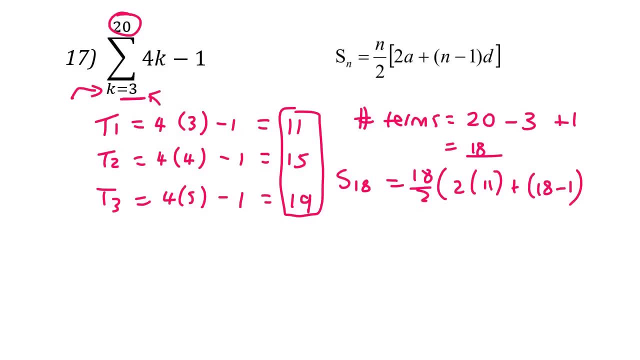 one which is 11.. N is 18.. We don't use that 20 at all in the calculation. And then D, which is the difference is. you can see we're plussing four, So that'll be your common difference. 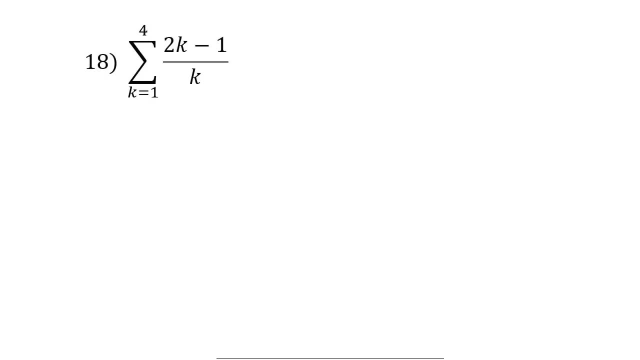 So that's going to be 810.. Question 18 is very interesting, But I'll explain the interesting part just now. You might have seen it If you tried this one by yourself. So let's go find the first three terms. So term one: 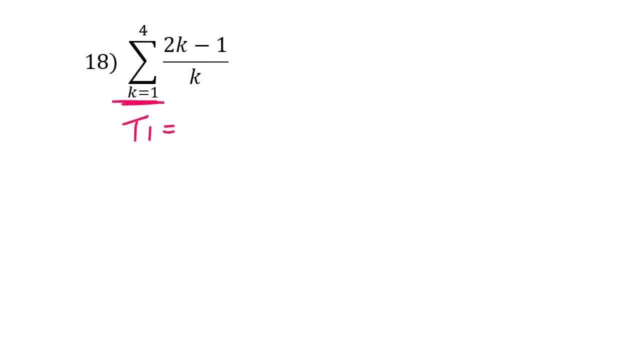 we know that you start by plugging whatever this number is into the place of K, So that'll be two times one minus one over one, And that actually just gives us one. Term two is going to be two times two minus one over two, which is three over two. And then, lastly, term three. 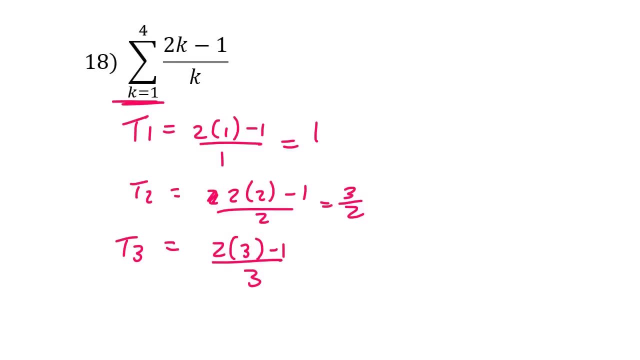 which will be two times three minus one Over three, And that gives us five thirds. Now here's why this question is very interesting. It is not arithmetic, but it is also not geometric To test. if it's arithmetic. I would test to see if T2 minus T1 is the same as T3 minus T2.. Let's see if it is the same. So if I 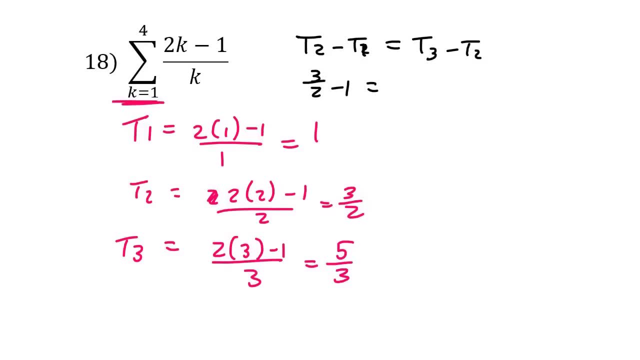 say three over two minus one, that gives us one, One half minus one, which is a half. Is that the same as T3 minus T2, which is five thirds minus three over two? So let's see what that gives. It gives us one over six. So these two are not the 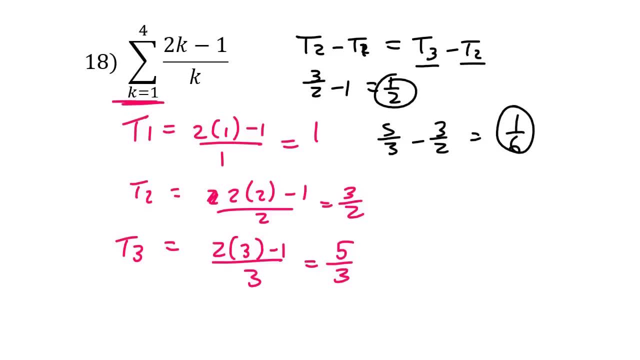 same, So it's not arithmetic. Then let's check if it's geometric. For it to be geometric, the ratios should stay constant, like that. So let's see if it does. So if we say term three, which is five thirds, if you divide that by two, that gives us one over six. So let's see if it's. 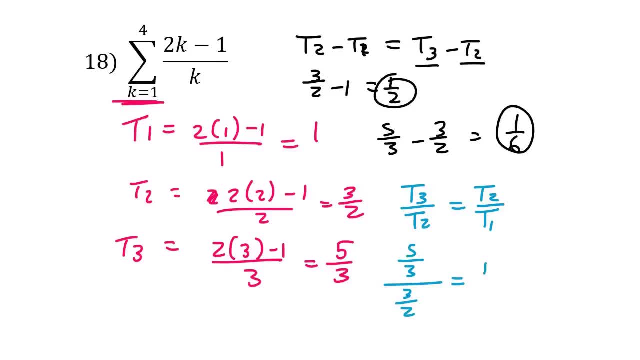 term two, which is three over two. Let's see how much that gives. So that gives us 10 over nine. Now let's check T2 divided by T1.. So T2 over T1 would be three over two divided by one. 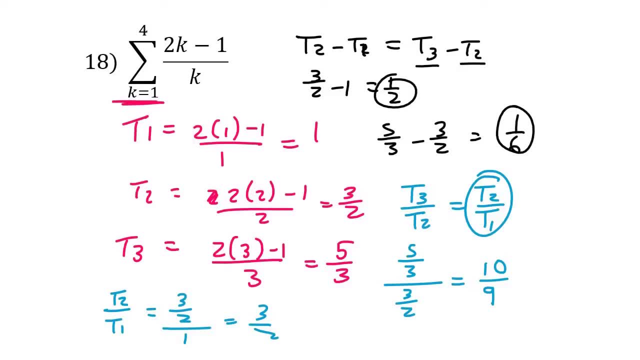 which is three over two. So the ratio is not even constant. So, Kevin, what is going on? We're in grade 12. We're learning about arithmetic and geometric patterns, And here you've thrown us a question that doesn't have any of them. So, guys, when you get a question like this in the exam, 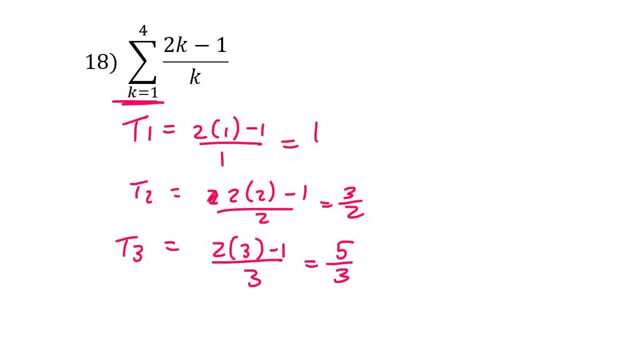 you've got to be careful. It's not arithmetic or geometric, It's not even quadratic. It doesn't matter, though, because what does the symbol stand for? again, It means the sum of, So you have to plus everything together. They haven't given you a lot of terms. Remember to work out the 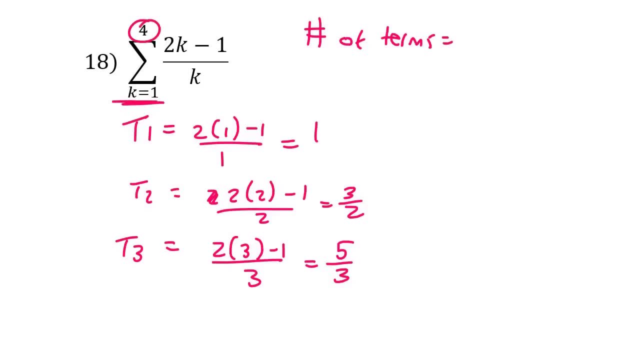 number of terms. You take the number at the top minus the number at the bottom, and then you plus one. In this case it means there are four terms, but it won't always be the same as this number, So be careful. 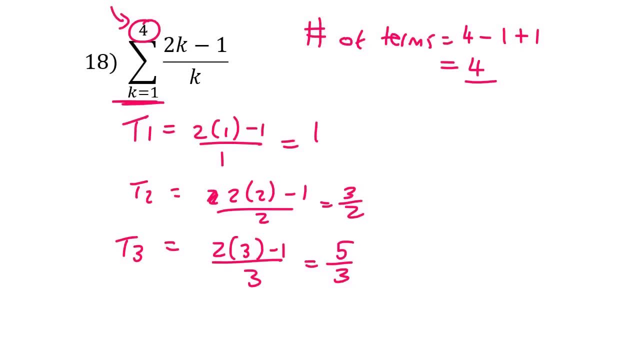 So we only have four terms. So let's just go find the fourth one by plugging in everything that we need to over here, And that gives us seven over four. Now what we do is we just go add these numbers together, because that would give us the sum And our answer is 71 over 12.. And if it wasn't? 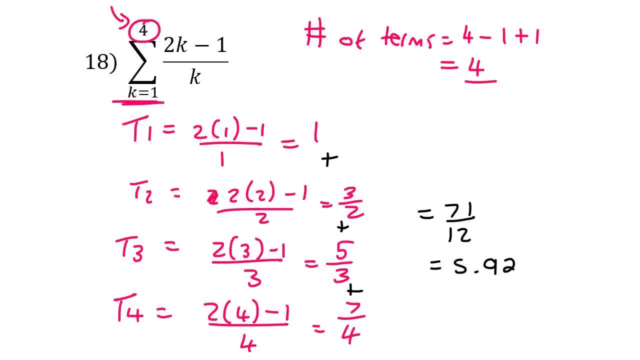 an exam where you would have two decimal places, you would say 5.92.. Now, Kevin, why didn't we just do this in the previous examples? You could, but in the previous examples they gave us like 20 terms, So it would take a lot longer. 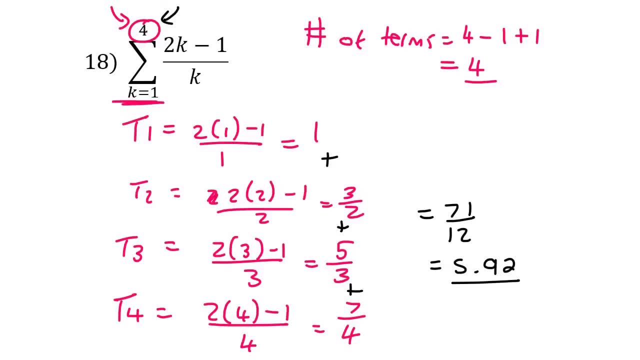 So that's in those types of examples it will always be arithmetic or geometric, And so you can just use the formula. But when they give you something like this that doesn't have any pattern, it'll usually be a very small amount of terms, And so you can do it manually on your calculator. 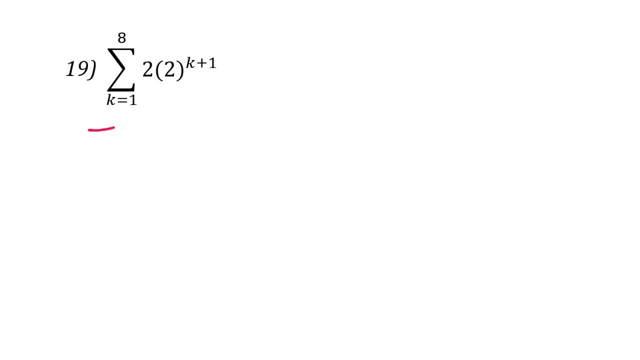 Question 19.. Remember with sigma notation questions, the first three terms. that helps us to work out what pattern we have. So for term one you start with whatever this number is In this example it is a one, but it doesn't always have. 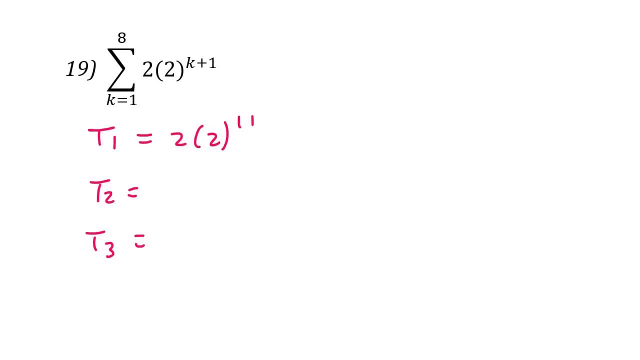 to be a one. So we can say two times two, and then one plus one, And that would give us eight. Then we just keep the process going on. So now it'll be a two plus a one, And that's 16.. 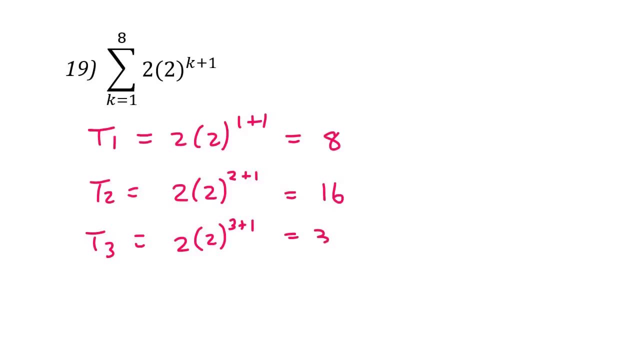 And then the last one, that'll be 32.. So you can see that this is geometric. They are multiplying by two each time, So we could go up to term eight if you wanted to, and then you would add everything together, like we had to do in. 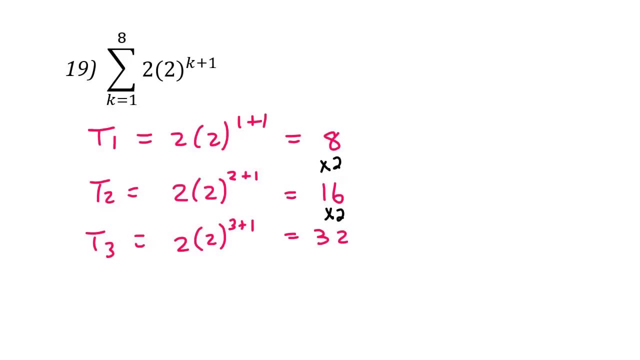 question 18.. However, we can do this in a much better way. We know that the sigma notation symbol stands for finding the sum, So we just use the sum formula of a geometric pattern, And so we finding. well, we need to see how many terms we have. 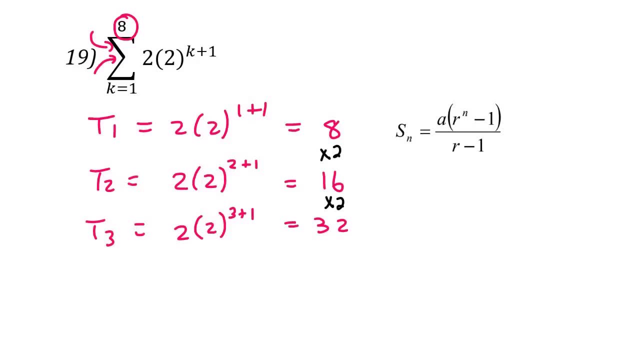 now remember it's not always going to be the same as this number at the top, But it is if this number is a one. But remember, the proper way to work out the number of terms is to go top number minus the bottom number and then always add one. So that's going to be eight. 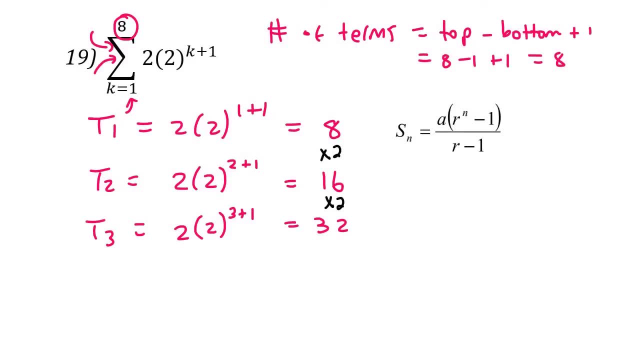 minus one plus one. So in this example there will be eight terms. So to find the sum of eight terms we go a: a is always your term one, which is eight, The ratio we are multiplying by two, then to the power of eight, and then over two minus one, And that gives 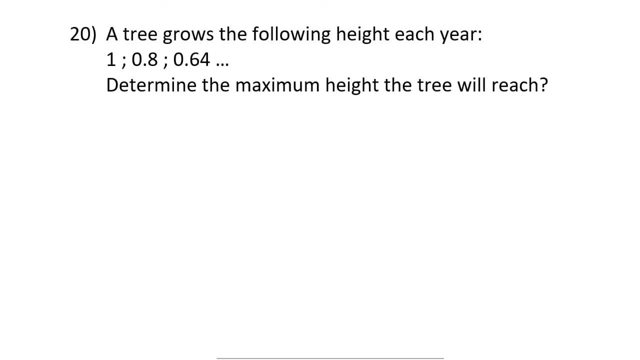 us 2040.. Number 20 is quite a good question In exams. they love to test students on this kind of concept. So they tell us that we have a tree that is going to be growing. Okay, now, in the first year the tree grows one meter. All right, let's draw it out. It's one meter. Then in the 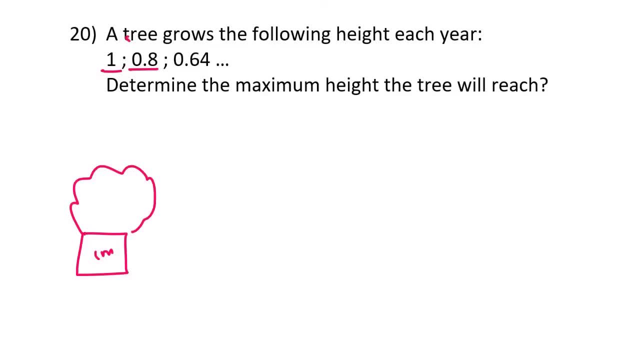 second year it grows one meter. And then in the second year it grows one meter And then in the third year it grows by 0.8.. So it would be 1.8 meters tall. Then in the third year it grows 0.64.. 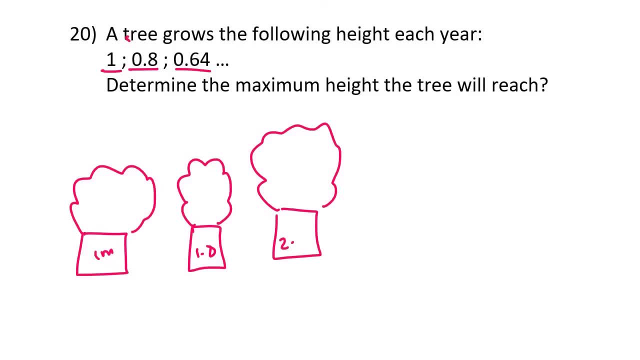 So now it would be 2,64 meters. It says now what says that we need to determine the maximum height that the tree will reach. But, guys, we don't know how long the tree is going to be growing for. Is it 10 years, 100 years, 2000 years? 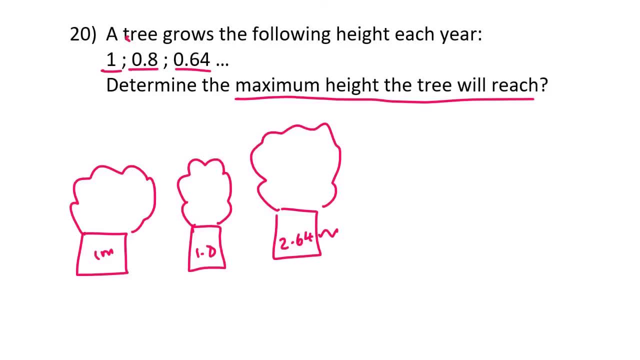 Guess what? It doesn't matter, Because what we should realize is that this is a geometric pattern And the numbers are getting smaller. This means that they will eventually approach zero. That is a converging geometric pattern, So all we need to do is use the sum to infinity. 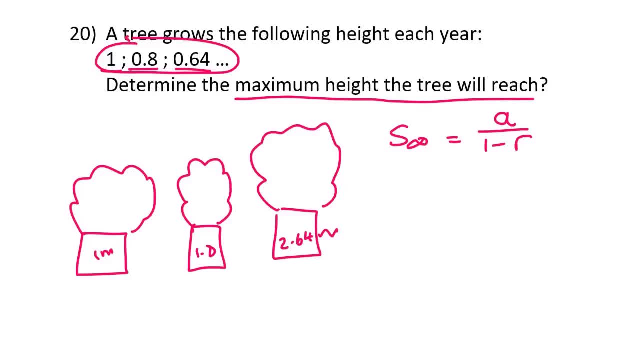 formula which is a over one minus r. So which numbers do we use? Well, if we add these numbers together, that will not make sense, Because if you say one plus 1.8, then are you telling me that the tree is 2.8 meters tall after year two? No, these numbers. 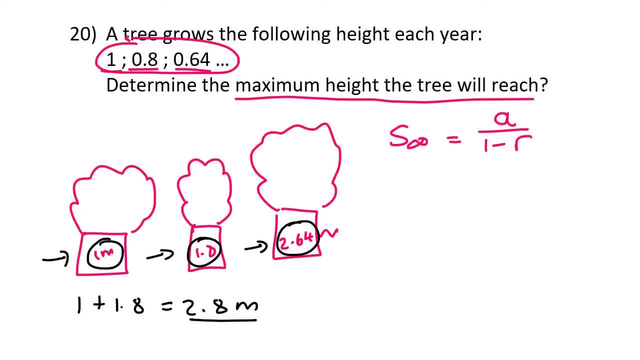 are showing us the height of the tree, the total height of the tree, So you want to ignore those numbers. I just did that so I could explain this part. What you want to do is you want to take how much the tree grows by every single year, And you want to take the total height of the tree And you 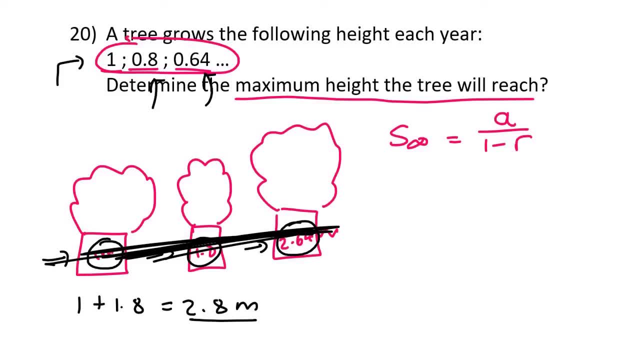 want to add those numbers together, Because if you add the amount of growth, that will give you the total height of the tree. So we need to work out r? r. you can work out as t2 over t1,, which is going to be 0.8, over 1, which is 0.8.. Let's just make sure that the ratio stays constant, So we can. 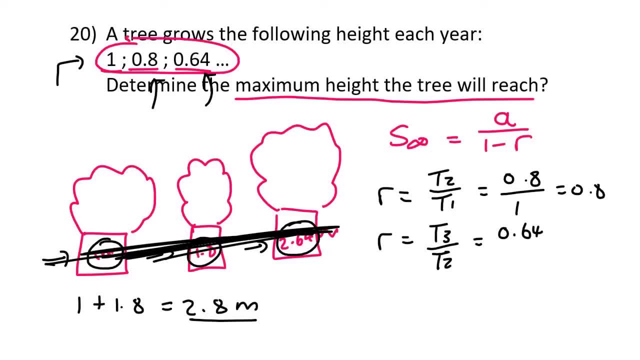 also try t3 over t2, which is 0.64 over 0.8.. And that actually does Give us 0.8.. So then we can go ahead and work out the sum to infinity as a, which is the first year's. 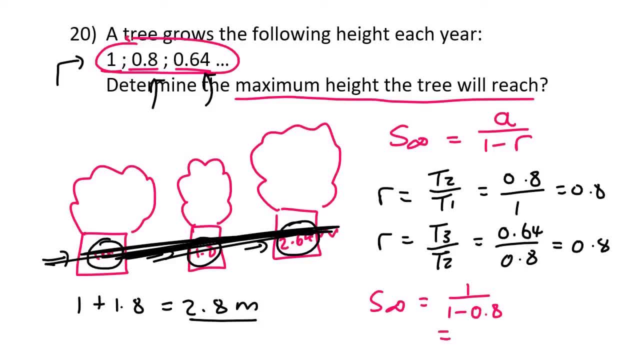 growth, which is 1 over 1 minus 0.8.. And that'll be 5.. I've seen a lot of students who try find the ratio using these numbers. But guys, those numbers don't make any pattern. You need to look at how. 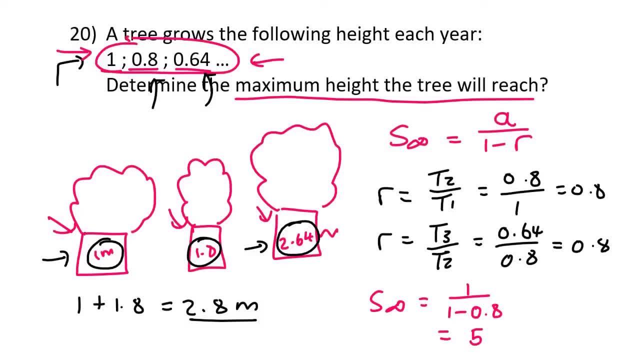 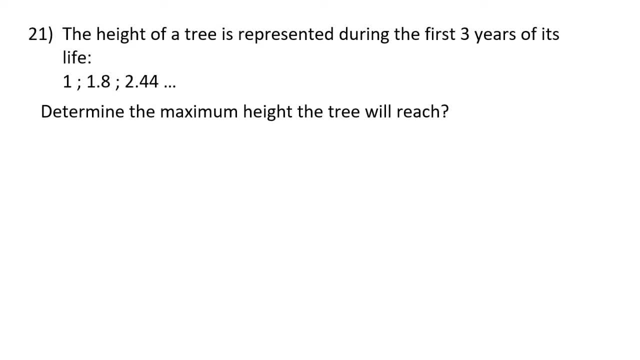 much does the tree grow by each year? Those are the numbers that are going to make any pattern That you want to add together. Question 21 is similar to question 20. But there's a slight difference in the way that we understand it and approach it. So what I see a lot of students do. 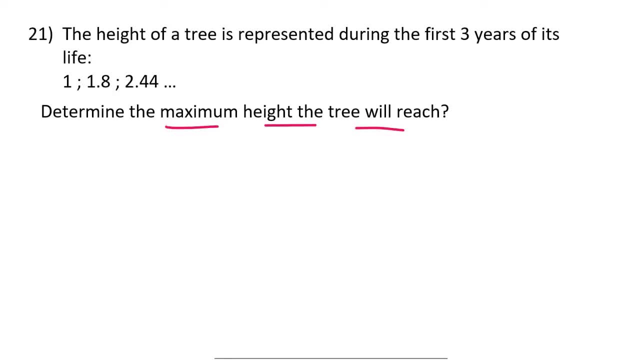 is they realize, okay, determine the maximum height of the tree, So they know that that's probably a sum to infinity question. But then what they do is they look at these numbers. Now, guys, these numbers represent the height of the tree each year. 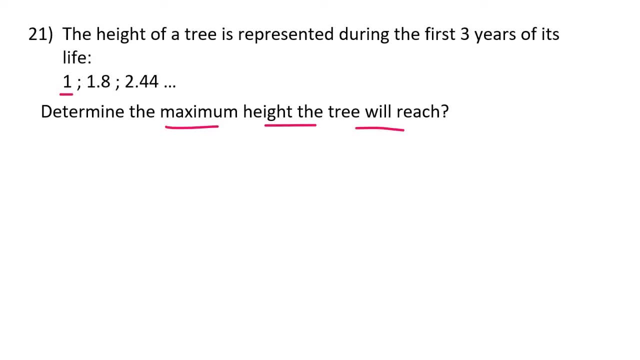 So after year one it's one meters tall, After year two it's 1.8 meters tall, And then after year three, it's 2.44 meters tall. No matter what you do, you will not be able to form a ratio. 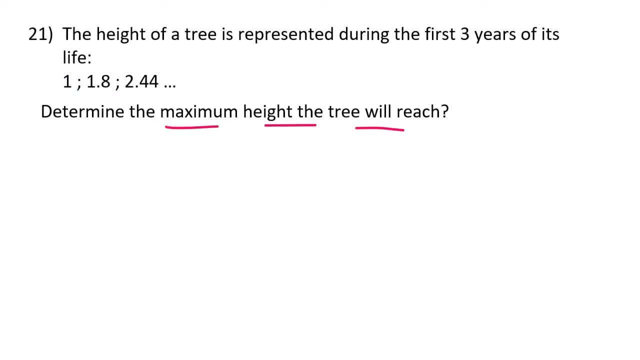 or a difference with those numbers. It just won't work. So then, Kevin, what is happening? Guys, the trick is: don't look at the height of the tree, Rather look at how much the tree grows Each year. that is where the ratio is. So in year one tree grows one meter, In year two, 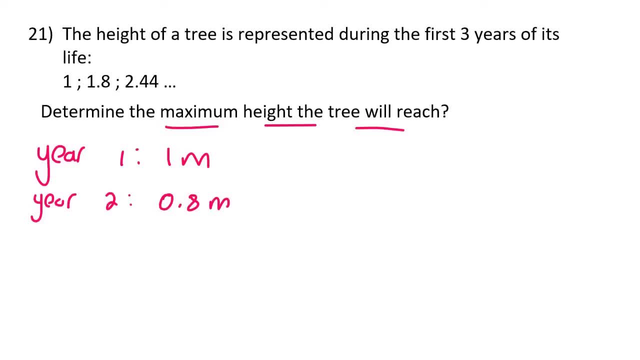 the tree grows 0.8 meters. So that's after two years it'll be 1.8 meters tall. In year three it grows 0.64 meters, Because if you add these three together now you would get 2.44.. 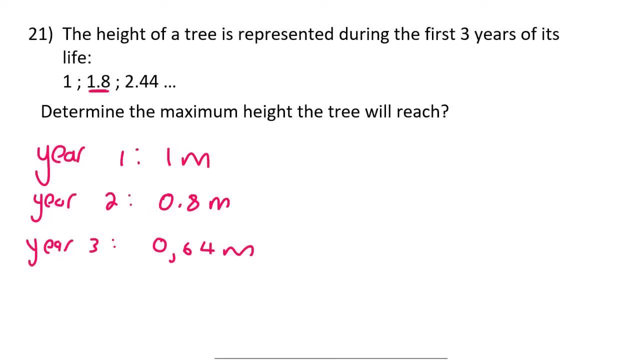 Now, these are the numbers, These ones that we've just found over here. they form a nice ratio. Let's see what is T2 over T1?? Well, that's 0.8 over 1, which is 0.8.. T3 over T2 is 0.64. 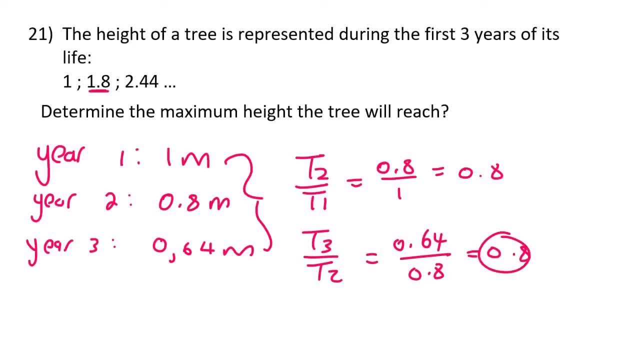 over 0.8, which is 0.8.. So there is a constant ratio. So to work out the total height that the tree reaches, you would have to add these numbers together. You wouldn't add these numbers together, That would make no sense. 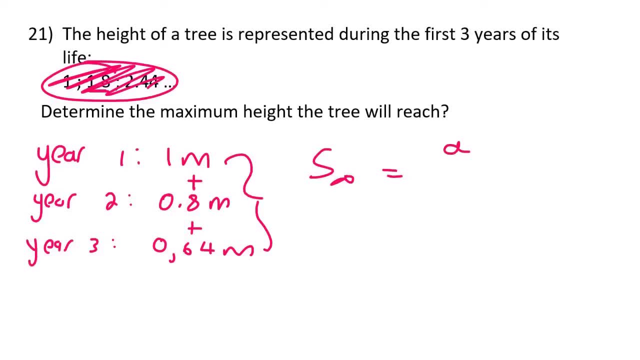 So we use the sum to infinity formula, which is a over 1 minus r, where a is your first term, which is 1.. And our common ratio we found was 0.8.. And that will give us 5.. This 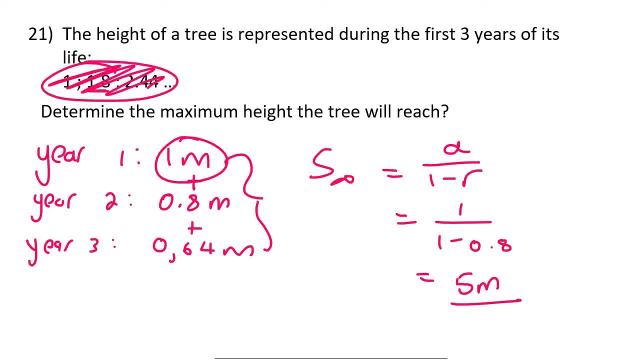 means the tree will only reach a maximum height of 5 meters Because these numbers, as we keep going, they become smaller and smaller and smaller And eventually they will reach 0.. What that means is that the tree will stop growing. 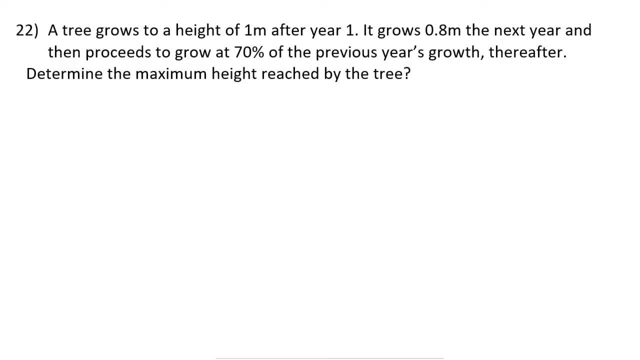 Question 22 is really good. It has a little trick that catches a lot of people out. It looks similar to question 20 and 21,. but there is something we need to be careful of. If you've already watched my explanation on 20 and 21,, you would have already learned that you must not. 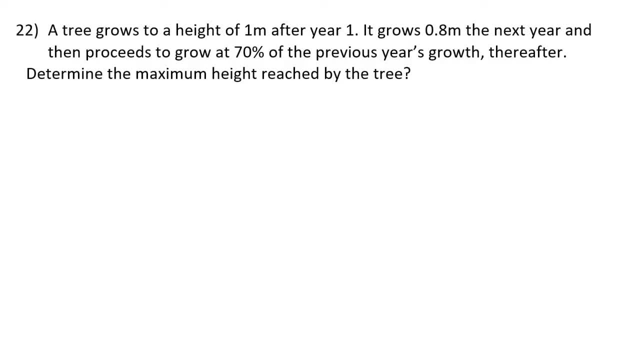 look at the total height of the tree, but rather look at the amount that the tree grows each year. that is where you will find the ratio or the pattern. okay, so in the first year it grows one meter. in year two it grows 0.8 meters. so I'm not going to say 1.8, I'm just 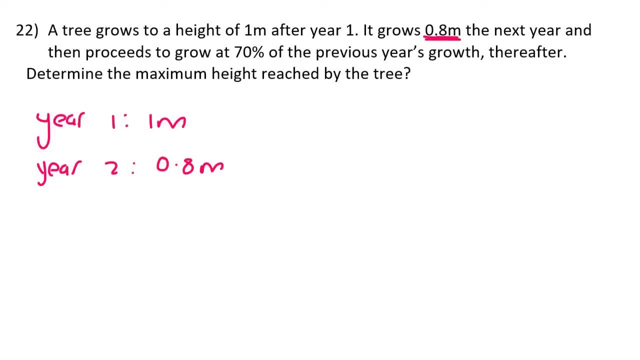 going to look at how much it grows by, and then they tell us that it grows at 70% of the previous year's growth. thereafter that means it just keeps going on and on and on. so in year three it'll be 70% of the previous year's growth. so it'll be 70% times 0.8, which is 0.56 meters. 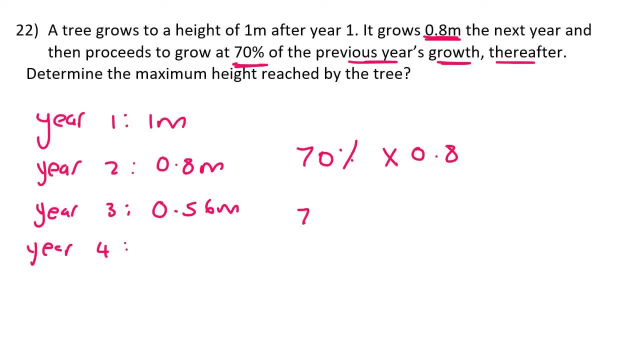 and then in year four it'll be 70% of the previous year's growth. so it'll be 70% times 0.8 of the previous year's growth, which is now going to be 0.56, which will give us 0.392. now we don't. 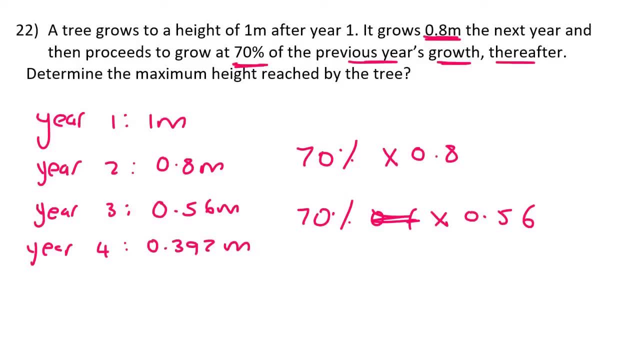 need to go any further now. check this out, guys. when did they bring in the 70%? the 70% only started here, so we need to be careful. is this also a 70% ratio, or let's check it out? so what we can do is: 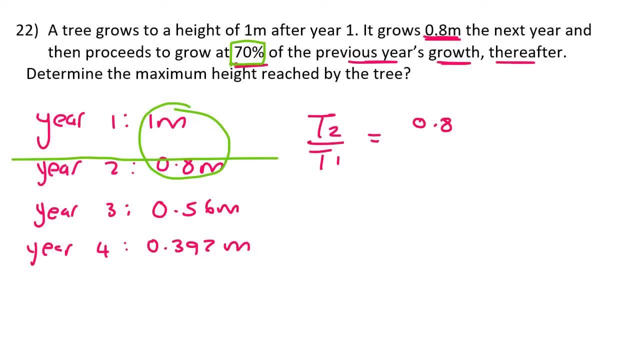 we can say term two divided by term one, and that's 0.8 divided by one, and that gives us 0.8. if we then say term three divided by term two, that'll be 0.56 divided by 0.8, which is 70% or 0.7. and if I say term four divided by term three, 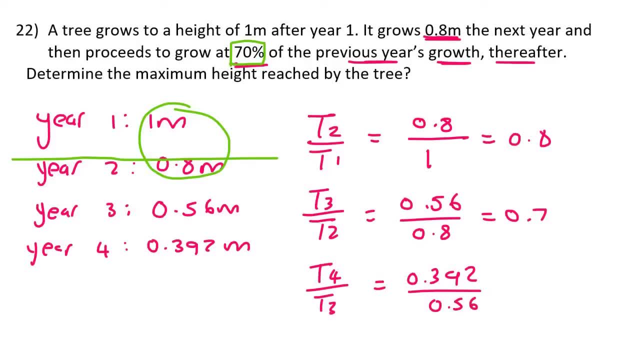 that'll be 0.392 over 0.56 and that'll be 0.7, and that 0.7 would obviously carry on because we keep using 70%. so the first number is causing a bit of a problem because it's throwing the ratio off. so what we do is we 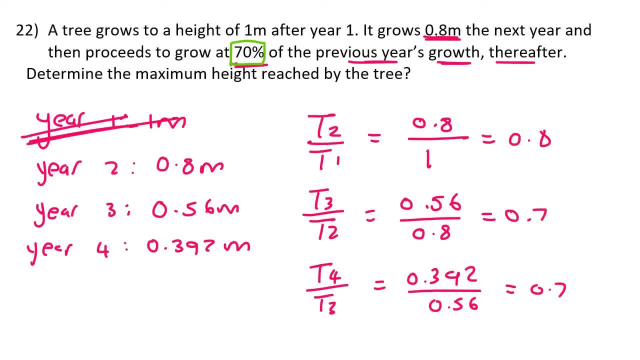 completely ignore the first year. let's forget about that. why don't we just add up all of these growths and let's see how much the tree grows, just from year two up to whenever it stops growing, up to infinity? because if we use some to infinity, we need to use some to infinity to get to the 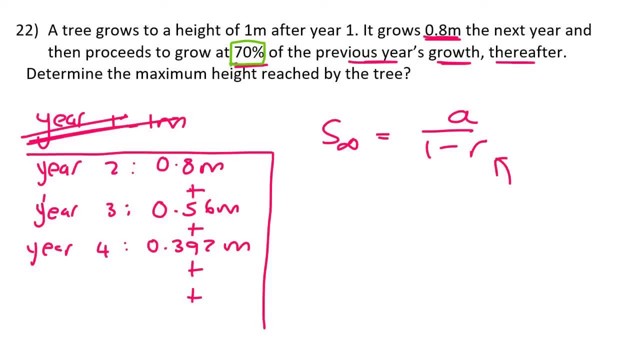 value of 0.9, which is exactly the same as the value of 0.8. the second did: 0.8 is the same as the value of 0.8 is 0.9 minus one, and if that is the case, we can now add up all the way to our. 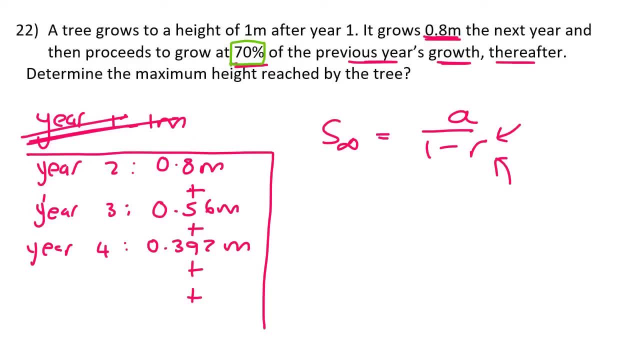 √5, and then we can do that by looking at our MapR算: this value and bringing it over to infinity, because that's 0.9, and to this value I'm going to use 0.8, and after doing that, I'm going to. 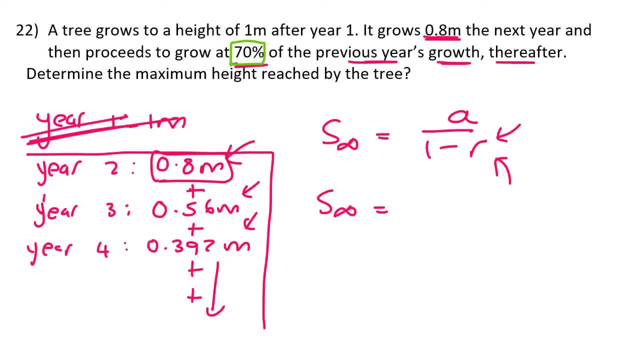 also is to use some to infinity and it would not be correct to use an r-value. and it would not be correct to use an r-value of 0.8, because the 0.8 only works for the first two. we also can't you 0.7, because the 0.7 doesn't work for the first part. so we just leave out the one meter for now, so we can say some to infinity now, because we only using these numbers, our a value is actually going to be 0.8. 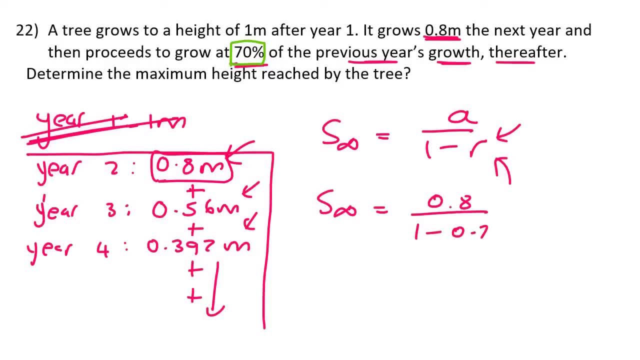 the ratio we can now use is 0.7, and this gives us 2.67 if you round to two decimal places. but now we must, okay. so what that means is that the tree, from year two up to infinity, it grows 2.67 meters. then all we do is we add on the one meter that it already had in the beginning, and 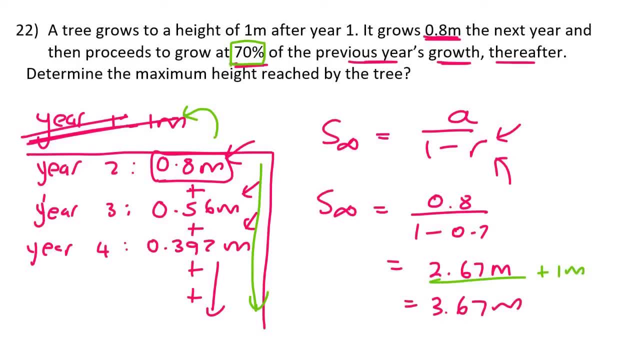 so the total height of this tree will be 3.67 meters. guys, they will never make it so that you have to check all the ratio numbers. it'll usually just be the first number that is out of place, and then you can just ignore that one. so just always look out for that first number. 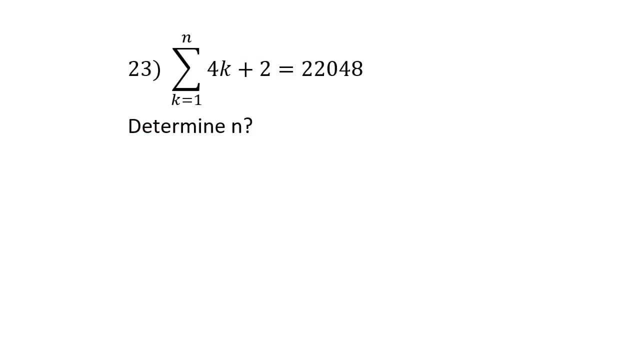 in number 23 we have a sigma notation question where we have to work backwards. what i've seen a lot of students do in the past is they think that this means 4k plus 2 is equal to 2, 2, 2, 0, 4, 8. 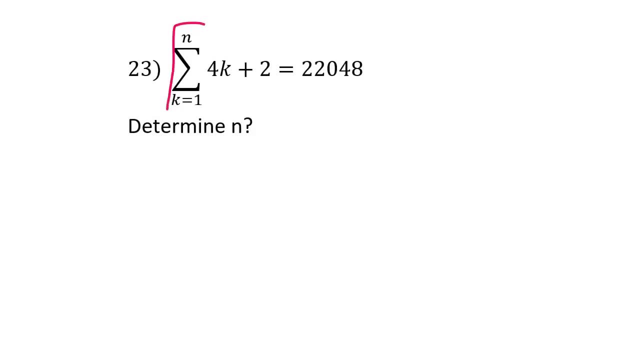 you mustn't read it like that. what it actually means is that the answer to the sum is equal to 2, 2, 0, 4, 8. but as always, let's find the first three terms, so to find term one, you plug in whatever. 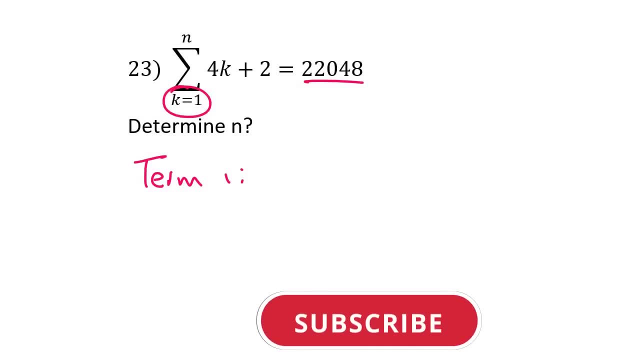 this number is which? in this case it is a one, so and so that'll give us six. term two is 10 and term three is 14, so what we have is an arithmetic pattern, because we can see that we are plussing four each time and we know that the sum of all the terms is 22 048, so we can use the sum. 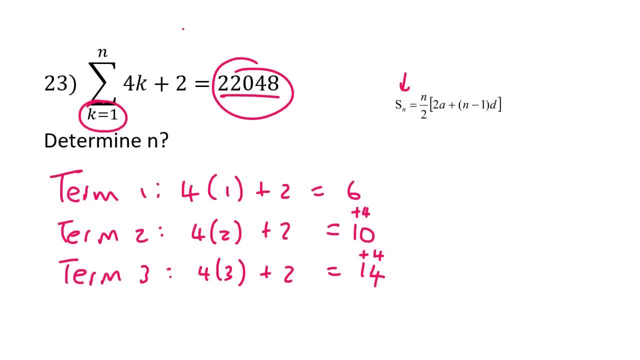 formula, and so what we do is we can say that the sum we already know, that is 22 048, and we can say that the sum of all the terms is 24 048. we don't know the number of terms, so we just leave that like. 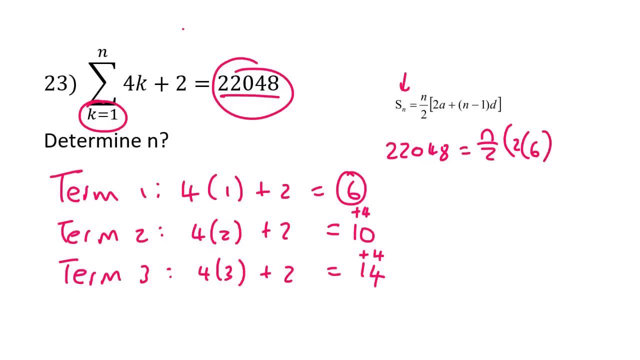 that a is term one, which is six. once again we don't know n, and the common difference is four. now what i like to do is i take this number two over here and i multiply that across, so we end up with forty four thousand and ninety six equals to n. then, on the inside, two times six is twelve. 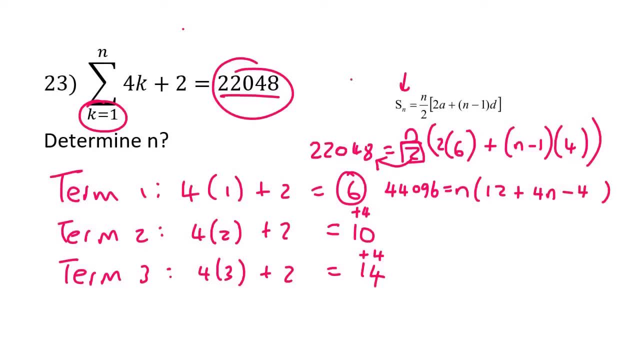 then i multiply this out four in minus 4.. I then put the 12 and the minus 4 together to make 8.. Then what I do is I multiply the n into the bracket, So that'll be 8n plus 4n squared, And then we get a trinomial, So we: 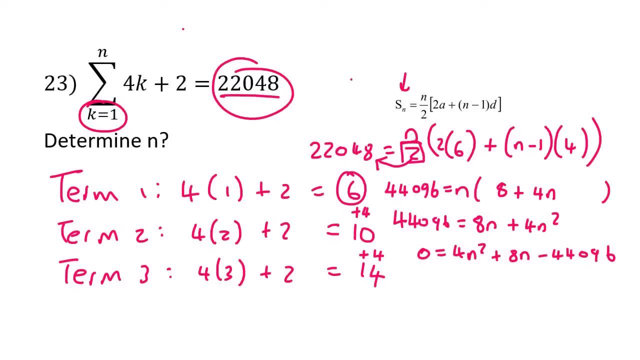 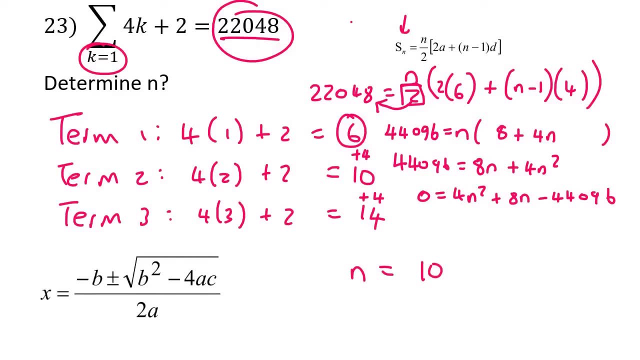 move everything to the one side, Then you could use the quadratic formula And you would find that n is equal to 104, or n would also be equal to negative 106.. But please remember that you can't have a negative n value due to the fact that n is a position, and you can't have a negative 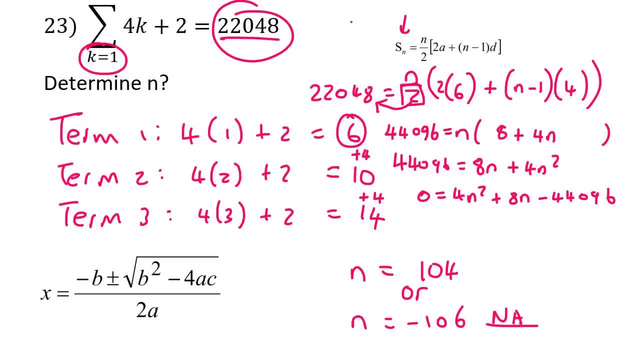 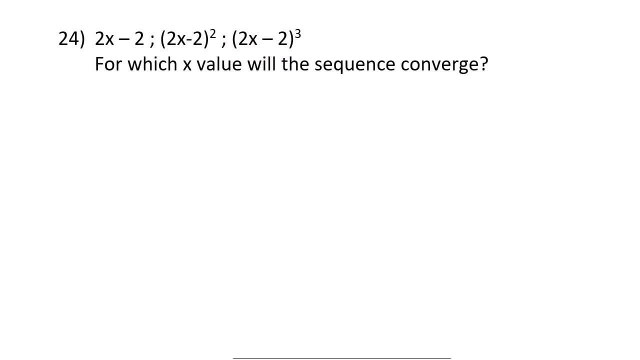 position. So this one will say na or no solution, And so therefore, our final answer is 104.. For something to converge, it's when the ratio is between minus 1 and 1.. So to find the ratio, you just say term 2 divided by term 1, which is 2x minus 2 squared over 2x minus 2.. Now 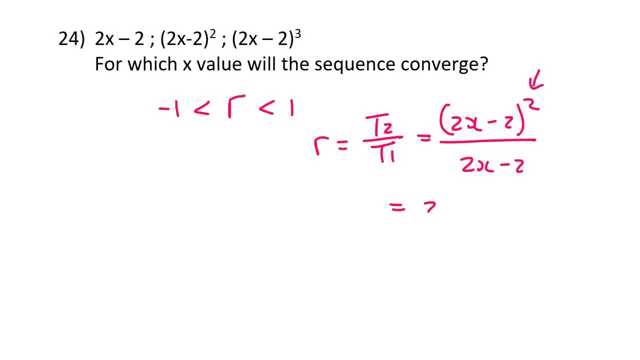 I'm going to make this. 2 over here means that there are two of those brackets, So it actually looks like this, And so one of them cancel like that, And so the ratio is 2x minus 2.. I then put that ratio in the place over there, And so my sum, or my equation, now looks like that. 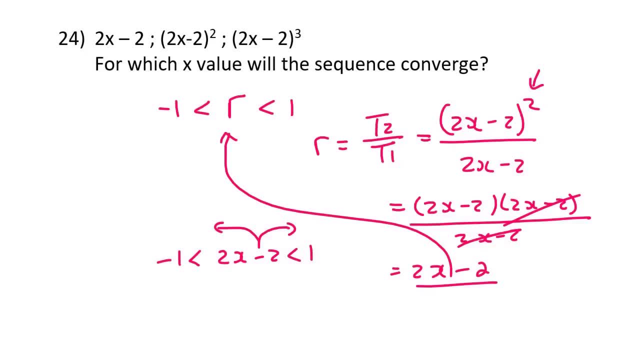 you then take the minus 2 to that side and to that side, So it'll become 1 and 3. You then divide everything by 2. So we end up with that. Question 25 is quite a challenging one, So we are. 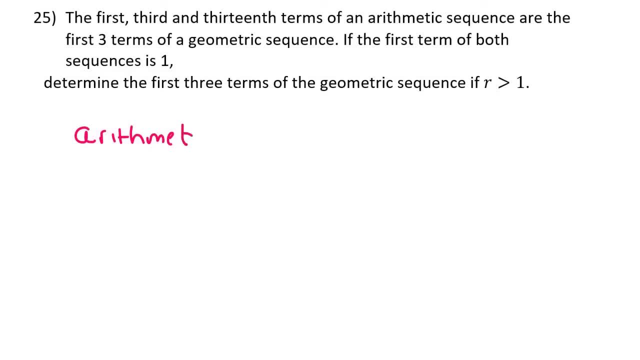 given information about an arithmetic pattern, And then we're given a given arithmetic pattern And, as well as a geometric, They tell us that the first term of both sequences is 1.. So we know that term 1 for this one is 1,. 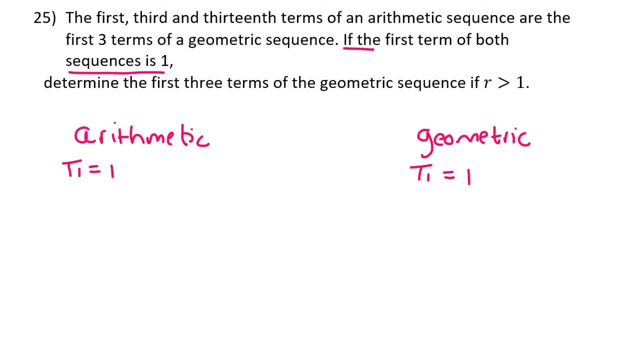 and term 1 for this one is also equal to 1.. Then they say that the first, third and 13th terms of an arithmetic sequence are the first three terms of a geometric sequence. So the third term in the arithmetic is the same as the second term of the geometric 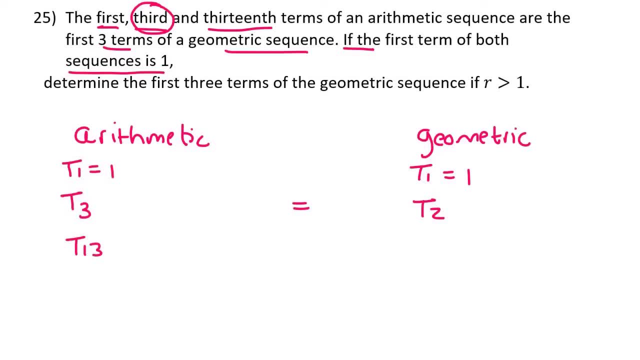 And then the 13th term of the arithmetic is the same as the third term of the geometric. Make sure that when you've read this, you understand what I've just done. They said that the first, third and 13th. here I've got them. 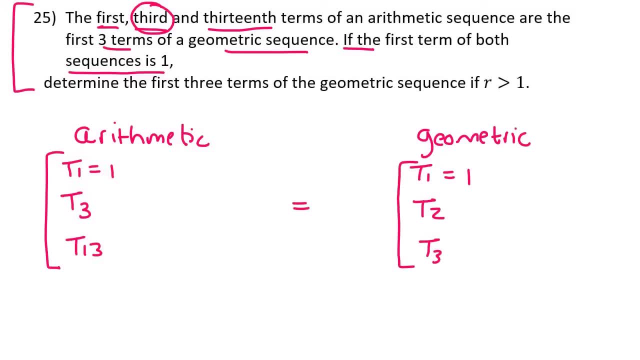 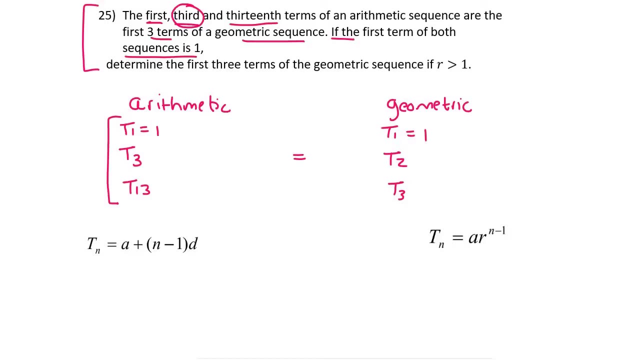 they are the first, second and third of the geometric. So that's all. That's all I've done there. What I would now do is use the formula for an arithmetic and also the formula for a geometric, And so for term 3 of the arithmetic, this one over here. 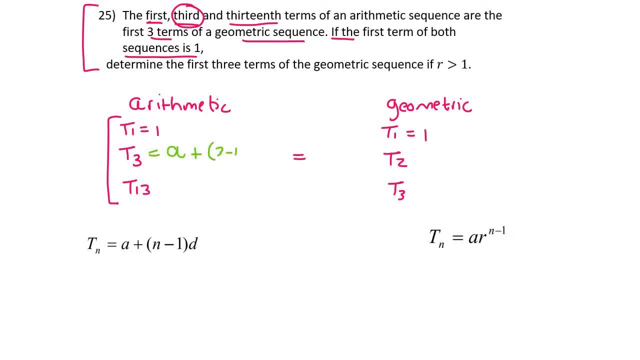 that would simply be equal to a plus 3 minus 1 times d. So if you simplify that, that'll be a plus 2d For term 13,. it'll be a plus 13 minus 1 times d, which is a plus 2d. 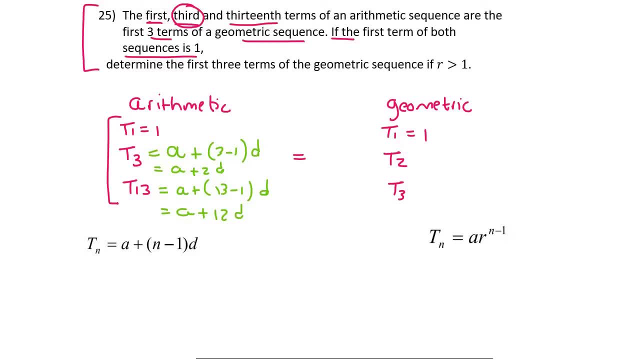 12d. Oh, but we know what a is, Remember. a is 1.. So we can go change all of these to a 1.. And then for the geometric for term 2, that would be a times r to the 2 minus 1.. 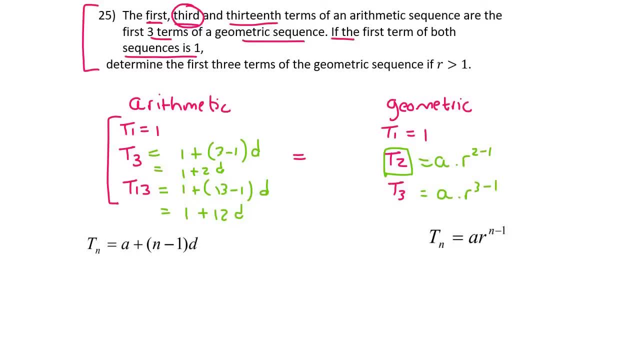 And then term 3 would be a times r to the 3 minus 1.. And then we could simplify. We know that a is 1.. So that's just 1 times r, because 2 minus 1 is 1.. 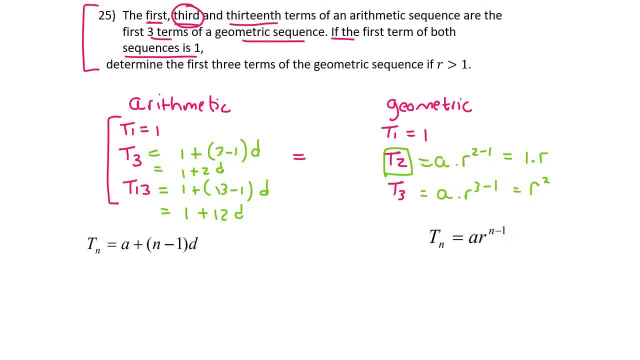 And then this one will be r times 2, or 1,, if you would like to, If you write it there, because a is 1.. So let's just highlight what we now have. We've now got this equation, this equation, this equation. 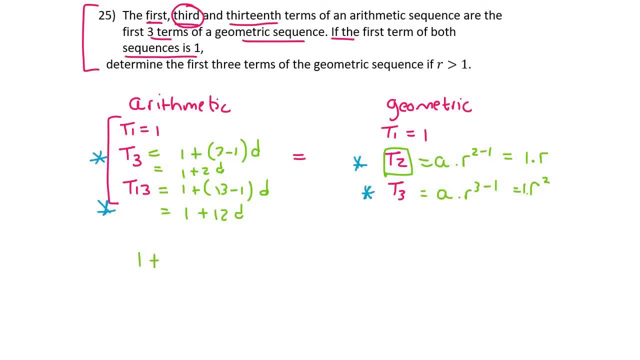 and this equation, So we can say that 1 plus 2d is the same as r. The reason I say that is that they said that this term is the same as this term. Then my other equation that I could say is: 1 plus 12d is the same as r. 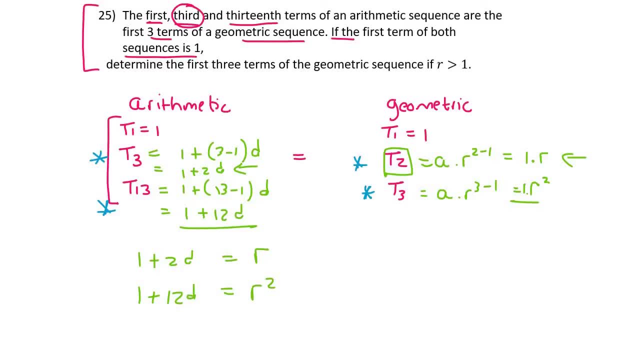 squared, because this must be the same as this. They told us that, And so here we have it, guys. We can use simultaneous equations on these two, So here we already have r. alone, r is equal to 1 plus 2d. 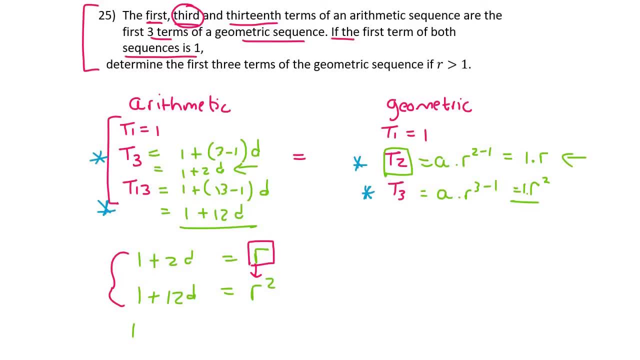 So I'm going to plug that into this equation. So we're going to end up with: 1 plus 12d equals 2. And then here we can replace this with 1 plus 2d squared, And now we just solve. 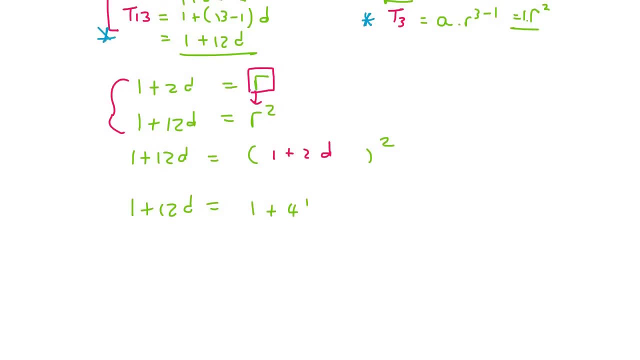 So 1 plus 2.. I'm going to just multiply this out, So it'll be 1 plus 4d plus 4d squared. If you had to make this into two brackets, then it's going to become a trinomial. 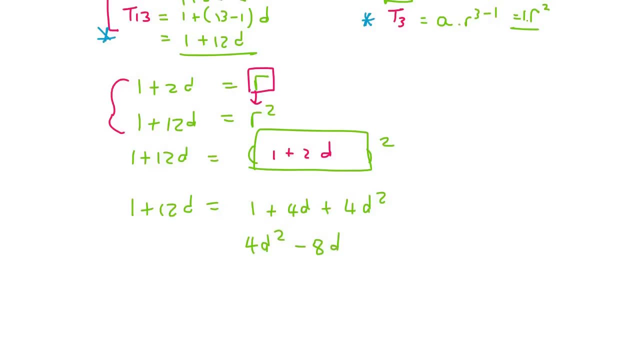 So we're going to get 4d squared minus 8d. Oh, but luckily the 1s cancel And so we get that. We can then take out d as a common factor. You can take out a 4 if you want as well. 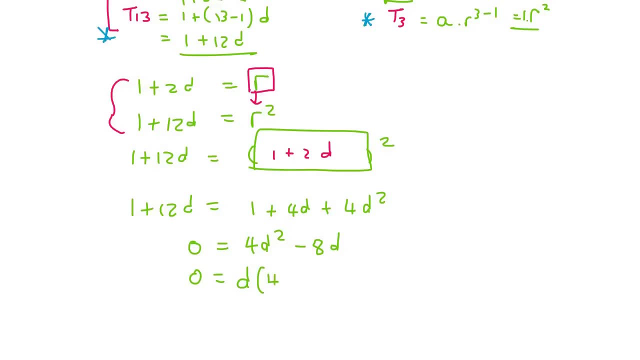 But it's not really going to make a difference. I'm just going to take out a d, And you'd be left with 4d minus 2.. Sorry, not 2, 8. And so we get d equals 2.. 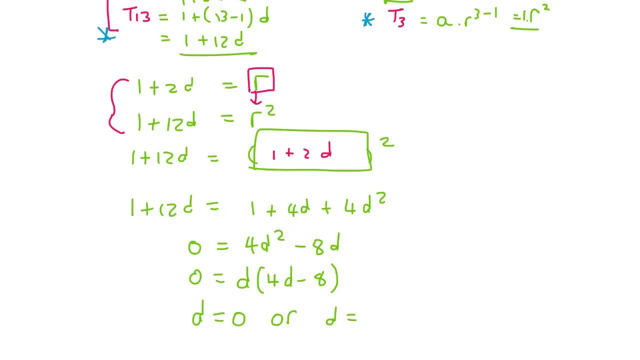 Sorry, not 2, 8.. Or d equals to 0, or d equals to 2.. Now that we have d, we can work out a. I mean r, because r is over here, So r is equal to 1 plus 2d. 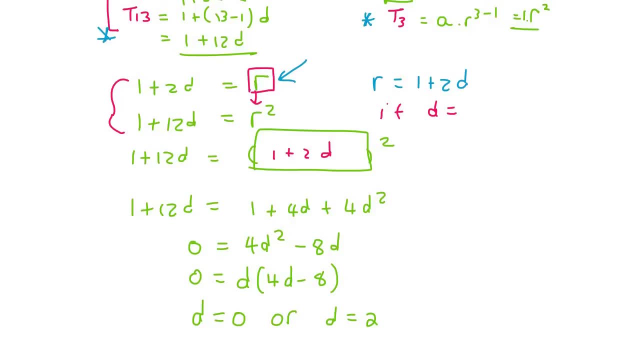 So if d is equal to 0,, then r would be 1 plus 2 times 0,, which is equal to 1.. If d is equal to 2,, then r would be 1 plus 2 times 0,, which is equal to 1 plus 2 times 2.. 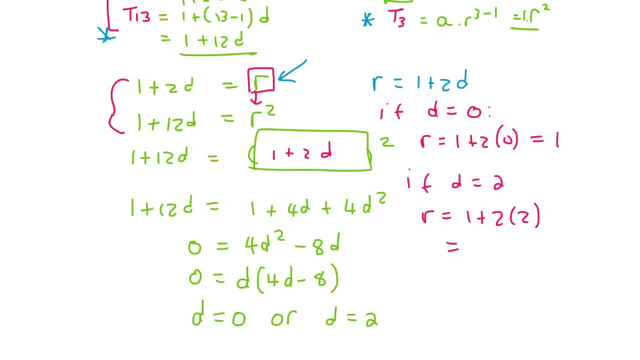 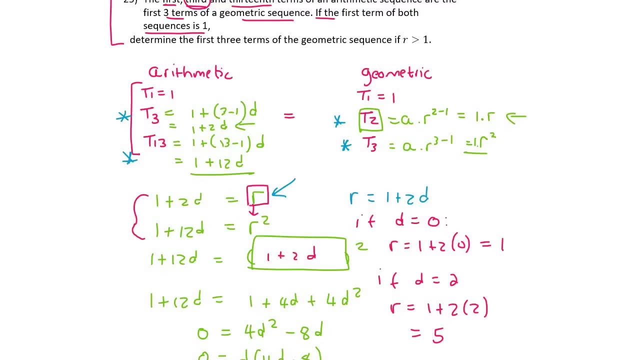 Then r would be equal to 1 plus 2 times 2. And so r would be 5.. I would just like to highlight something, though. They said that determine the first three terms of the geometric sequence if r is bigger than 1.. 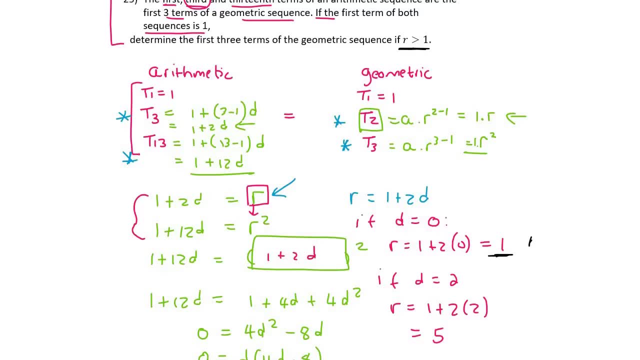 So if r is 1, that's not allowed. So this one is a no solution, which means that that d is also a no solution. d equals 0 is no solution, So the only valid one that we can use is this one over here. 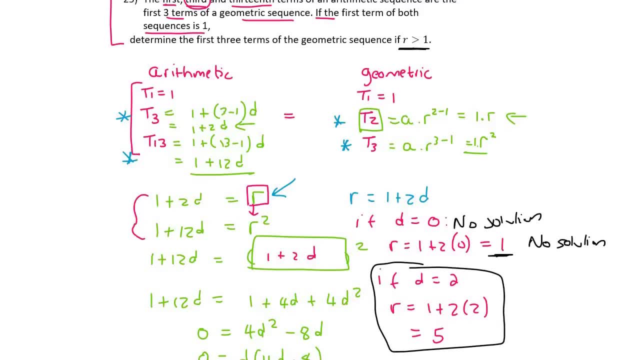 So this one over here, So this one over here. Now they want the first three terms of the geometric. So we know that term 1 is already 1.. Term 2 was this one, So it'll be 1 times r, which is 5.. 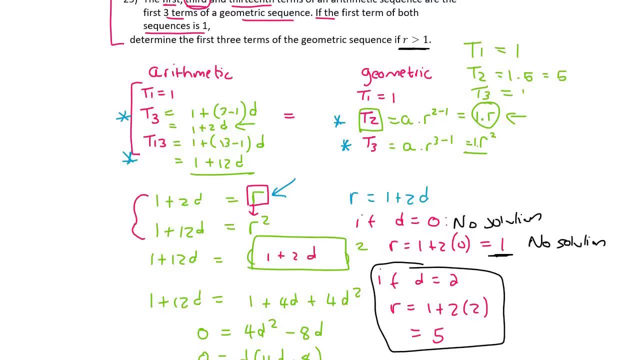 And that'll just give us 5.. And then term 3 would be 1 times 5 to the power of 2, which is 25.. And so those would be the first three terms of the geometric sequence, Question 26.. 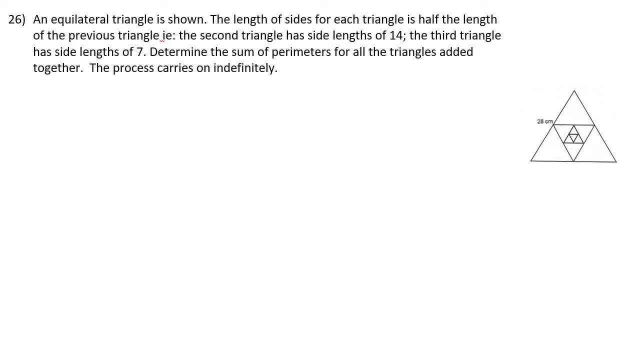 Question 26.. We are given an equilateral triangle and they give us the length of this side as 28.. Now, because it's equilateral, it means all sides are the same. So that's 28 as well, and this side is 28.. 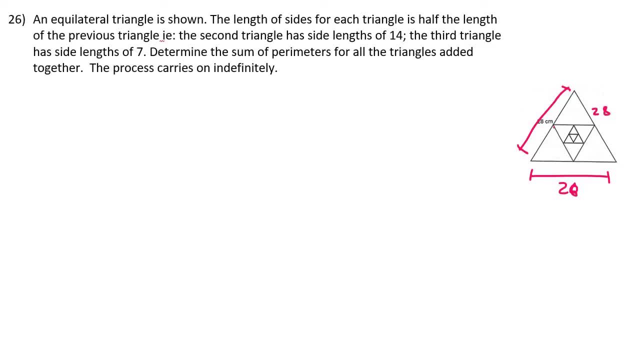 They tell us that the next triangle, which would be, for example, this one over here, has side lengths that are half of the previous triangle. That means that this would be 14.. This would be 14.. This would be 14.. 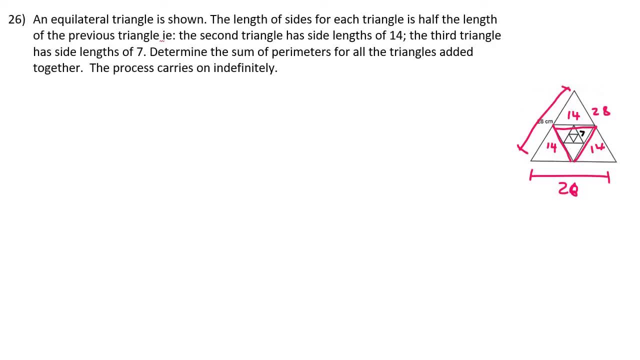 And then it would just keep going on and on and on. So your next triangle would be 7,, 7, and 7. They would like us to determine the sum of all of the perimeters. So for the first triangle, so I'm going to go triangle 1,. 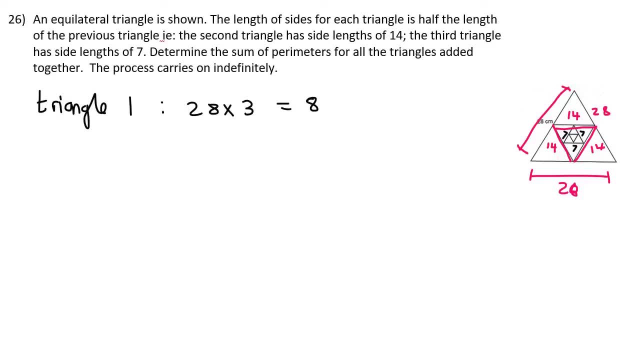 the perimeter would be 28 times 3,, which is 84.. For triangle 2, it'll be 14 times 3, which is 14.. Right, which is 42. And then, for triangle three, it would be seven times three, which is 21.. 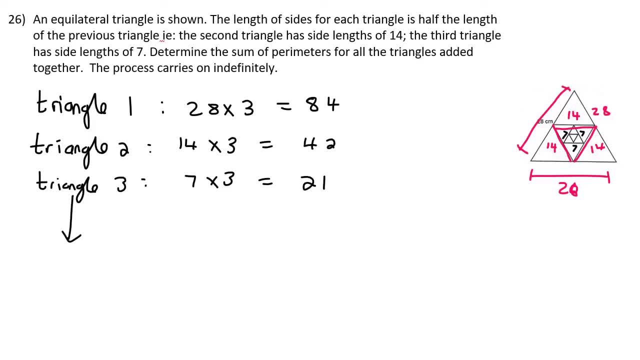 Now, of course, this process just keeps going on and on and on. That's what it means when they say indefinitely. So we don't know how many triangles there are going to be, And this is when we can use sum to infinity. Now we know that sum to infinity is a over one minus r, So all we need 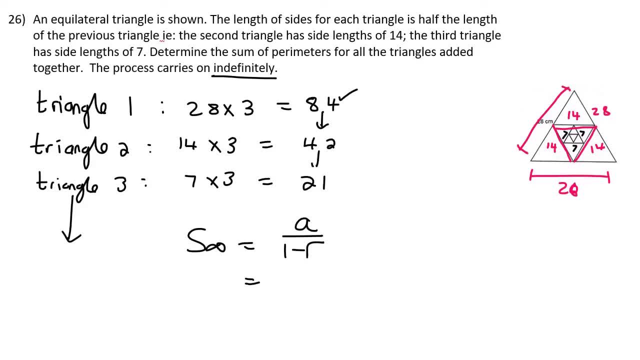 is a which is 84. And then we can see that there's a ratio here of a half. If you battle to find the ratio, you can just say: term two divided by term one, and that would be one over two. But yes, Kevin, how do we know that this carries on? Well, then you can go find the next. 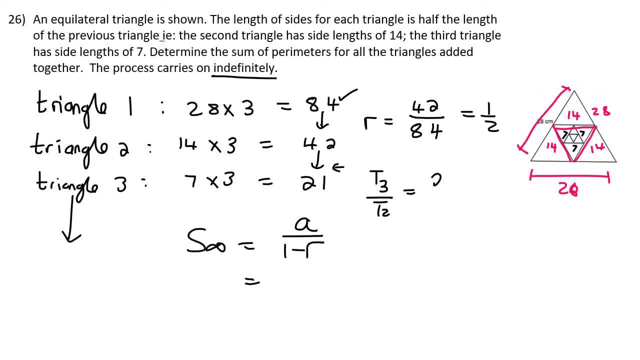 one. You can say term three divided by term two, which is 21 over 42, which is also a half. So the ratio is a half. So all we do is we say 84 over one minus a half, and that's going to be 100. 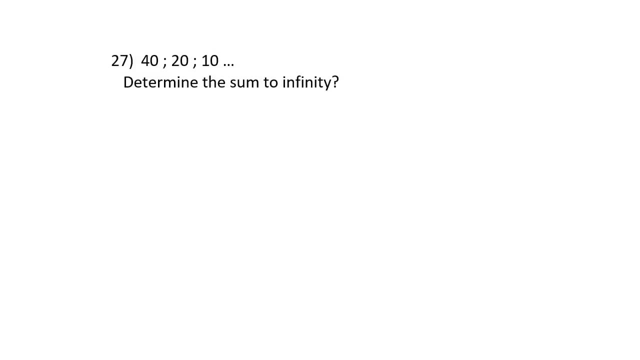 And 68.. The sum to infinity for this question is very easy. We know that the sum to infinity is a over one minus r. A is term one. And to work out r, you just say term two divided by term one, which is 20 over 40, which is a half. Yes, but Kevin, how do we know that that carries on Well? 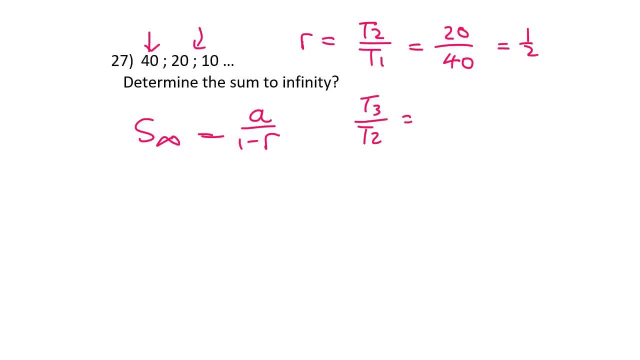 you can check the rest if you need to. Term three divided by term two would be 10 over 20, which is also a half. So it's easy: Sum to infinity is going to be 40 over one minus r, And to work out r, you just say term two divided by term one, which is also a. 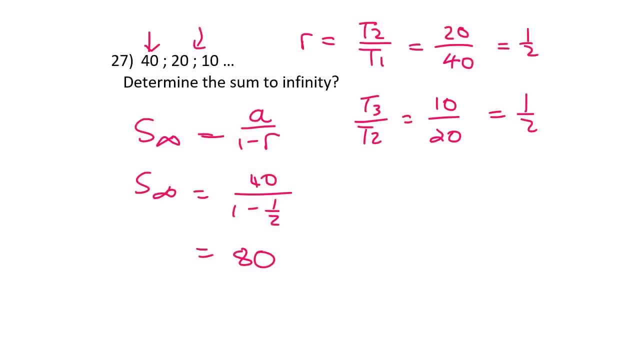 half, So it's easy. Sum to infinity is going to be 40 over 40,, which is also a half, So it's easy: Over one minus a half, which will eventually equal 80.. A good thing to do with sigma notation. 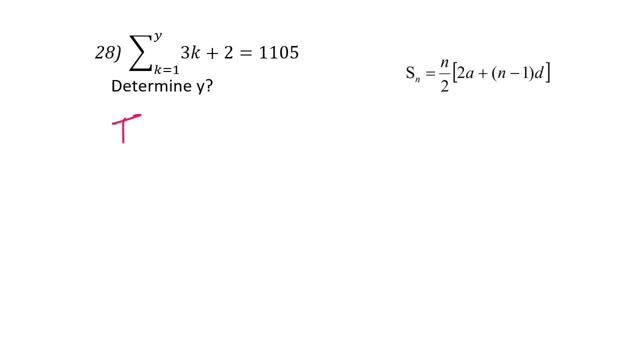 questions is to find the first three terms. So for example term one. you would start off by plugging in this number, So it'll be three times one plus two, which is five. Term two would be three times two plus two, which is eight, And then term three would be- you obviously plug in a three. 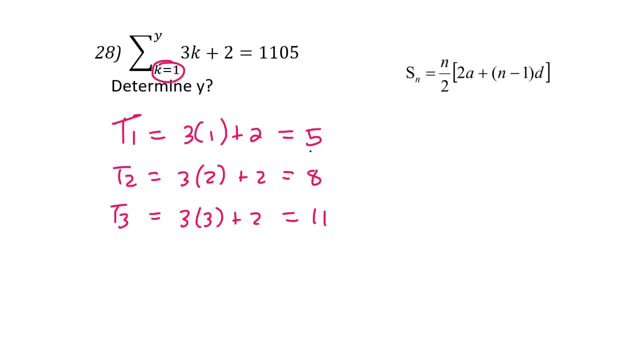 over there now and that'll be 11.. So we can see that we have an arithmetic equation. So we can see that we have an arithmetic equation. So we can see that we have an arithmetic sequence where we are adding three each time. And we also know that the sum of 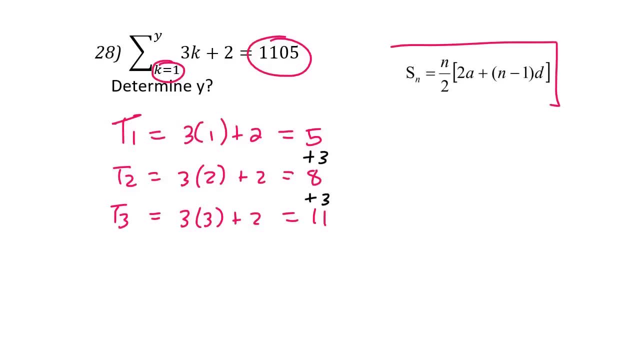 all the terms is 1105.. So we can use the sum formula of an arithmetic sequence. So I'm going to write that over here. We don't know the number of terms, so we'll just keep that as an n A is. 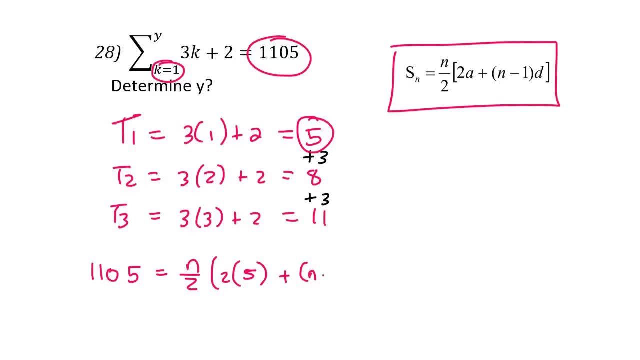 your term, one which is five N- once again, we don't know. And then d is your common difference, which is three. What I like to do here is multiply the two over, Which will be 2210.. And then I neaten up the inside, which will be 10 plus 3n minus 3.. I put 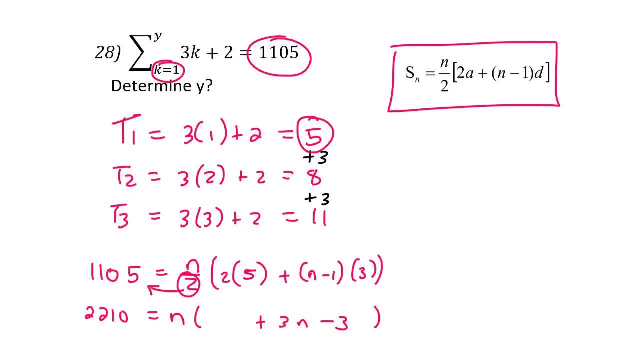 the 10 and the minus 3 together to make 7.. Then we can multiply the n into the bracket, So it'll be 7n plus 3n squared. We then bring the 2210 over so that we get a trinomial. 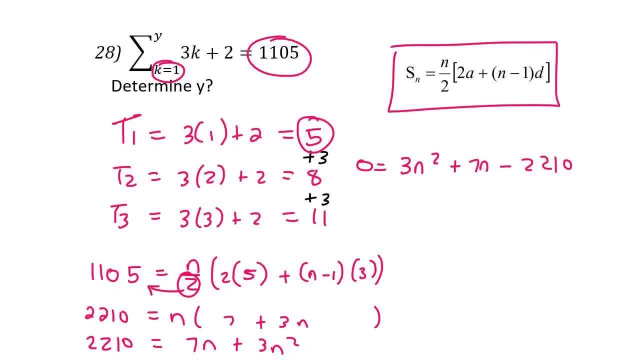 Then you can use the quadratic formula And you'll get that n would equal to 26 or n would be equal to negative 28.33.. But now you can't have a negative n value, So this one will be no solution. All right, So we found n, but that's not necessarily the same as y. Sometimes they 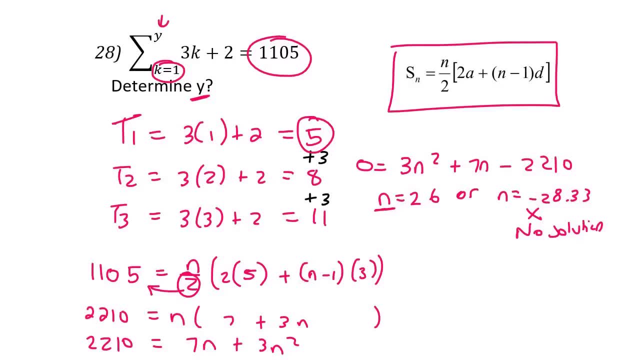 are the same. But remember what I showed you in previous videos or questions Is that to work out the number of terms, you always take the top, which is the y, minus the bottom, which is this: k equals to 1.. And then 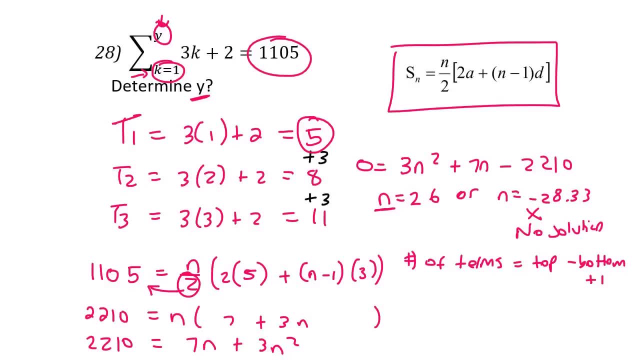 you always add 1.. So the number of terms, which we've just worked out as 26,, is equal to the top letter, which is y, minus the bottom, which is a 1 plus 1.. So in this scenario y will be 26.. But if 0 is the number of terms. y will be minus 3n, minus 3n. So this is the first term you're going to get in the next step. So you're going to have a number of terms, which is 6, plus the bottom. 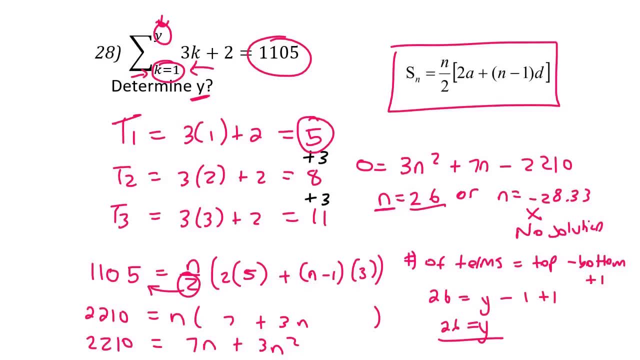 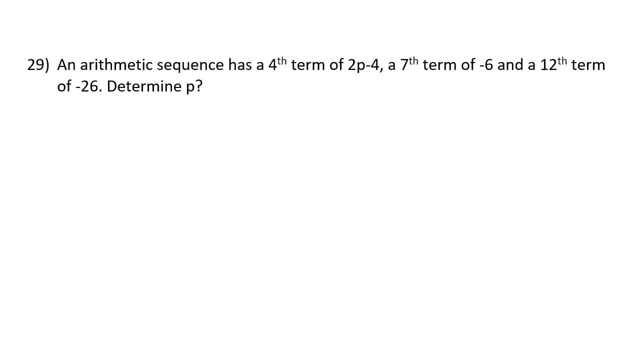 which is the bottom, which is 1 plus 1.. So you can always add 1.. And then you have to add the number. k value was something different, then you would have to be very careful because it wouldn't be the same as this 26 value. This is quite an interesting question. So when they do something, 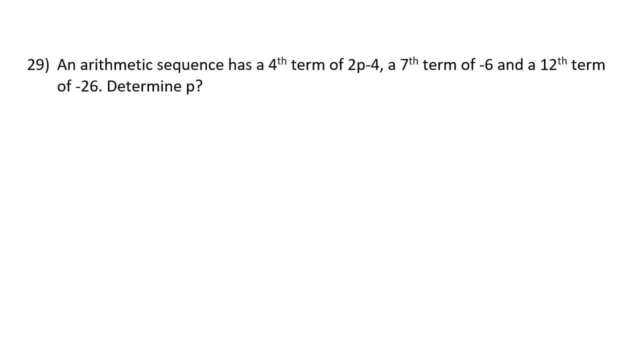 like this: just plug it into the formula. So they said it's an arithmetic sequence, so we use the arithmetic term formula. And so let's start with the first piece of information. They say that t4 has a value of 2p minus 4.. So we can say 2p minus 4 equals to a. 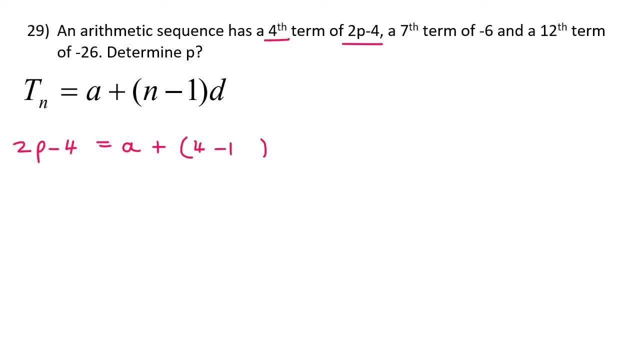 which we don't know Now. that's term 4, so we say 4 minus 1 times d. So we're going to say 2p minus 4 equals to a plus 3d. Oh, three unknowns. that's quite interesting. 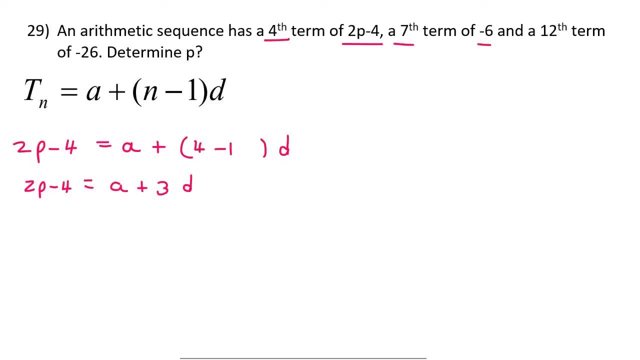 Then they say a seventh term equal to minus 6.. So we can say minus 6 equals to a plus. now it's a seventh term, so 7.. 7 minus 1 times d. Oh, and now I sort of see how this is going to play out. 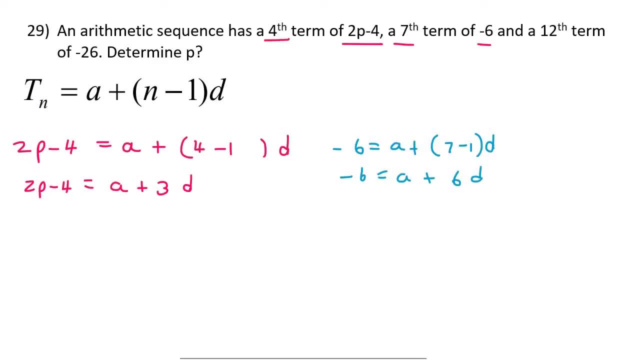 So we're going to say minus 6 equals to a plus 60. Then we need our third piece of information, a 12th term of minus 26. So we can say minus 26 equals to a plus 12 multiplied by d, which we don't know. 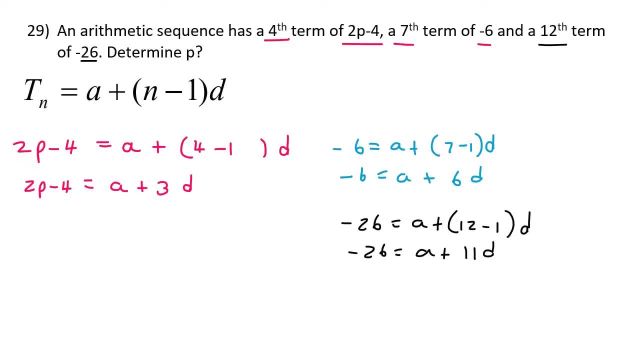 I'm just going to neaten this one up: 11d, All right. so I think what we can do is we use these two, This one and this one, And we solve simultaneously to find a and d. Then we can use the a and the d here to find p. 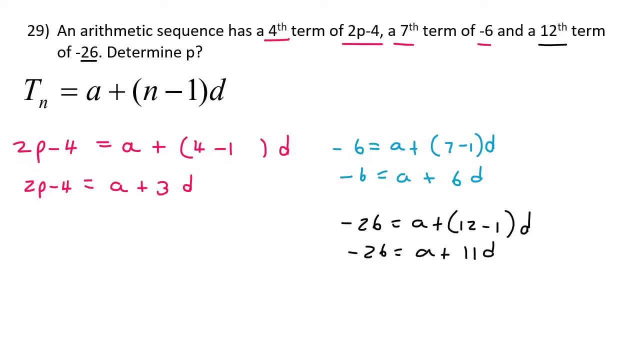 Does that make sense? Awesome, So you can solve this however you like, but I'm going to take this equation And I'm going to get a by itself. So if I do that, I'm going to find out that a is minus 6, minus 6d. 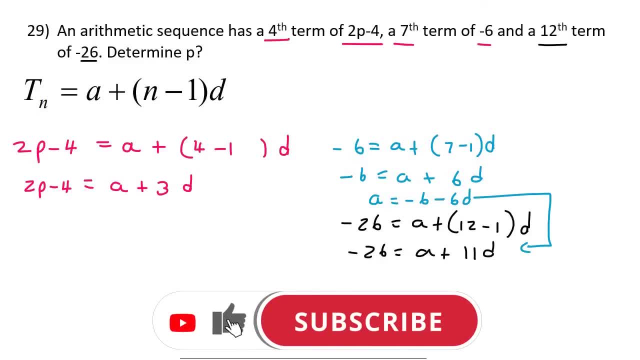 And I'm going to plug that into this. one's a, So. So it's going to look like this: It's going to go minus 26, equals 2.. And then a is minus 6 minus 6d plus 11d. 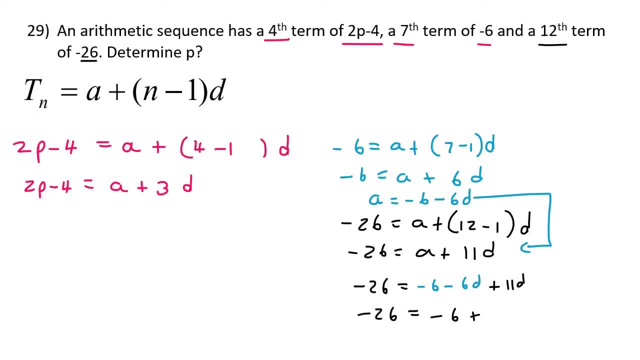 And so it's going to be: minus 26 equals 2 minus 6 plus 5d, And so if we do all the maths, we would eventually find that d is negative 4.. So we can plug that d value back into here. 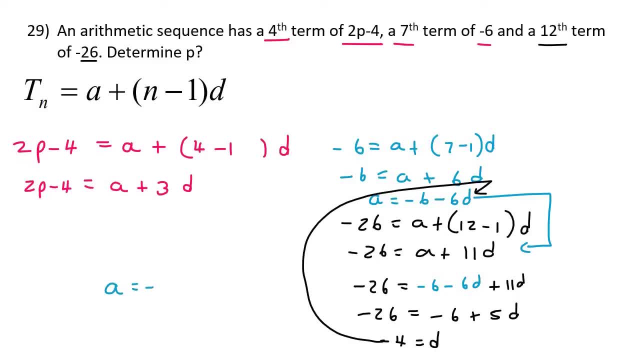 To find a, And so a is going to be minus 6, minus 6 multiplied by negative 4.. And so a would eventually equal 18.. Now that we have a and we have d, then we can find p, So we can plug everything into here. 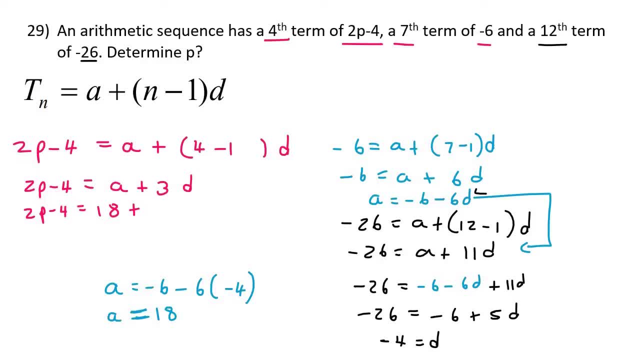 So 2p minus 4 equals to a, which is 18, plus 3 times d, which is negative 4. We would eventually see that 2p is equal to 10. And if you divide you would find that p. 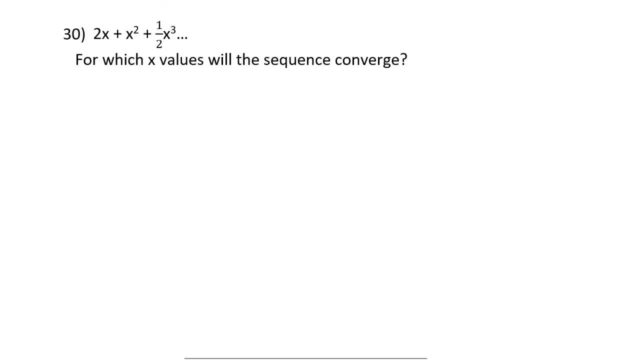 Is 5.. A converging sequence is one where r is between minus 1 and 1.. So to find r, you could say term 2 divided by term 1, which would be x squared over 2x. Now, to simplify this, an x would cancel at the top and the bottom. 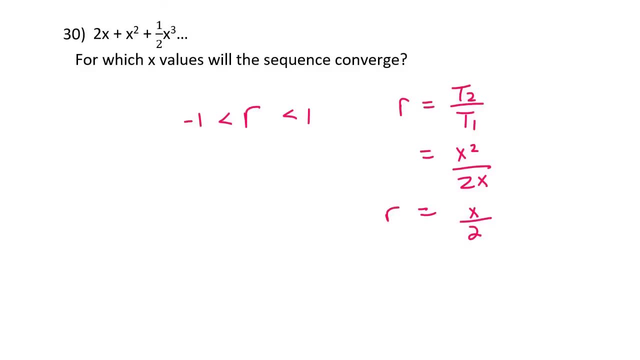 So you'd have x over 2 as your answer, Or you could even use term 3 divided by term 2.. It doesn't really matter. So that would be a half x to the power of 3 over x squared, And so the x2 would cancel and there would be 1x left over. 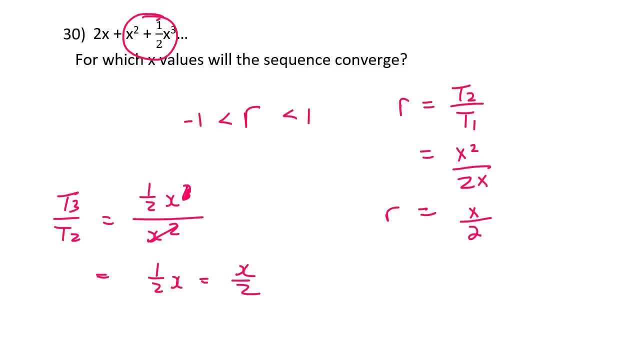 And so that's a half x, which is the same as x over 2.. These two are the same thing, So r is x over 2.. So you can plug it into there And then you can multiply this 2 over to both sides. 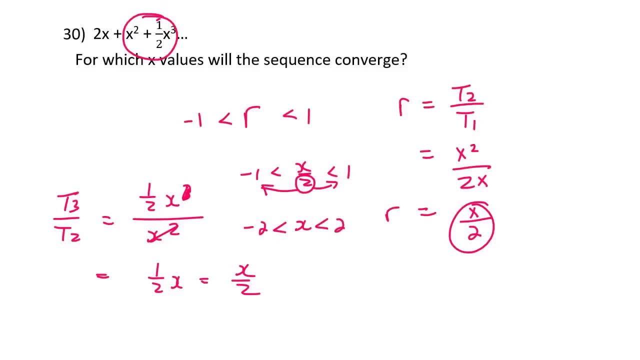 And so you're going to end up with: x is bigger than negative, 2 and smaller than 2.. In this question we are told that the sum all the way up to infinity is equal to 6.. But let's go find the first three terms first. 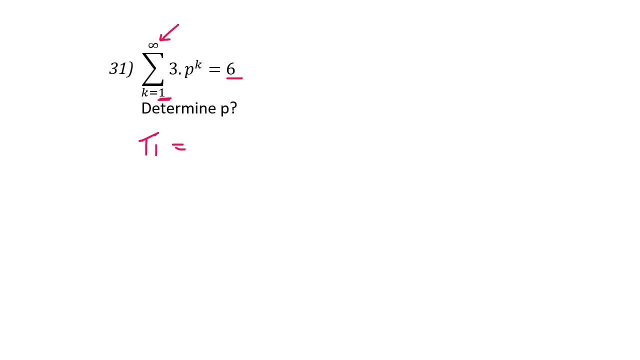 So to find term 1, you would plug this number into the place of k, So that's going to be 3.. And now some people are going to be like Kevin: what about p? Don't worry about that, Just keep it as p for now. 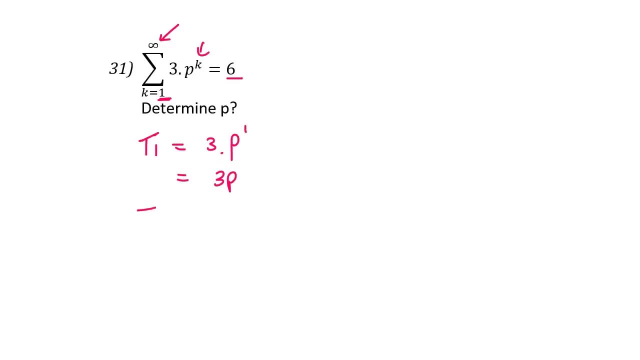 And then that's the power of 1.. So that actually just equals 3p. Term 2 would be 3 times p to the power of 2, which is just 3p squared, And then term 3 would end up being 3p cubed. 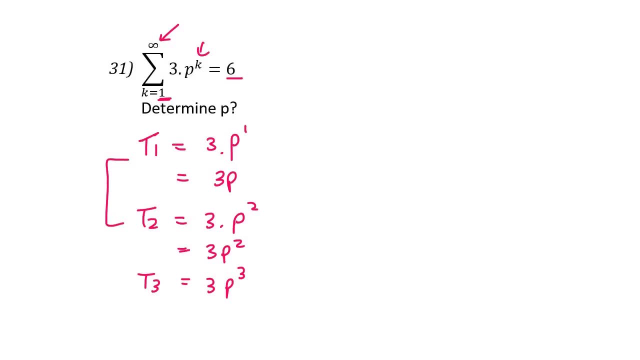 So we only really needed the first two, because we know that it's a geometric sequence, because only geometric sequences can go to infinity. So we don't need to check up on that, But we need to find r Now. r can be term 2 divided by term 1, which is going to be 3p squared over 3p, which equals p. 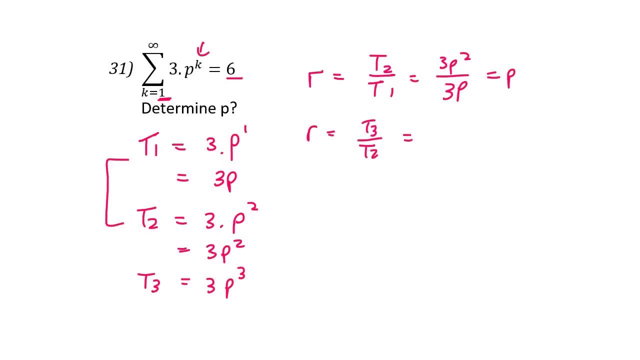 You could also use term 3 divided by term 2 if you wanted to. That would be 3p cubed, 3p cubed over 3p squared, which is also p. All right, So we know what r is. 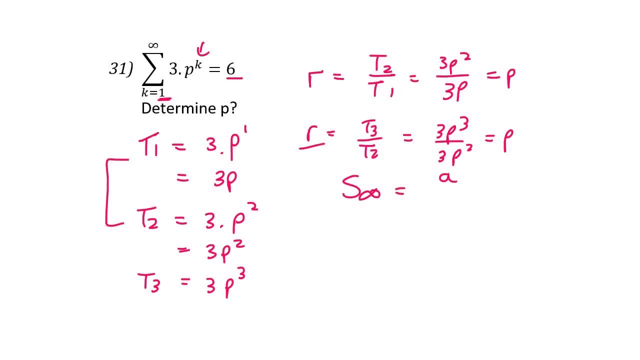 It's p. Now we know that sum to infinity is a over 1 minus r. Now the sum to infinity is 6.. a is term 1, which is 3p. See how I just plug it in. I don't really worry about p. 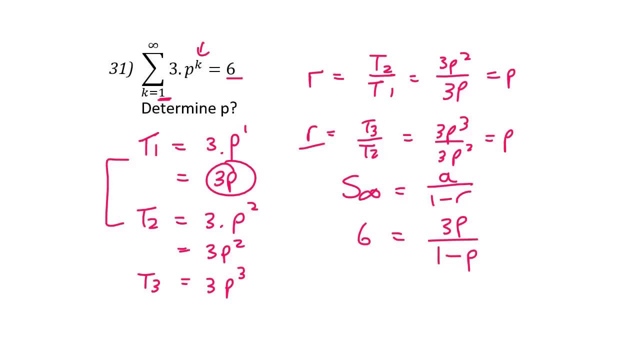 I just plug it in as it is. Then r is p. Now what I would do is I'd multiply this 1 minus p over, So it would become like that You can then say 6.. 6 minus 6p equals to 3p. 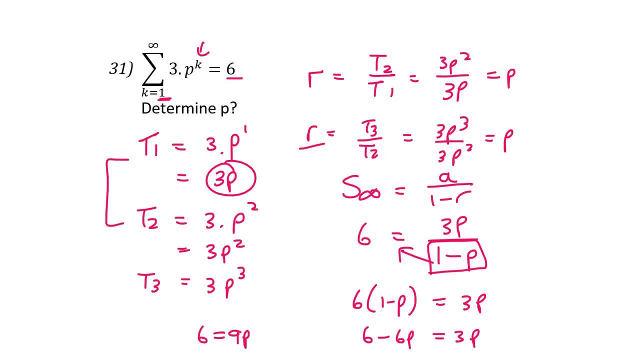 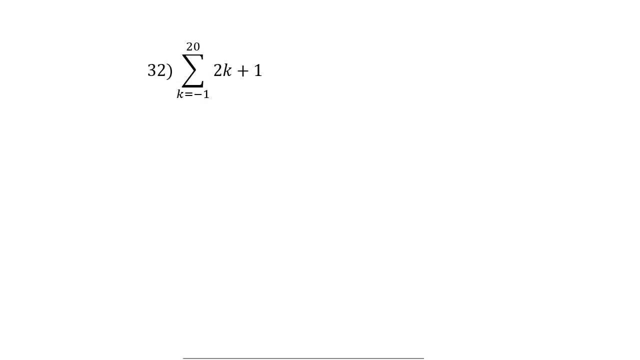 You would eventually end up with 6 equals to 9p, And then, if you divide, you should eventually get p is 2 thirds. When I give some of my students a question like this, they often look at me as if to say: 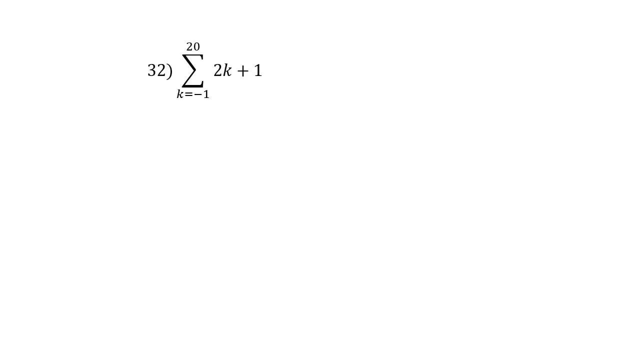 Kevin, what is the question? Like you're giving us this, but what do you want us to do? And what you need to remember is that this symbol stands for sum of, So it's actually asking you to calculate the sum of the sequence. 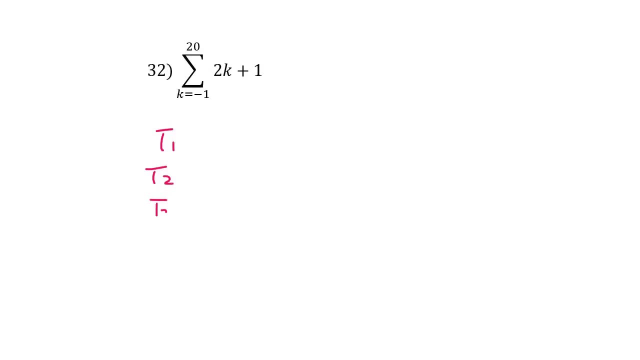 So you need to go find term 1,, term 2, and term 3, just to work out if it's arithmetic or geometric. To find term 1, you start with whatever number is over here. That number does not have to always be a 1.. 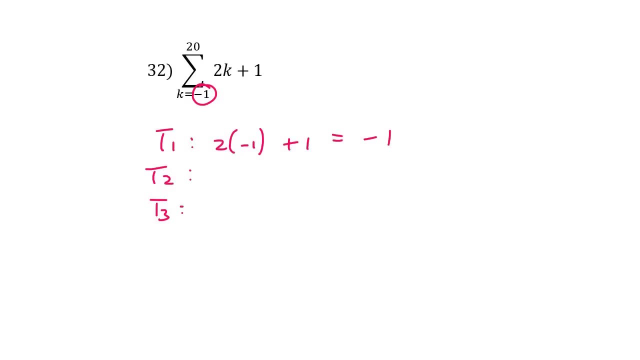 So you'll plug it in and that's going to give us negative 1.. Then to find term 2, you are going to be careful here. You must always add Add 1 to this. Now, if you add 1 to that, it actually becomes 0.. 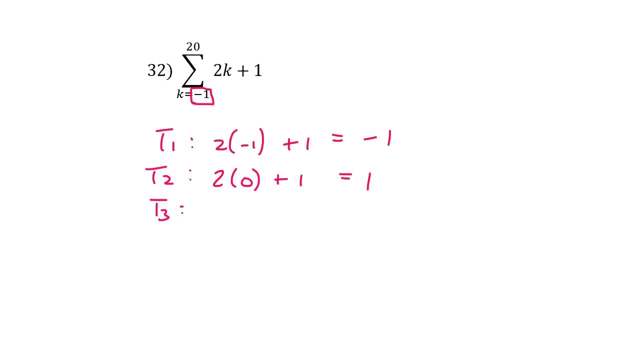 So then it'll become 2 times 0 plus 1,, which is 1.. And then you add another 1,, so it'll become 1.. So it'll be 2 times 1 plus 1,, which is 3.. 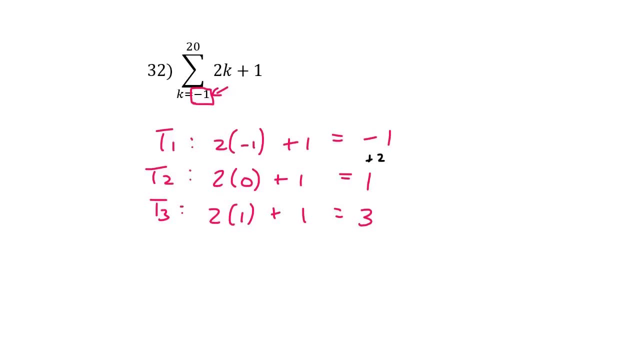 So it's definitely an arithmetic pattern. We're adding 2 each time, So we can use the arithmetic formula. Now, guys, if you've looked at some of the previous questions, you'll remember that this number is not always the number of terms. 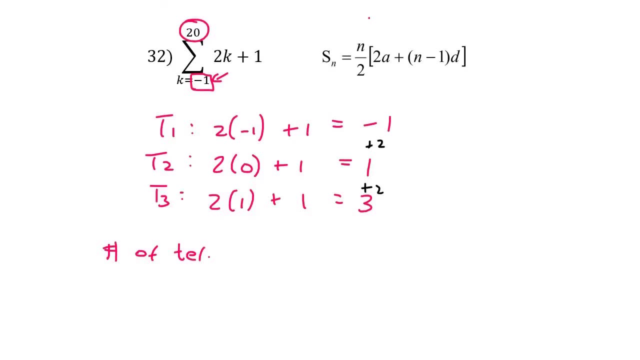 To work out the number of terms, you take the top minus the bottom, which is this bottom number here, and then you plus 1.. So the number of terms is 20 minus minus 1 plus 1. And so that actually becomes 22.. 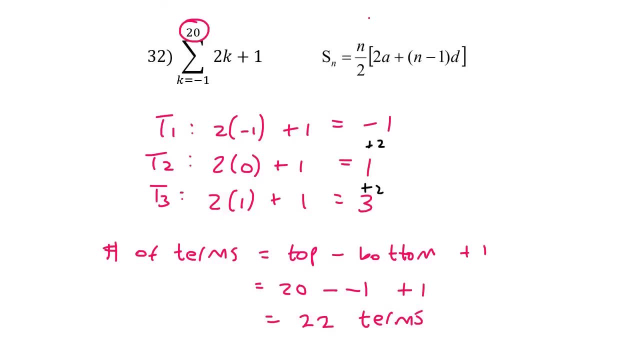 There are 22 terms. If that caught you out, don't worry, It catches a lot of people out. It's because when your teacher explains this to you in class, they always make this number at the bottom, And so it makes you think that this is the number of terms. 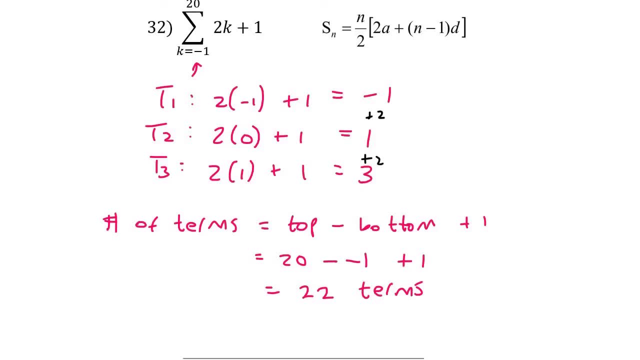 but it's not true, Only sometimes, And so now it's just a matter of filling in. So that's just going to be 22 terms. A is term 1,, which is negative 1.. 22 minus 1, and the common difference of 2.. 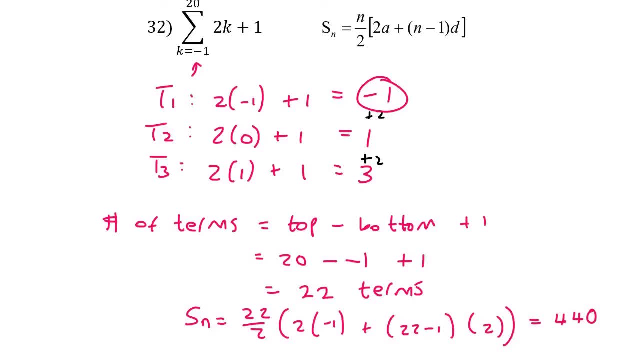 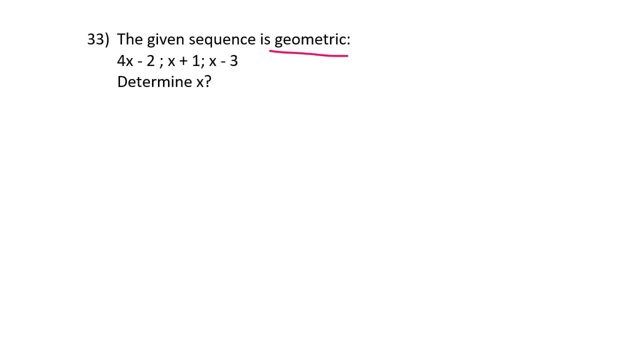 And so we end up with a final answer of 440.. They tell us in this question that we have a geometric sequence. A property about geometric sequences is that term 2 divided by term 1 will always be the same as term 3 divided by term 2.. 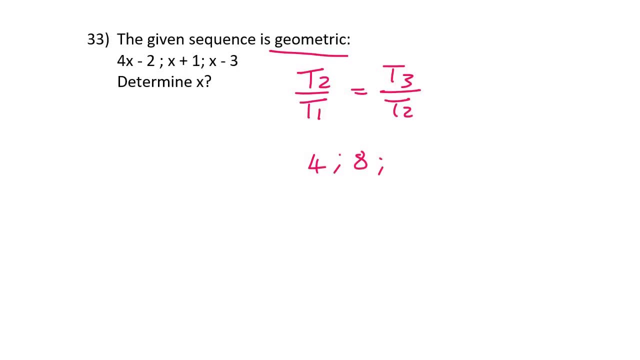 Want some proof. Well, imagine we had a sequence that goes 4,, 8, and 16.. That's a geometric sequence. If I take term 2 divided by term 1, that gives me 8 over 4,, which is 2.. 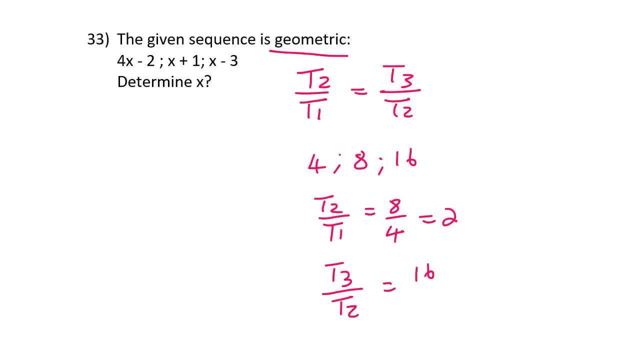 If I say term 3 divided by term 2,, that will be 16 divided by 8, which is 2.. So the ratio remains constant. So when they give you a question like this, all you do is you write this out. 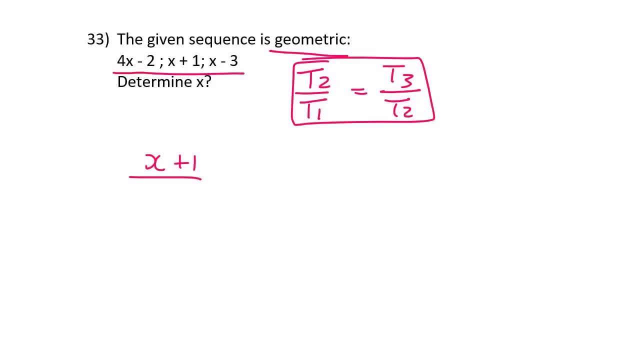 And then you just fill everything in. So it's x plus 1 over 4x minus 2 equals to x minus 3 over x plus 1.. Do cross multiplication next, So you end up with x plus 1 times by x plus 1 equals to x minus 3 multiplied by 4x minus 2.. 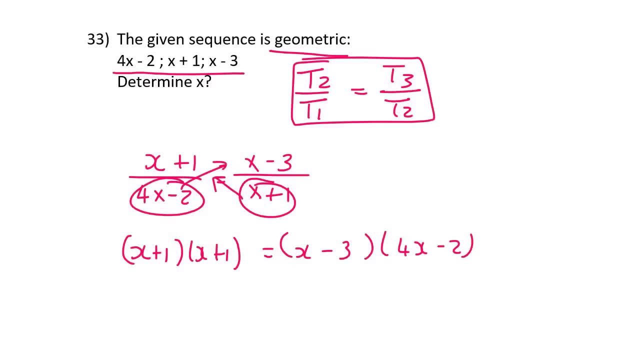 You see. so what I did there is: I just took these numbers across. We're then going to multiply out. I'm going to do it fairly quickly, because you guys do know how to do this. I'm then going to take everything to one side. 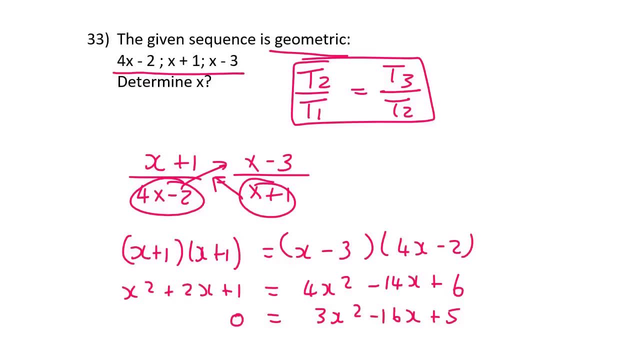 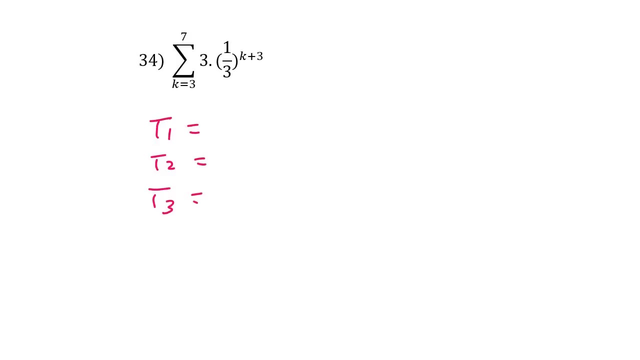 And then I would use the quadratic formula And so we would find that x is 5 or x is a third For a sigma notation question. we usually just go find the first three terms just to see if we're busy with an arithmetic or geometric sequence. 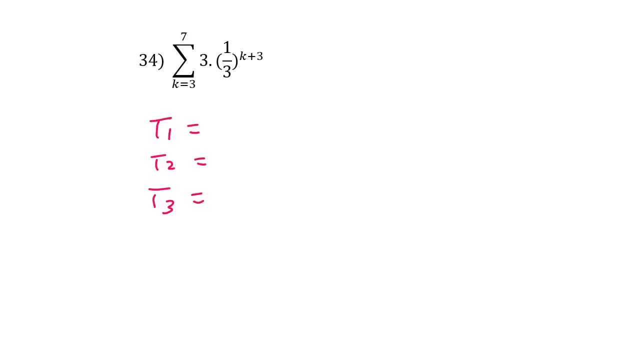 To find term 1, you start off with whatever this number is, So that'll be 3 times a third to the power of k, which is 3, and then plus 3. And that'll give us 1 over 243.. 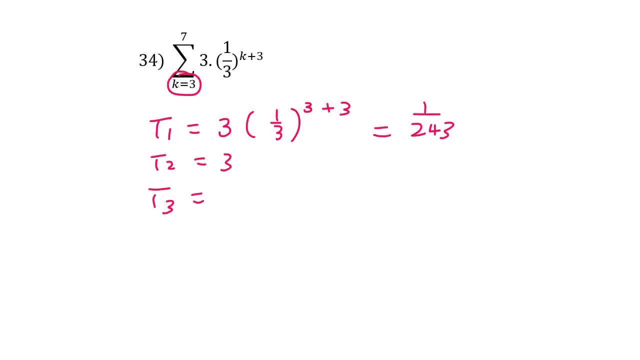 I wouldn't recommend using decimals at that step. Then for the next one, you just make k go up by 1.. So that's going to be 4 plus 3, like that. So that's 1 over 729.. And then the last one. 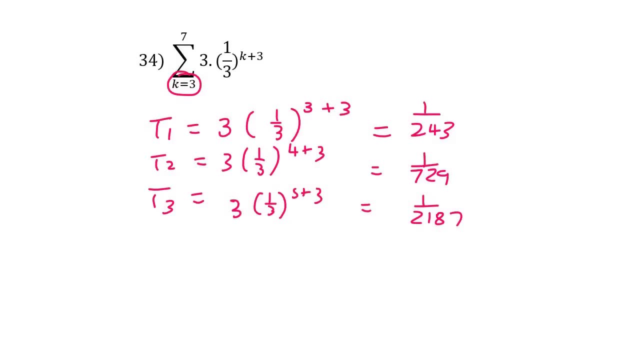 And that's 1 over 2187.. So we need to try to figure out: is this arithmetic or geometric? Now, for it to be arithmetic, the difference must stay constant. So you could test out what is term 2 minus term 1?. 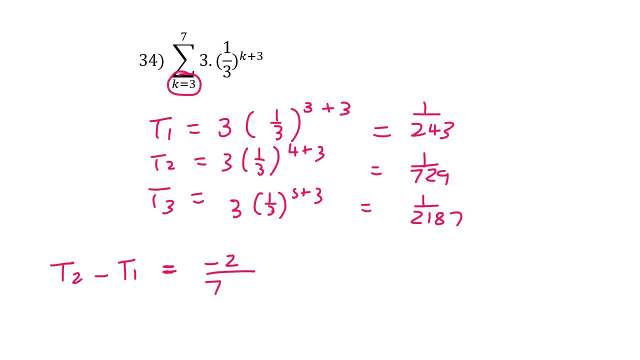 Well, if you go work that out, it's negative: 2 over 729.. Right now we go to t3 minus t2. And we're going to see if this stays constant. So it's going to be 1 over 2187. 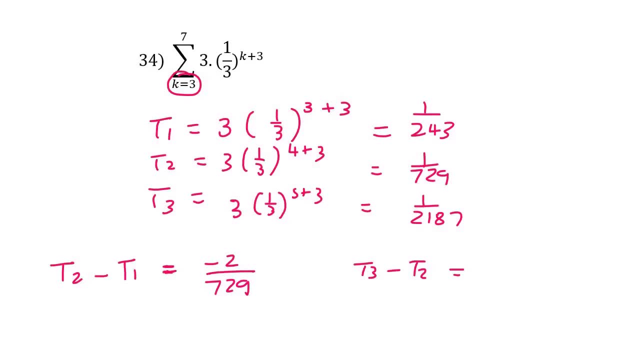 minus 1 over 729.. And no, it's not constant. You can see that we get a different answer. So these two are not the same, So the difference is not staying the same. Okay, so then possibly it could be a geometric. 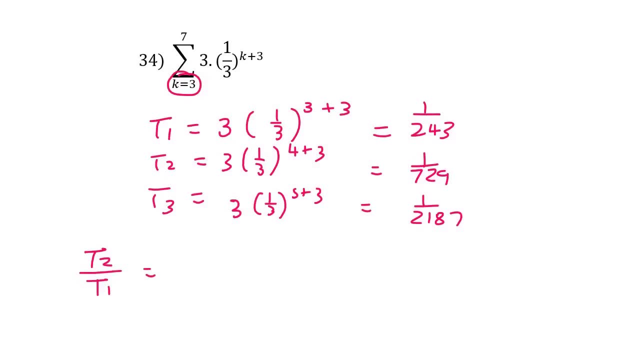 For it to be a geometric, we'd have to look at t2 divided by t1. And let's see what we get there. A third: If you got a different answer to me, it's because you're typing it in on the calculator. 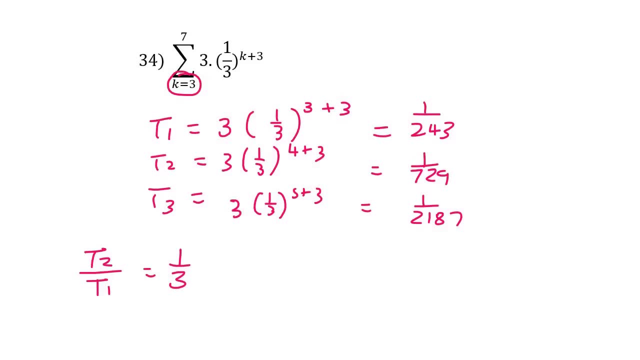 in a weird way. The Casio calculators can be a bit funny when you're dividing fractions, So just look out for that. If we look at t3 divided by t2, it's also a third. Okay, so it's a geometric sequence. 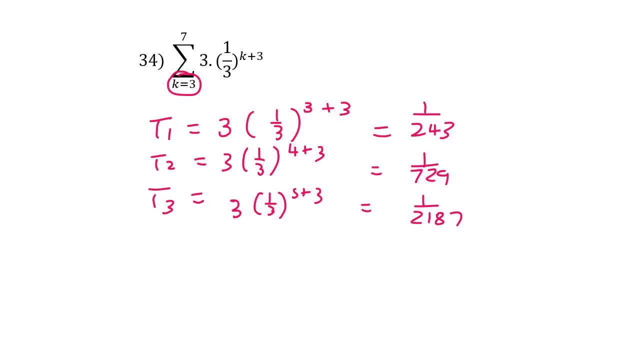 because the ratio is staying constant. So now we know that the sigma notation symbol means the sum of, So we need to go get the sum of formula for a geometric pattern, And so we're looking for the sum of a certain number of terms. 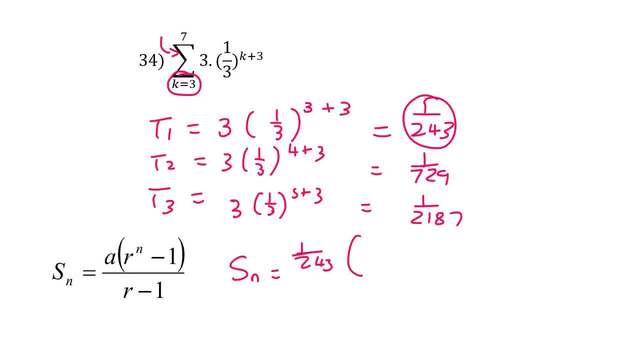 Now a is term 1, so that's 1 over 2.. And then r, we said was a third. The number of terms is not 7.. You've got to be careful. Remember how we've kept repeating in previous questions. 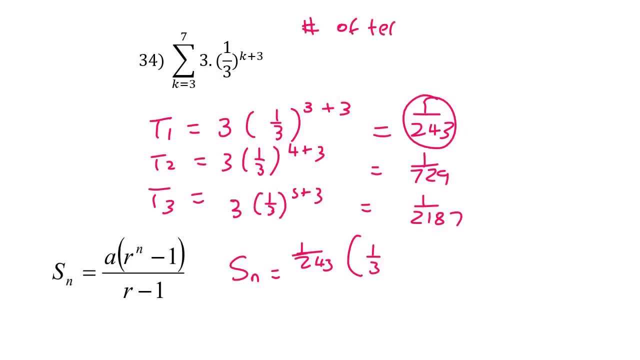 that the number of terms is the top number minus the bottom number plus 1.. So that's actually going to be 5.. So there are only 5 terms. What that means is you could theoretically go calculate t4 and t5 and then you could just plus. 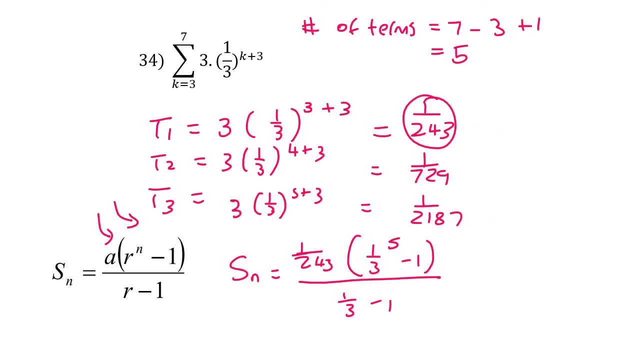 all of these numbers together, It will give you the same answer. And so to two decimal places. this should give us 6 point. It's not a very nice answer: 6.147.. Oh no, let's go to 6.15. 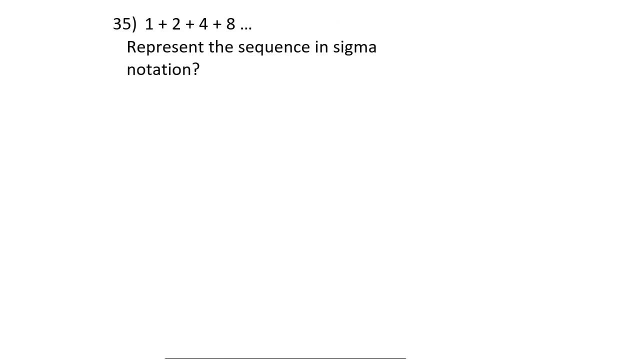 times 10 to the negative 3.. If you are asked to represent something in sigma notation, then what you do is you just put the sigma symbol. You put k equals to 1 down here, If you know how many terms there are. 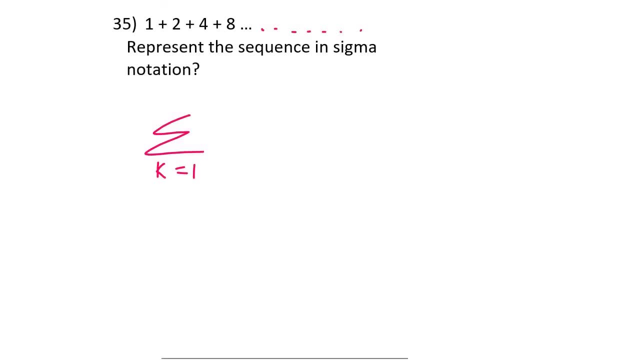 then you could put that number up here. But if they just give you something like this, then you just put an n over there. What you now need to do is work out whether this is arithmetic or geometric. Well, it's 1,, 2,, 4, and 8.. 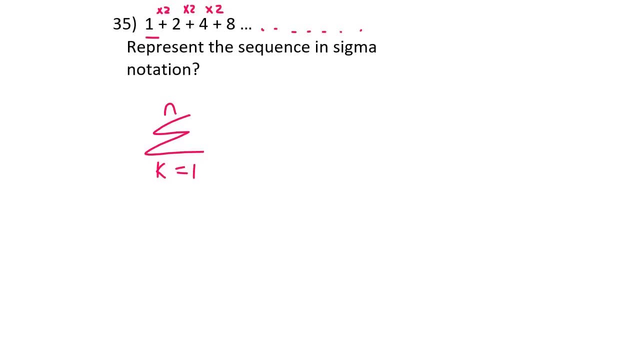 So it's definitely geometric where they are multiplying by 2.. So what you do now is you get the tn formula of a geometric sequence, And so a would be term 1, which is a, 1.. R is 2. And then n is 2.. 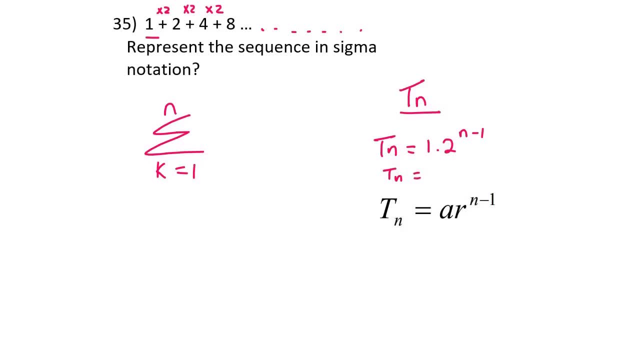 And so a would be term 1, and then n minus 1.. So this 1 over here doesn't even need to be there, because that doesn't really do anything, So it's just 2n minus 1.. You then take this tn. 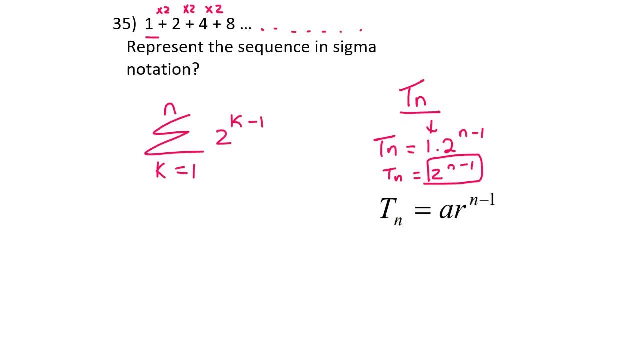 and you put it over here, But don't write it as an n, Rather leave it as a k. The reason is is that these two always need to match, And that is it. That's how you represent something in sigma notation. 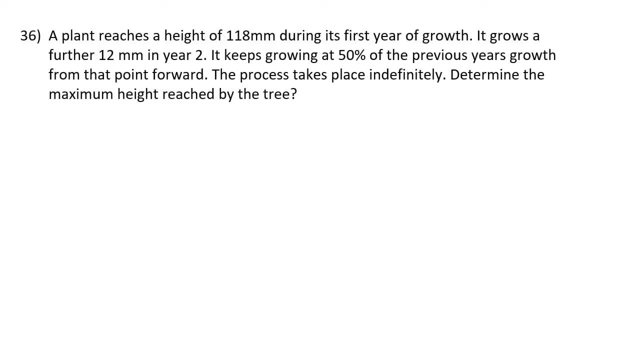 We are told that in the first year this plant grows 118 millimeters. So year one, 118 millimeters In year two. oh and by the way, if you've watched my previous questions on trees and things growing, you would see that we never look. 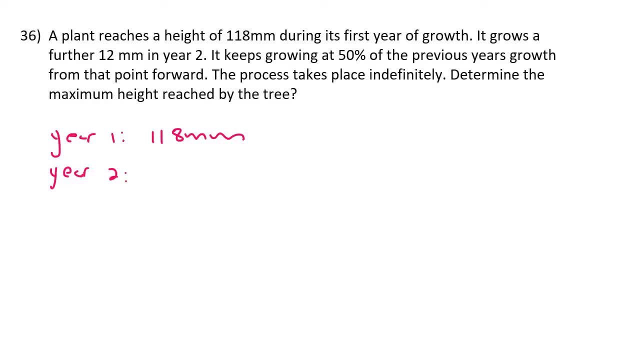 at the total height of the tree. We rather look at how much does the tree grow each year. That's where the ratio will be found. In the second year it grows 12 millimeters. Notice how I don't add these two together. 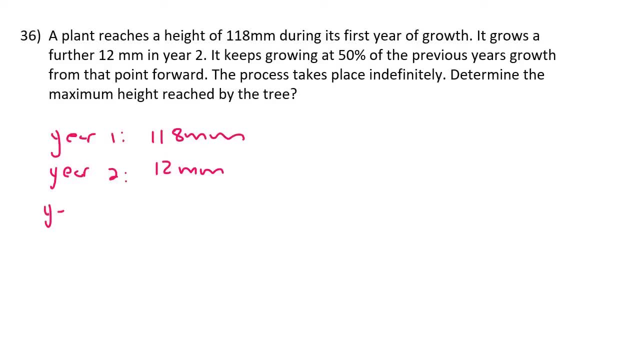 because I want to see how much it grows each year. Then for year three, they say it keeps growing at 50% of the previous year's growth. So it'll be 50% of 12, so 50% times by 12, which is 6.. 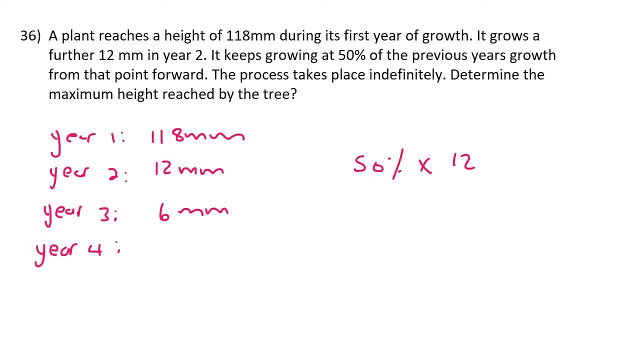 Then for year four, it'll be 50% of 6 now, which would be 3.. And this would just carry on, and on, and on and on. Do you guys remember the one question we did? I can't remember which question it was or which number it was. 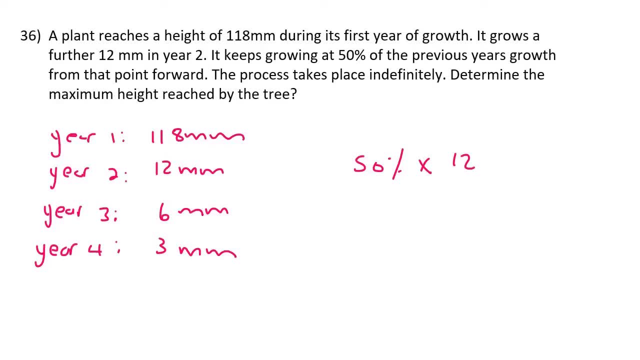 but I'm going to try to remember- OK, OK, OK- where we had to be careful because the ratio from the beginning was not constant. I'll prove that to you If we look at the ratio from 12 or 12 and 118,. 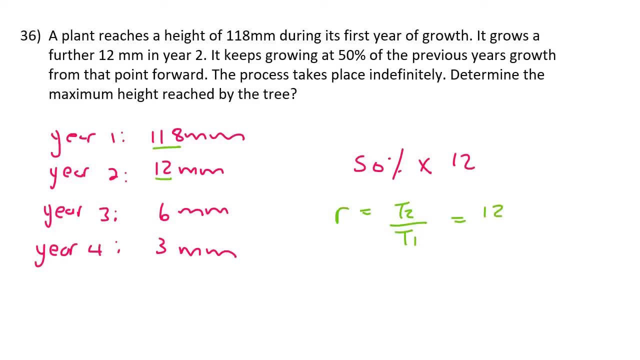 you would go term 2 divided by term 1,, which is 12 over 118,, 6 over 59. Then if we use term 3 divided by term 2, that would be 6 over 12,, which is a half. 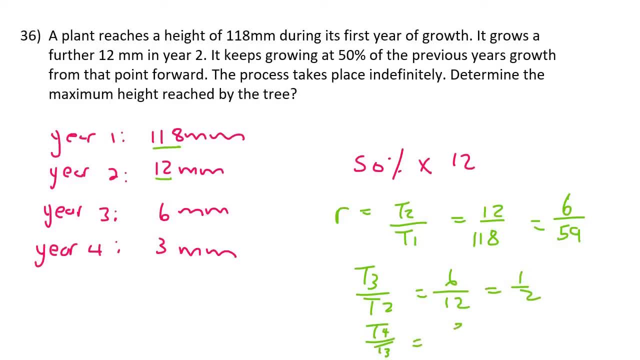 And if we go term 4 over term 3, that would be 3 over 6, which is a half, You see. so from this point onwards, the ratio is a half. Can you guys remember how we handled this type of question the last time? 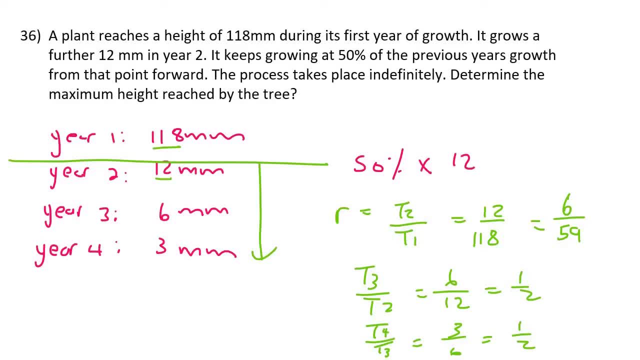 Well, what we do when this happens, when the ratio is not constant or when the first number is a little bit out of place, you ignore the first number, You just ignore it And we use the sum to infinity, because we don't know how many years. 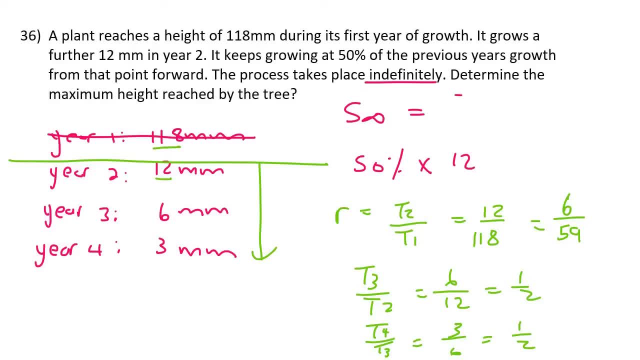 The tree is going to grow, for It says it takes place indefinitely. Now A is going to be 12 because we're not using this one, So it's going to be 12 over 1 minus. Now the ratio is a half. 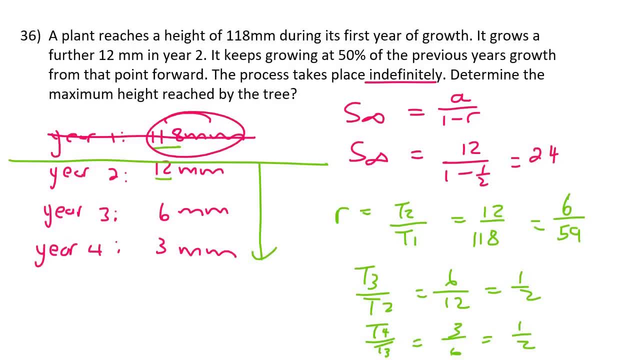 And so this is going to give us 24.. And then what we must remember is that, or what this means, is that from year 2 up until the tree stops growing, it'll grow a total Of 24 millimeters. okay, because 12 plus 6 plus 3.. 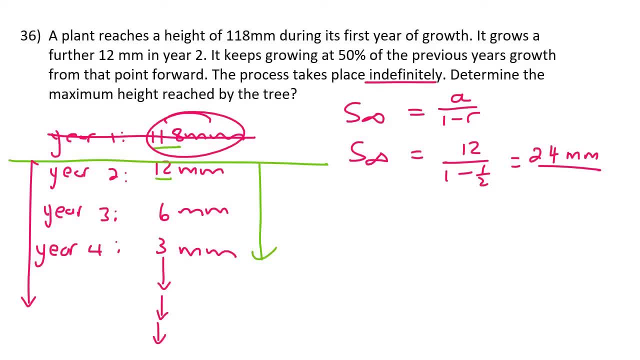 And then these numbers are just getting smaller and smaller and smaller And eventually they will reach zero. So it grows 24 millimeters, But then we need to remember that in year one it was already 118 millimeters. So the maximum 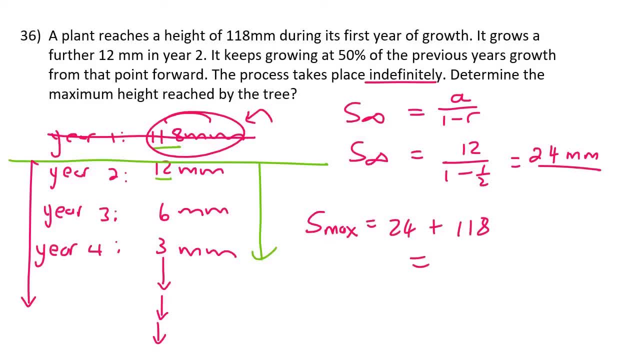 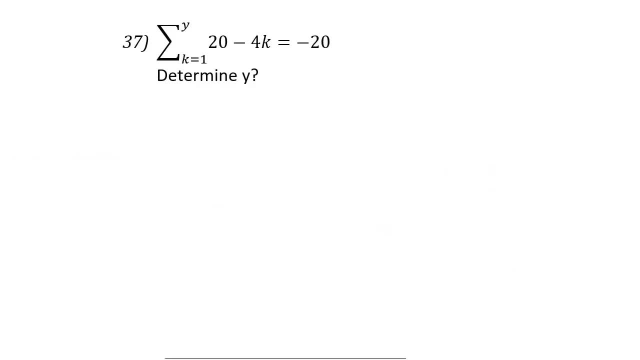 Will be 24 plus 118. And so it will reach a maximum height of 142 millimeters. It's usually A good idea to start Sigma notation questions by finding term one, term two and term three. to find term one, you plug in whatever this number is. 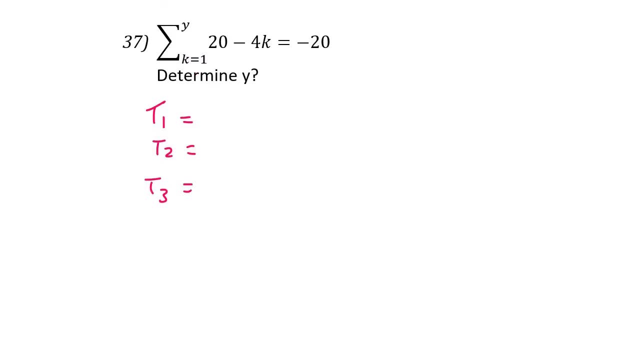 which in this case is also a one. That's just a coincidence. And so that's going to be 20 minus four times one, which is 16.. Then it's going to be 20 minus four times two, which is 12, and then 20 minus four times three. 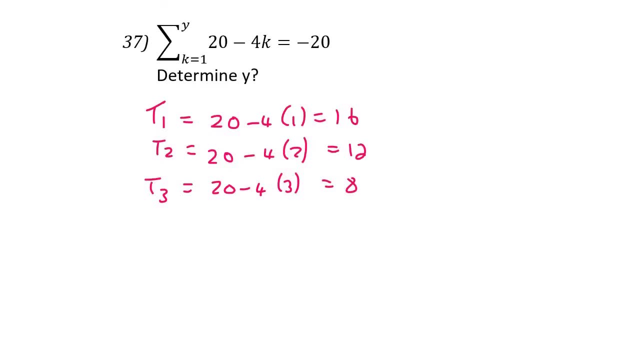 which is eight. So it's definitely arithmetic where the common difference is minus four. Be careful there. It's not four, It's minus four. Now they telling us. well, they are telling us that the sum is equal to minus 20, and we know it's. 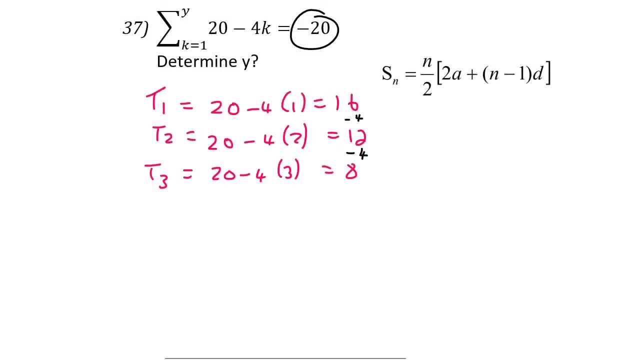 arithmetic, So then we can fill in the sum as minus 20.. I'm using this formula now and we don't know, So we go in over two and then two times a. a was first term, which is 16, and then N minus one. 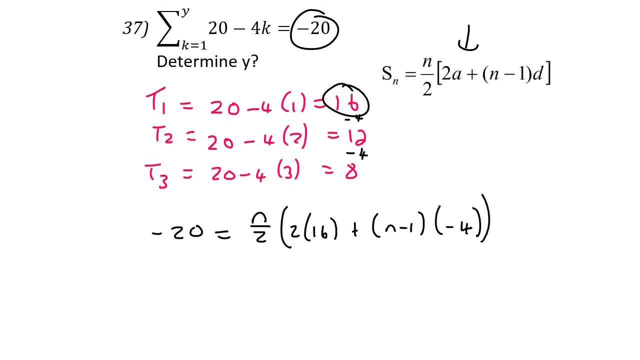 And then the common difference is negative four. Just remember that. then what I like to do here is I: I take this two and I multiply it over, So that's negative 40 equals to N. then inside these brackets it'll become 32 minus four, N plus four. 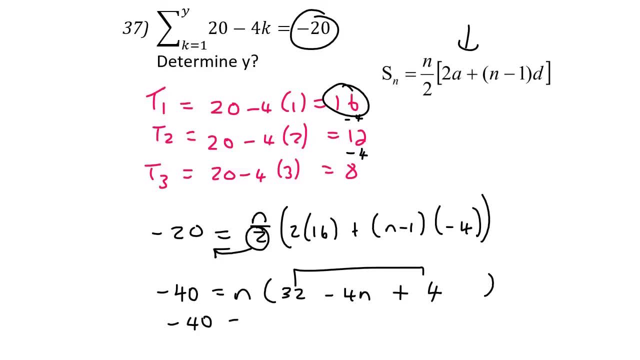 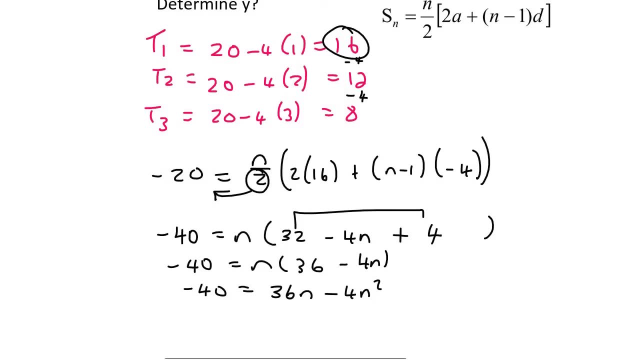 I then put the 32 and the four together, which would be 36.. Then I just multiply the N into the brackets, a trinomial by. I mean, you can do this however you want. I'm actually, I'm actually going to take everything to the left. 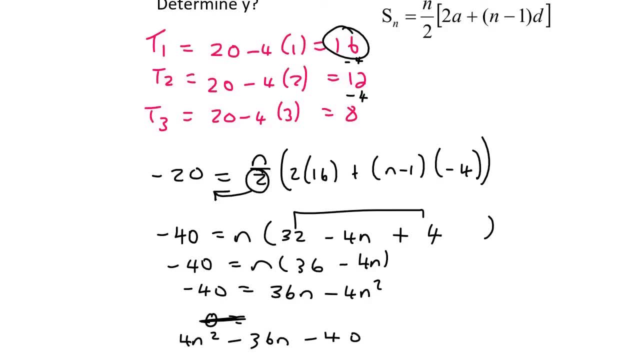 So that's going to be four N squared minus 36. N minus 40 equals to zero. Oh, I would just use the quadratic formula here. You can try factorize if you want, but I just like to use the formula. And so what we find is that N is 10 or N is minus one. 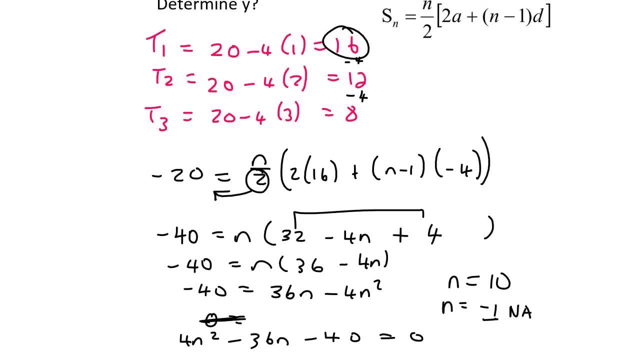 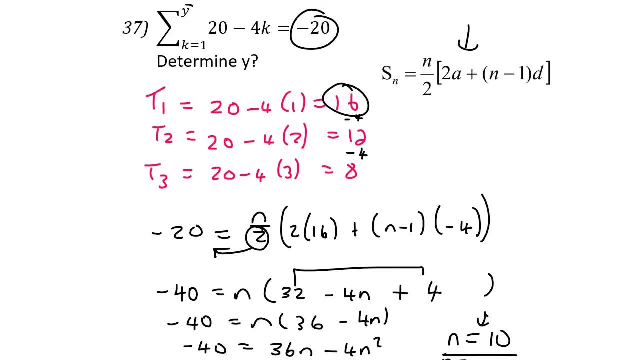 Now you can't have a negative position, so this will be no solution. Now be careful. N is your number of terms. that won't always be the same as this number over here, to make sure you always have to remember that This number, or the number of terms, is equal to the top number. 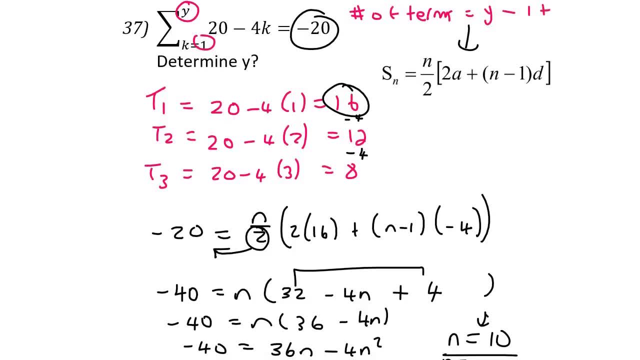 which is Y minus the bottom number, which is a one plus one. So in this case it won't always be like this: The number of terms, which is 10, is going to be the same as Y, because these cancel out. But if this number at the bottom was a two or any other number, 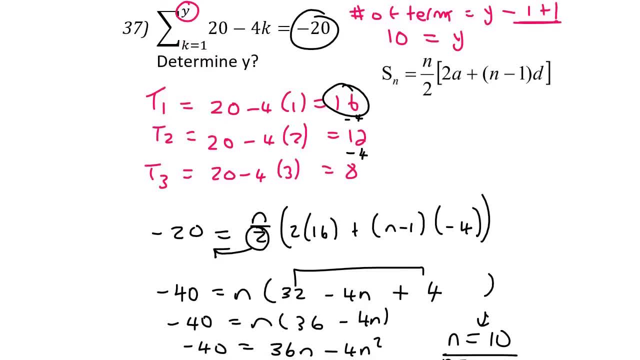 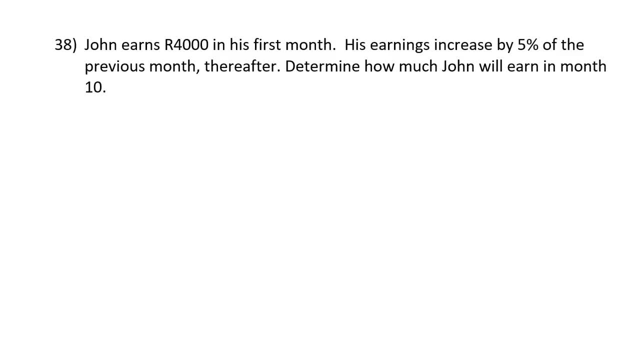 then you would have to be very careful, But for this one Y will be 10.. John earns 4000 rand during his first month, and then his earnings increased by 5% of the previous month thereafter. So what that means is that in 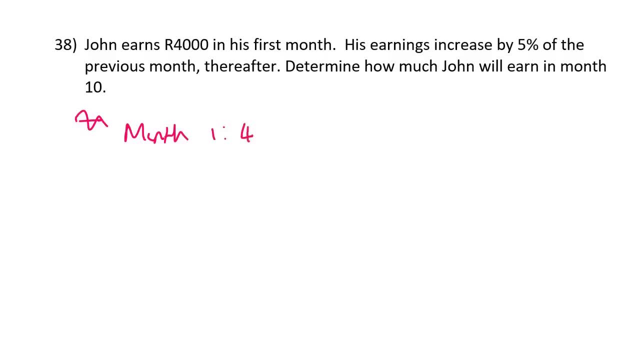 let's say month one he earns 4000.. Then in month two you have to add 5%. So you first work out what 5%. I mean, there's different ways of doing this, but you could work out 5% of 4000.. 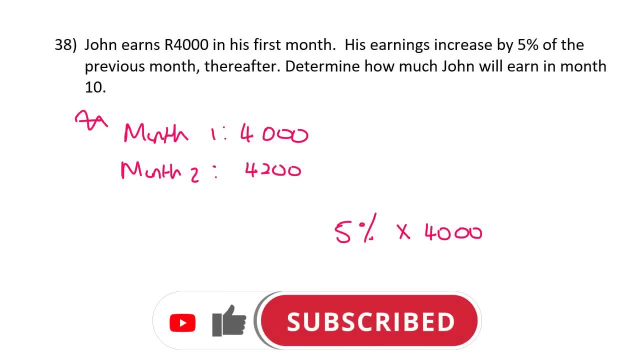 Then add that on, So then he earns 4200.. But now he's going to earn an extra 5% in month three of 4200, and that's 210 rand. So you add it on And so he earns 4410, 4410. 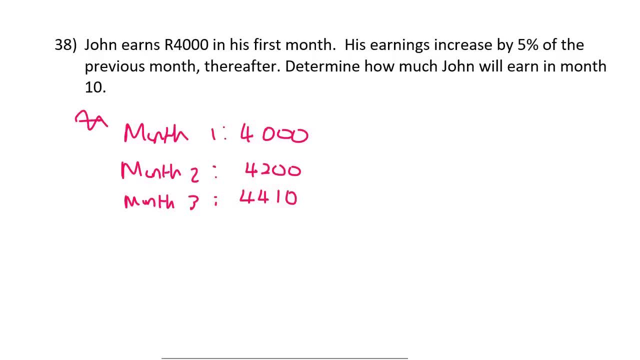 Now, those first three terms are enough to tell us whether we have an arithmetic or geometric. for it to be a geometric, term Two divided by term one would have to be the same as term three divided by two. But we need to see if that is true. 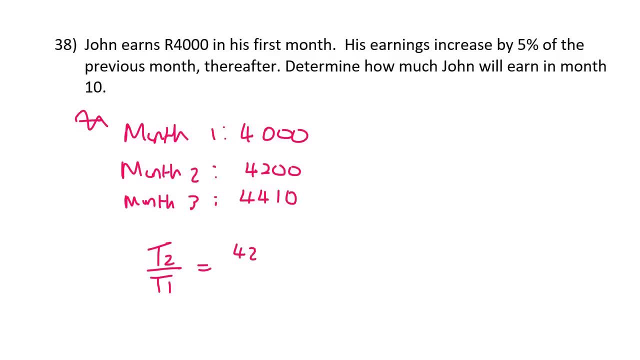 We can't say it's true. So let's check. We can say 4200 over 4000 and that's going to give us 1.05.. Now we need to check term three divided by term two, which will be 4410 divided by 4200.. 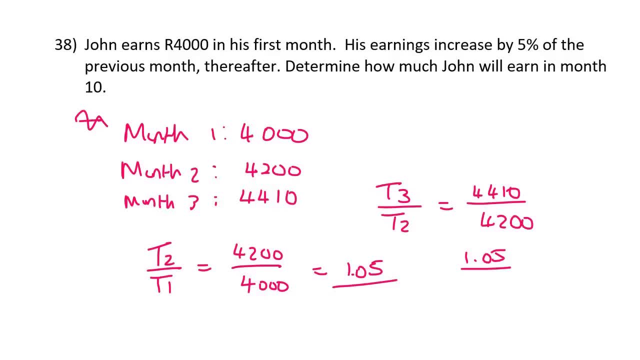 And that's also 1.05.. So it is geometric. They said: determine how much John will earn In month 10. guys are they asking us how much he's going to earn in month 10, or do they mean how much is he going to earn in total over 10 months? 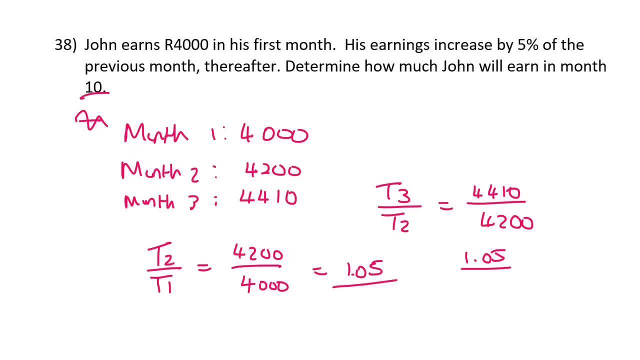 Well, well done, if you realize that they want to know only for month 10.. So we are not going to use the sum formula, because that would add up month one, month to month three, all the way up to month 10.. We're rather going to use the term formula of a geometric, because we're only looking for a specific term. 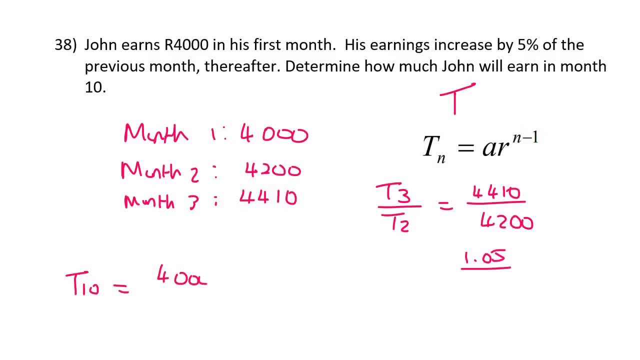 So we're looking for term 10. now a is 4000, the ratio is 1.05, and then n is 10 minus one. So then you can go type all of that in and that's going to be 6205 rand and 31 cents. 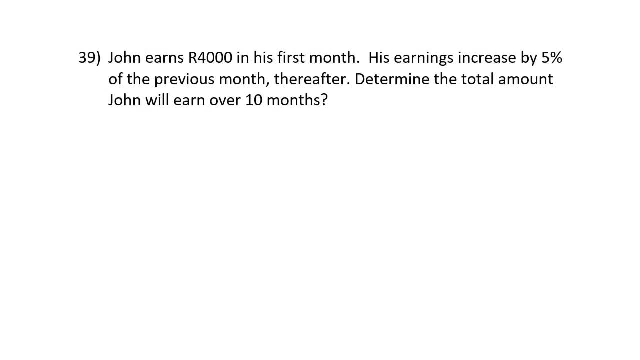 This question is almost identical to the previous question, So I'm going to- I'm going to assume that you've already watched that. if you haven't, maybe you should just go watch that quickly. But all that they change is, they say: determine the. 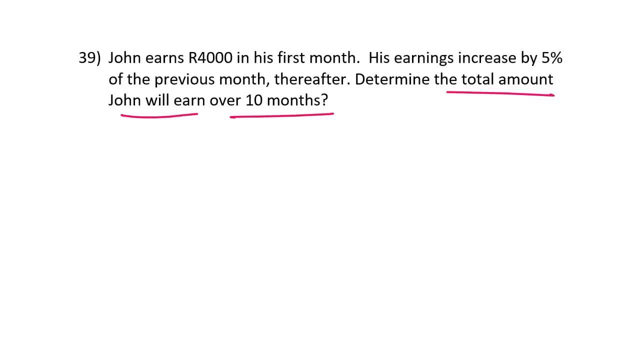 Total amount John will earn over 10 months. So they're not saying how much is he going to earn in month 10?. They want to know how much will you earn all together during the first 10 months. So that's like term one plus term two plus term three plus all the way up to term 10.. 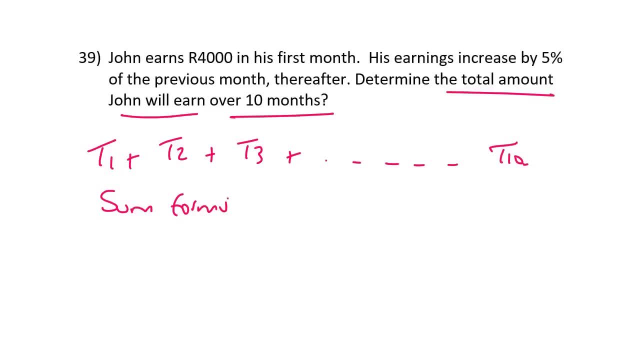 This is why we use the sum formula. that does that for us. We saw in question 38 that it's a geometric sequence with a ratio of 1.05.. So we use the sum formula now because we're trying to find the total over 10 months. 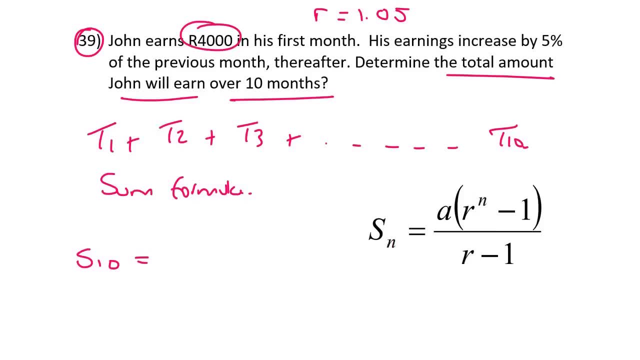 And so that's just going to give us a, which is the first term, which is 4000.. We said the ratio from question 38 was 1.05 over 10 months And then minus one, And so in 10 months, 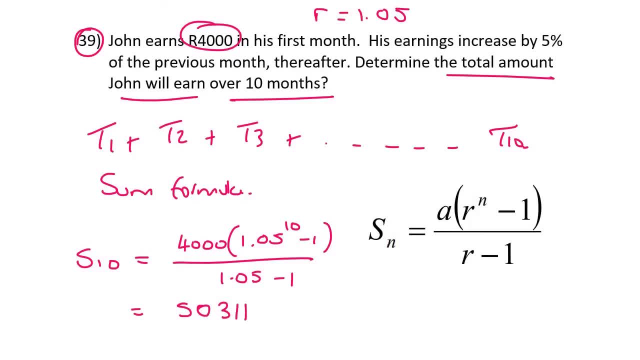 John is going to earn a total of 50,311 rand and 57 cents. I mean, this makes sense. Think about it. He earns 4000 rand in his first month and then a little bit more in month 10.. So if he only earned 4000 rand every month, 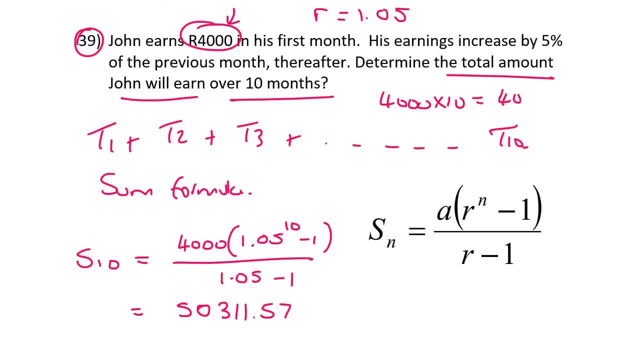 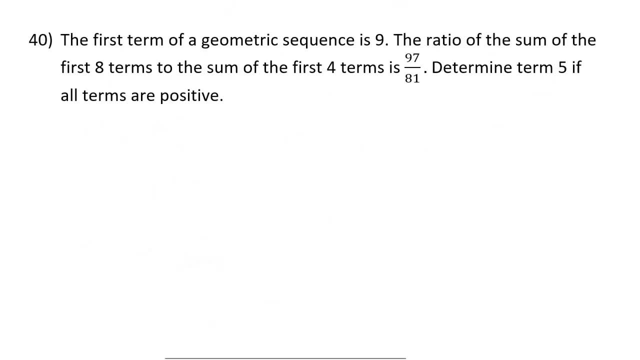 then 4000 times by 10, he would have earned 40,000.. But because they're giving him a slight increase, he's able to get his money up to about 50,000.. All right, question 40. They tell us that the first term of a geometric sequence is nine. 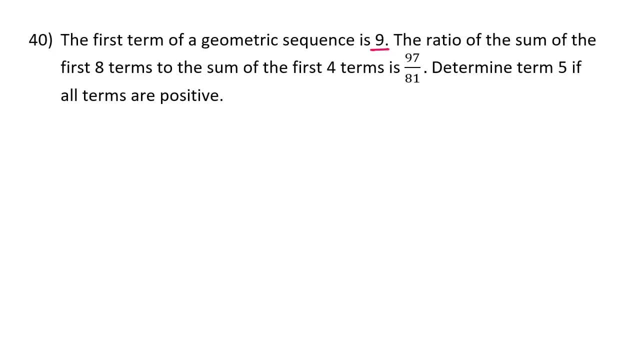 And then this one's quite interesting: The ratio of the Of the first eight terms to the sum of the first four terms is that determine term five if all terms are positive. So this is quite an interesting one. Okay, Well, they tell us that the first term is nine. 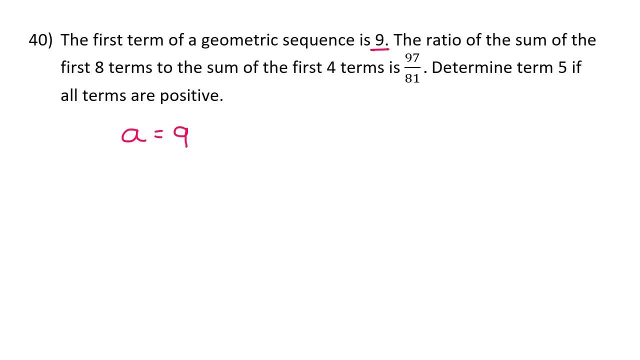 So we know that a is nine. Then they tell us that the ratio of the sum of the first eight terms. Let's find the sum of the first eight terms. We know that it's geometric and we know that a is nine, So we can say nine. 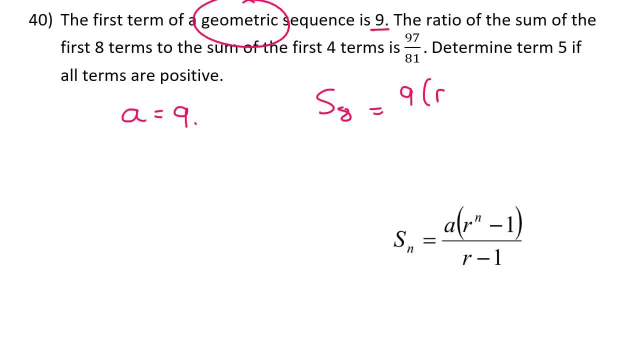 but we have no idea what the ratio is. And it says that the sum of the first eight terms- because that's eight minus one over R minus one, And then they also talk about the sum of the first four terms. So let's go full, that in. 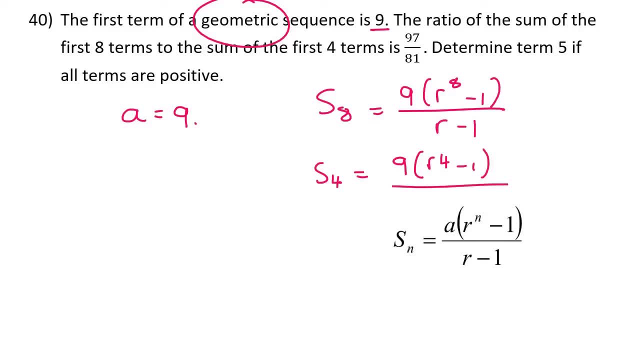 That's also going to be nine, Then it's going to be R four minus one Over R minus one. They tell us that the ratio of the eighth sum, which is this one, to the fourth one, is 97 over 81. What that means. 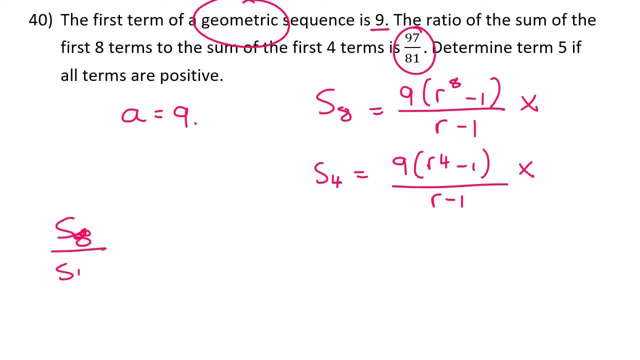 Mathematically is that S eight over S four is 97 over 81, which is going to be nine R eight minus one over R minus one over nine, R four minus one over R minus one. Okay Now, what I think we should do next is here: 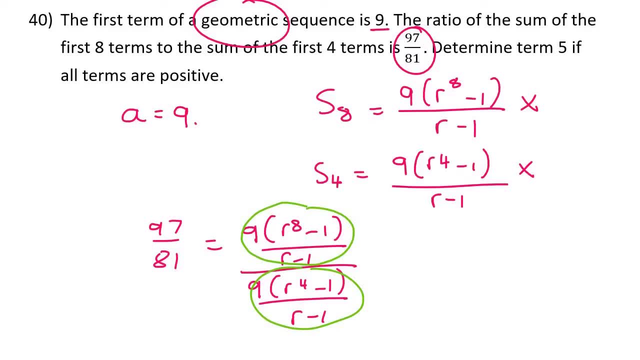 We have a fraction on top of a fraction. So you know, like in earlier grades, where if you have like one over four divided by three over two, then you can do that timesing and the flipping over things, So it becomes one over four times two over three. 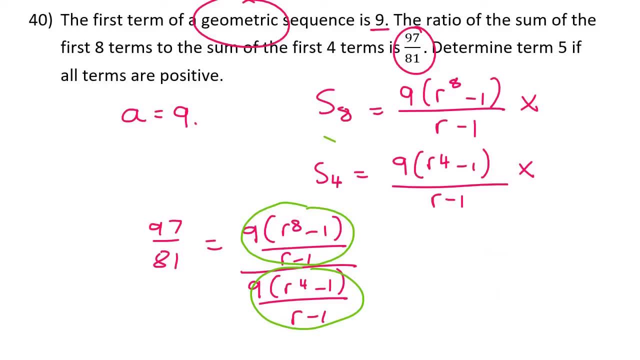 Well, let's try that now. I think some things might cancel out. So it's going to be 97 over 81 equals to nine, and then R eight minus one over R minus one. times by R minus one over nine: R four minus one. 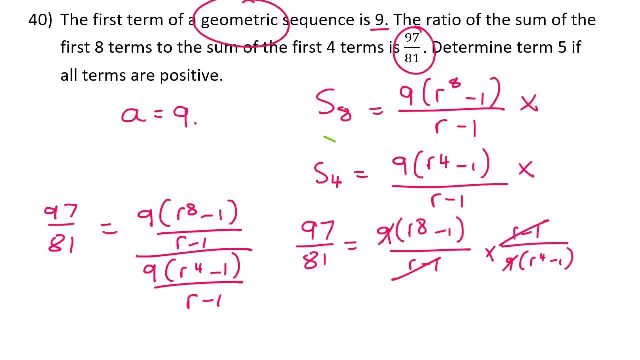 Okay, so those cancel, That's quite nice. The nines also cancel out, And so we left with 97. over 81 equals to R eight minus one, R four minus one. Now we could think of the top one, This one, here as a difference of squares. 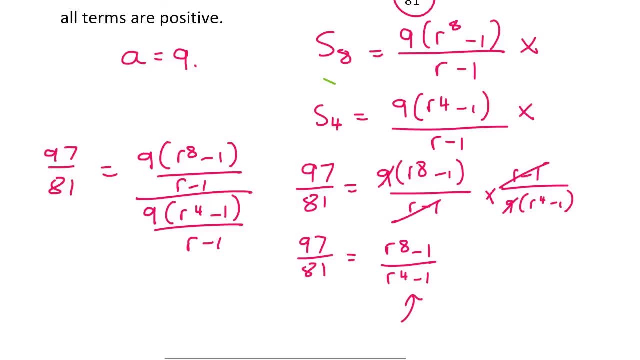 We could also do difference of squares with the bottom one, but it's not necessary. Let me show you why. if we do difference of squares with the top one, we're going to get 97 over 81 is equal to R four minus one and R four plus one. 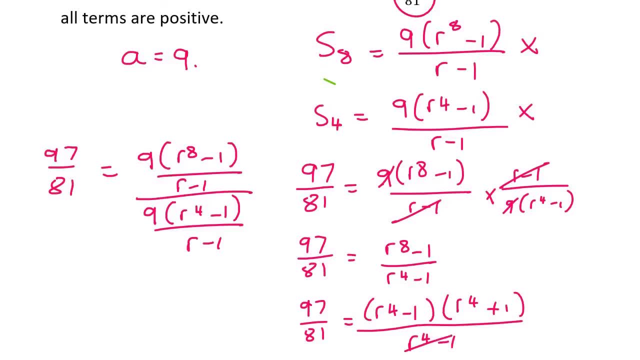 That's difference of squares. Then we have R four minus one here. Those cancel. Oh, it's working out nicely. I was a bit concerned just now. So 97 over 81 is equal to R four plus one. We then take the one over. 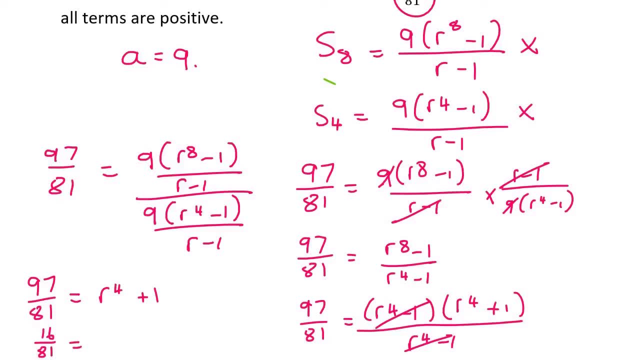 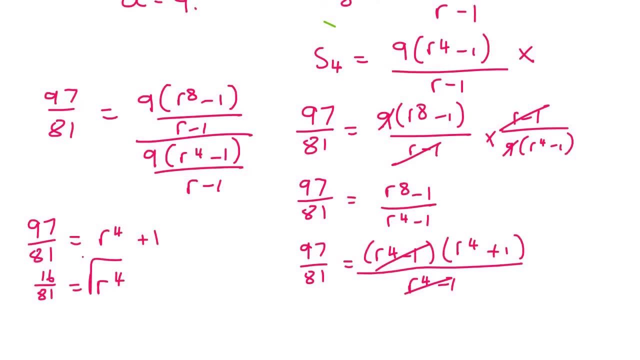 Oh, it's working on very nicely. So 16 over 81 is equal to R four. We can take the fourth root, so we can take the fourth root on both sides, And so R is going to be two over three Technically. 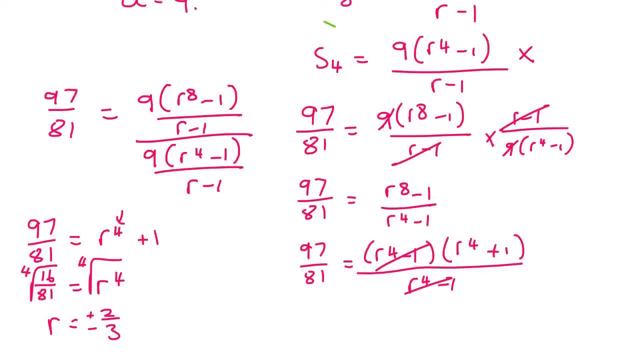 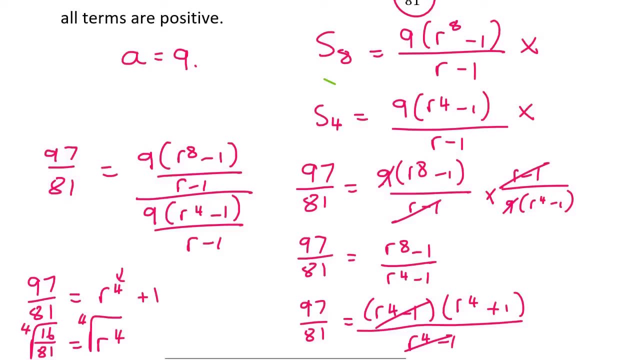 when you take in a root of a positive number, you should have a plus and a minus, But it's only going to be the positive one because they've told us that all terms are positive. So if my R value is negative, two over three. 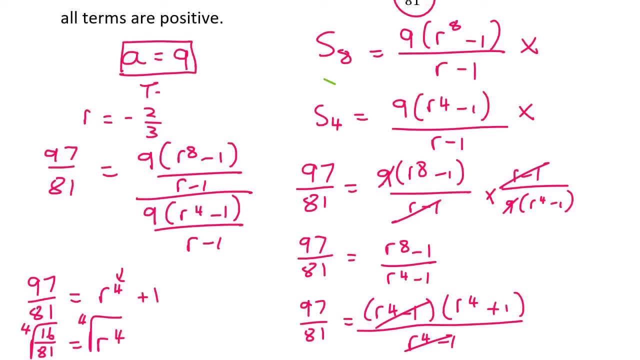 then if a, which is term one, is nine, then term two would be nine times negative, two over three, And so we would start including negative numbers, And so that's not going to be correct. So therefore, R is only going to be positive. 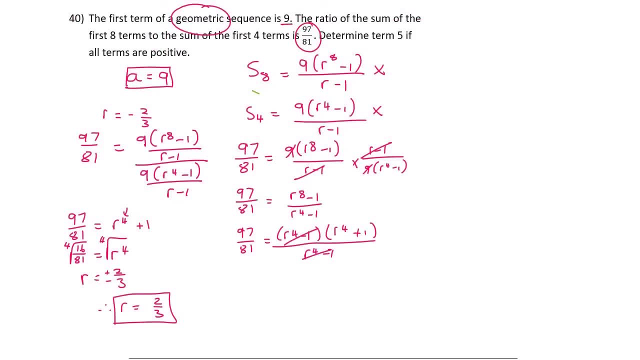 Two over three. But now we're not done because they said: determine term five. So to determine term five we can use the TN formula and we try to find term five. Now a, they told us, is nine R We just found as positive two over three to the power of five minus one. 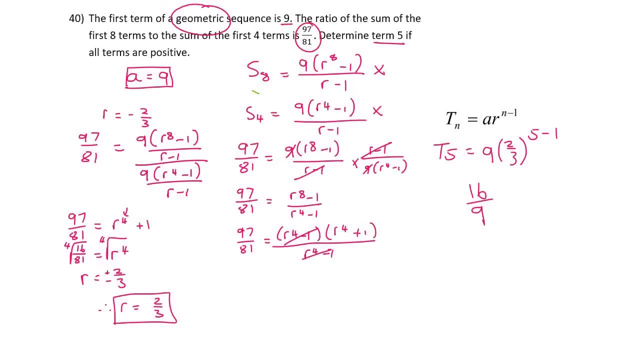 And that's going to be 16 over nine. Now, of course, you could leave it as 16 over nine or you could write it as A decimal 1.78.. If it wasn't a test, you would most likely do two decimal places. 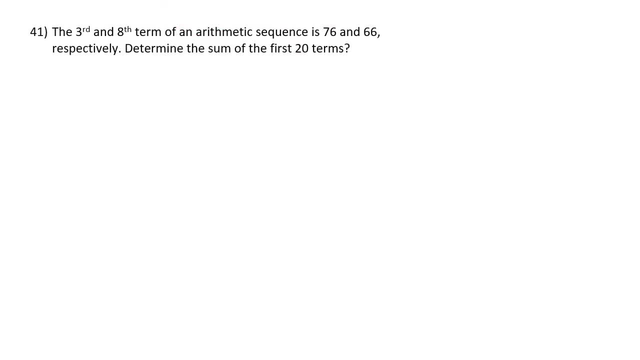 For question 41,. they said that the third and eighth term of an arithmetic sequence is 76 and 66 respectively. Determine the sum of the first 20 terms. All right, so they're trying to tell us that term three is 76.. 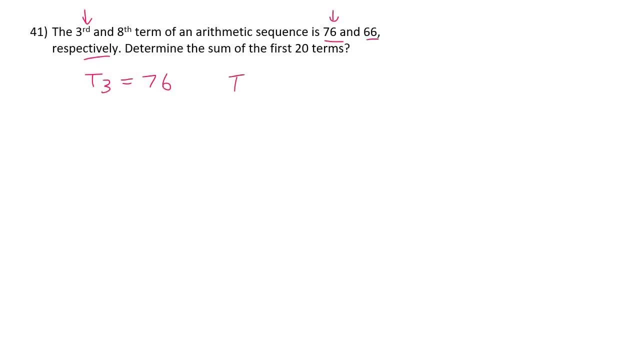 So we could say T3 is 76 and term eight is 66.. All right, so it's an arithmetic sequence, So I'm going to use this one over here first. So we're going to say 76.. Actually, let me make this a little bit neater. 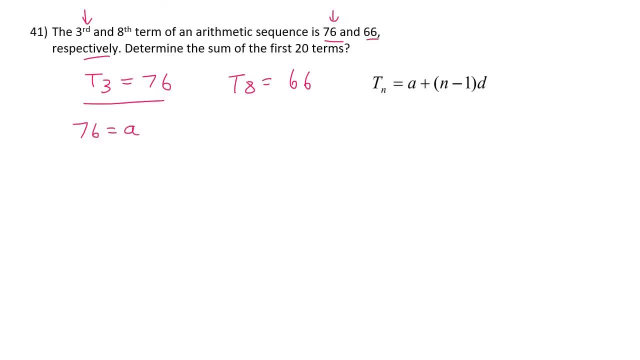 Let's put it over here. So we say 76 equals to a plus Now, that's term three. So we do that times D, which we don't know. So 76 is equal to a plus two D. Then I'm going to use this one over here. 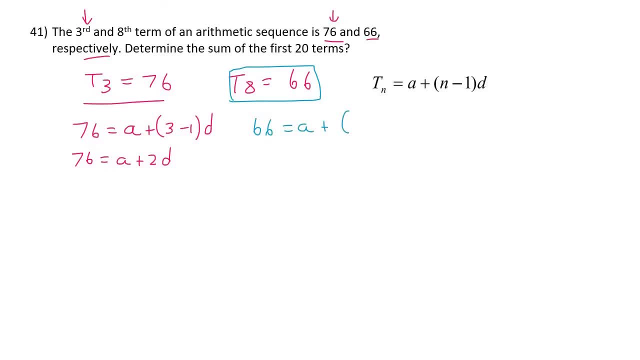 And so that's going to be. 66 equals to a plus eight minus one times D, And so 66 is equal To a plus 70.. All right, so now we just link these simultaneously, So I'm going to get this one by itself. 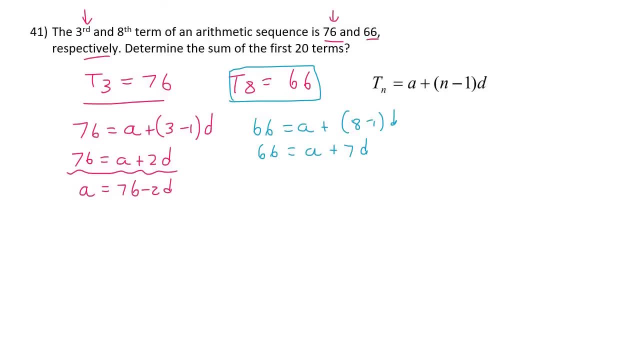 So that'll be a equals to 76 minus two D and I'm going to plug that a over here. So that's going to be 66 equals to, and then I plug that in a 76 minus two D Plus seven D, and then I can solve for D and that's going to eventually give us. 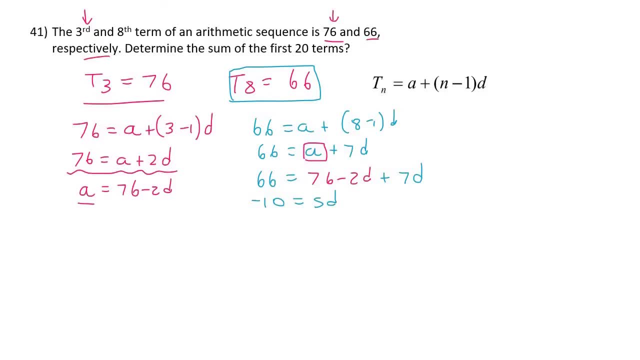 Minus 10 on the left equals to five D, and so D is negative two. Now I can plug that D value over here. So a would be 76 minus two in brackets, minus two, and so a would be 80.. Now they say: determine the sum of the first 20 terms. 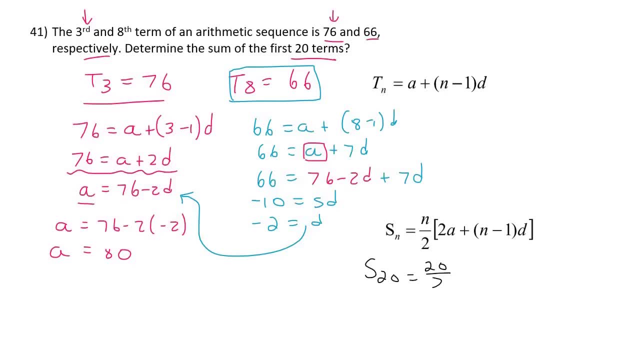 And so the sum of the first 20 terms, So n is 20.. A is What did we say? Oh, there we go. 80. now n is 20 and the common difference is negative two. That's going to give us a thousand two hundred and twenty. 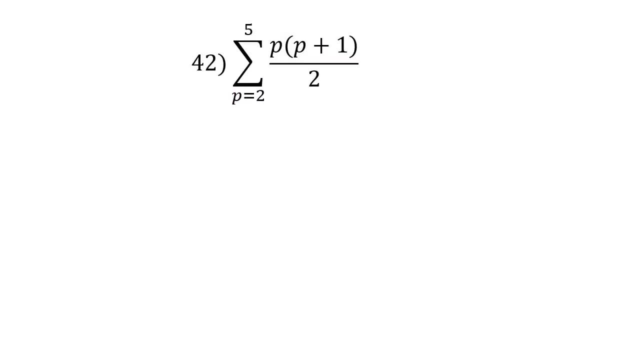 So whenever I give a question like this to my students, they often look at me and they're like: okay, So what is the question? Well, guys, we must always remember that this symbol stands for the sum, So they're asking you to calculate the sum. 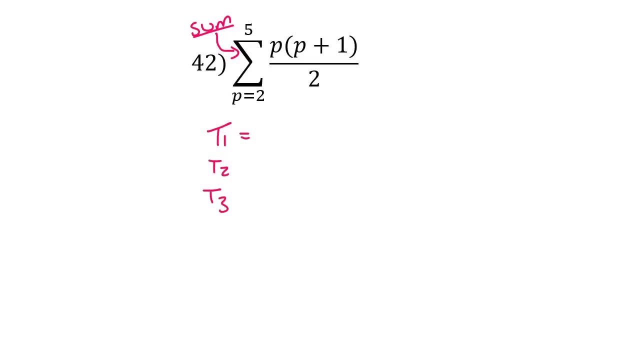 So what we usually do first is we find term one, term two and term three just to see if we have an arithmetic or Metric pattern. to find term one, you plug in whatever this number is in the place of P. So that's going to be. 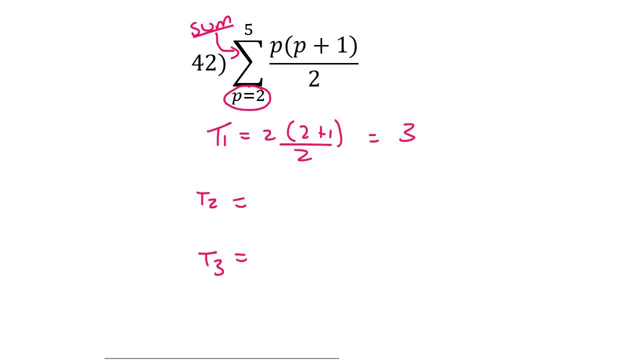 Like that, and that will give us three. and then to find term two, you just increase this number by one, So it'll be three times three plus one over two, Just six. and then to find term three, we increase it again, So it'll be four times four plus one over two. 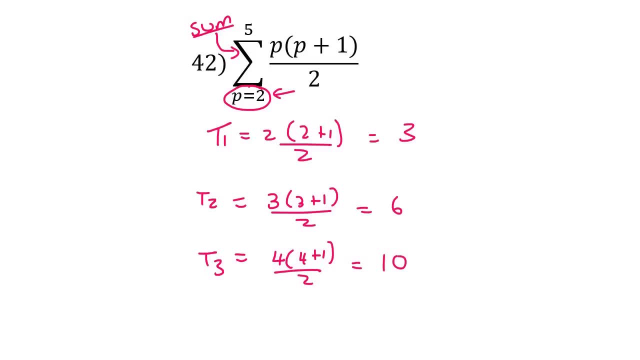 Which is 10.. Now, guys, what you are going to realize is that there is no pattern taking place. But if you watched one of the previous lessons In the sequence and series videos, can't remember which one it was. We realized that sometimes they will give us a question that doesn't have a pattern, but then they will usually make the number at the top really low. 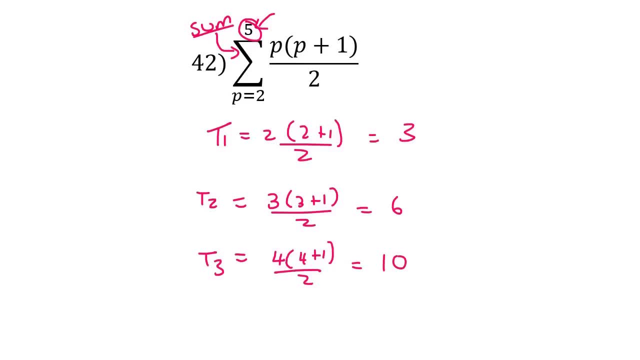 The reason for that is now we don't have a lot of terms, So we can go Find them ourselves. So how many terms are there? Remember, There's not five. The number of terms is the top number Minus the bottom number plus one, and so there's only four terms. 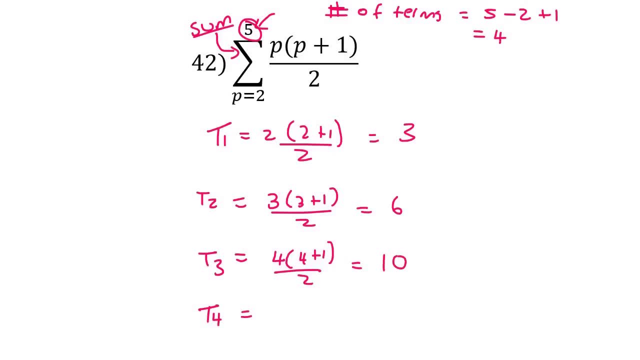 So we've already done the first three. We might as well just quickly go do the fourth one, Just 15.. Now what we do is we just add these numbers together And that gives us 34, and that's the answer. That is the sum. 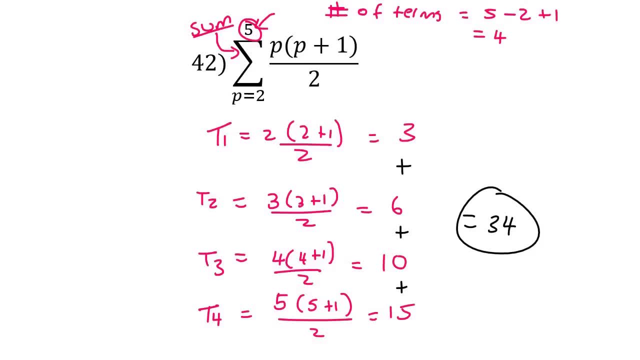 You can do it manually or you can do it yourself If they don't give you a proper kind of pattern. All right, with a question like number 43. All you do is the following: to find term five, You just need to add up the first five terms and then minus the first four terms. 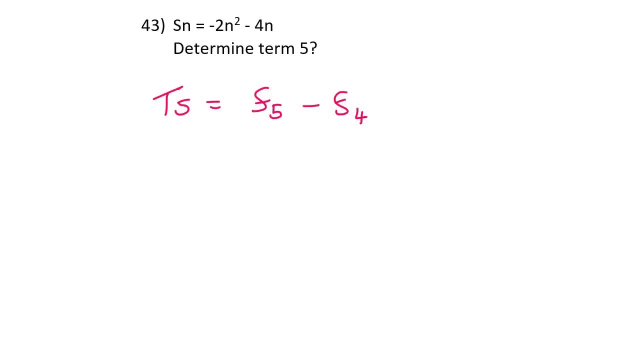 The sum of the first four terms. All right, And so to find s5.. You just plug five into the place of n, So that's going to be minus 25.. Notice, I'm always using a bracket when I plug it in. 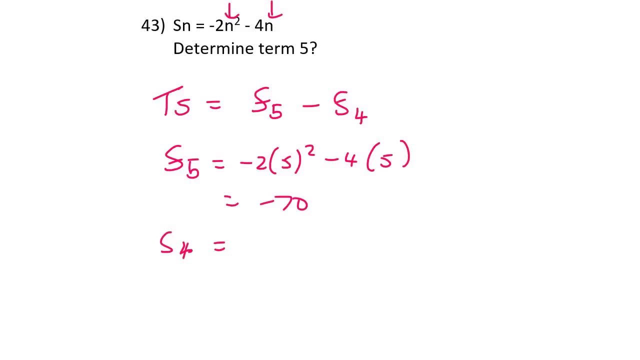 It'll be negative 70. then to find s4. You just plug in a four and that's negative 48. So to find term five, then you just say the sum of the first five terms minus The sum of the first four terms and that's going to be negative 70.. 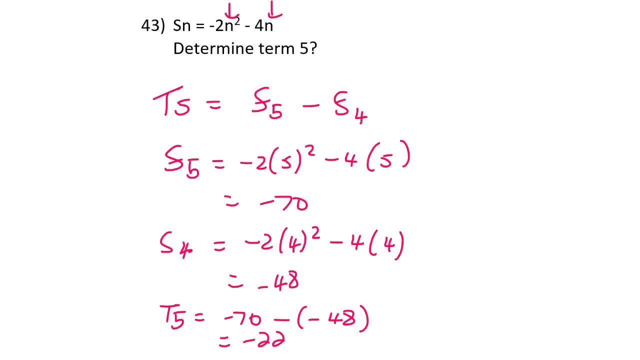 Plus 48 and that's going to be negative 22.. A sequence converges: when are the ratios between minus one and one? So we need to find R. So let's go find term one, term one. You start off by plugging whatever this number is into the place of P. 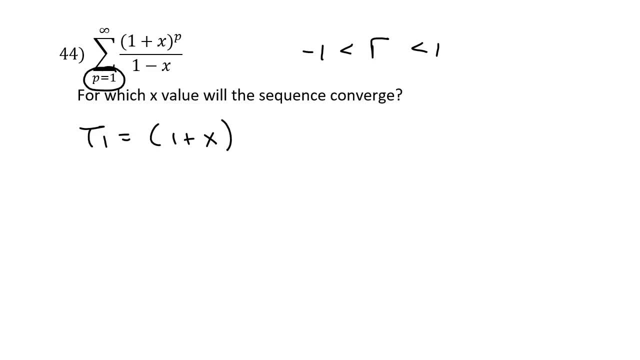 But, Kevin, what about X? Don't worry about that, guys, You'll see it all work out. So you just do that. then to find term two, You do the same thing. You plug in a two this time, because that's you always add one to this number. 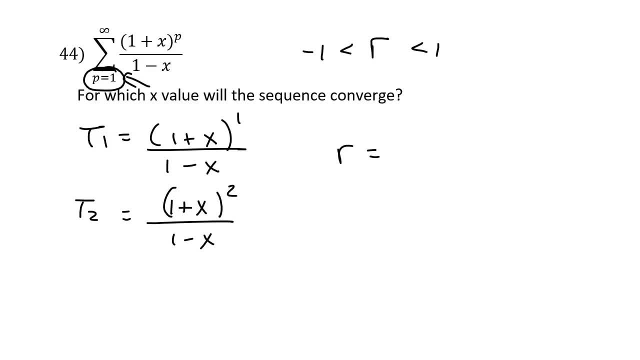 So that's going to look like that. now are for any geometric sequence. We know that it's geometric, because only geometric sequence Is converge. You could use term two divided by term one, and so that's going to be one plus X squared over one minus X, divided by one plus X over one minus X. 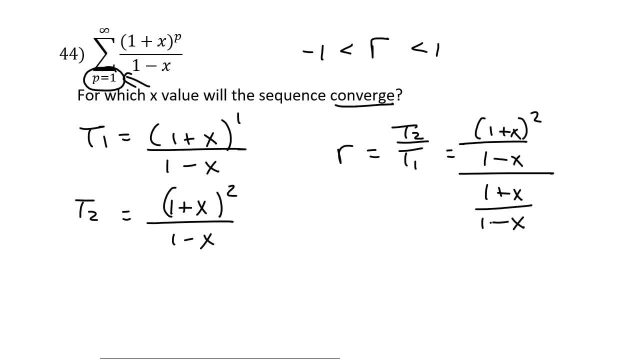 Now, whenever we have a fraction on top of a fraction, then we need to use a trick that we probably learned in earlier grades, Like if you have three over four divided by two of us nine, then you can say three over four times nine over two. 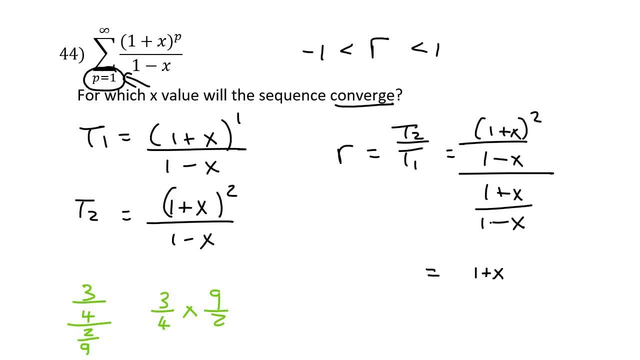 So we're going to do the Approach, and so that's going to be one plus X squared over one minus X, multiplied by one minus X over one plus X. So this cancels, and then this cancels with one of these. So you've just got one plus X left over. 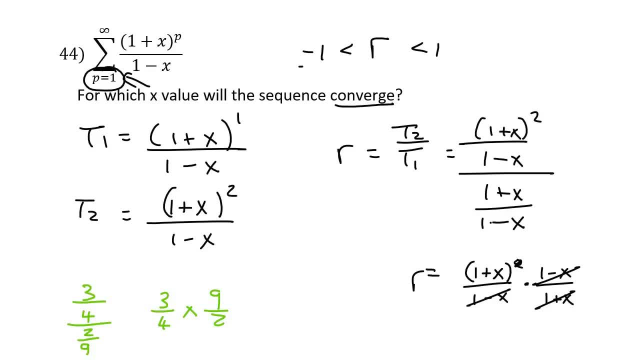 So R is one plus X. So what I then do is I go put that in the place of here. So I say one plus X must be between one and minus one, and so X is going to be zero If I take this plus one over to that side. 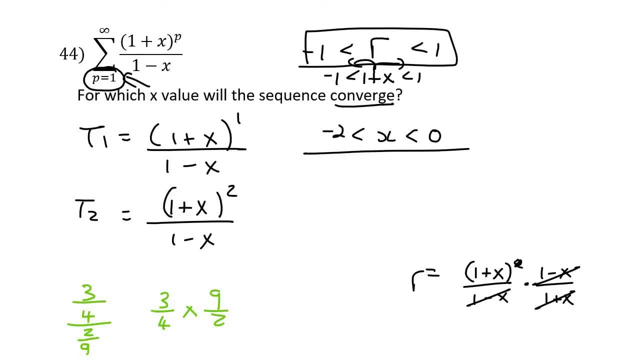 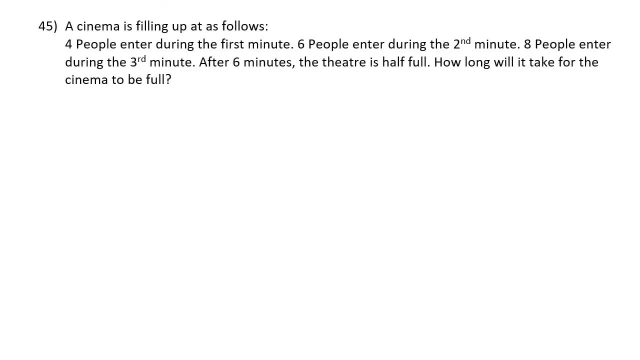 and if I take it to that side it's going to be negative. to question 45 is quite interesting. So we've got a cinema that is busy filling up because people are walking inside the cinema or walking into it. They say four people enter during the first minute. 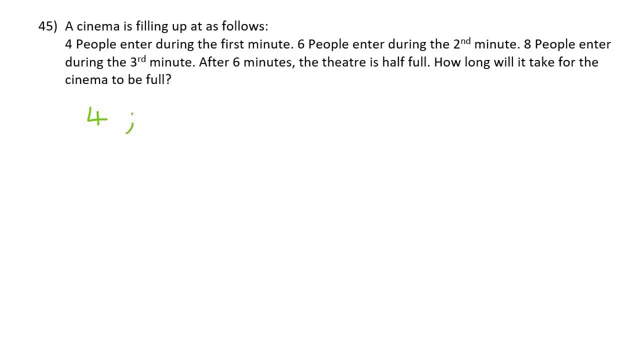 Okay, so four people enter during the first minute, six people enter during the second minute and eight people enter during the third minute. after six minutes, The theater is half Full. Okay, so we know that this is one minute. This is two minutes. 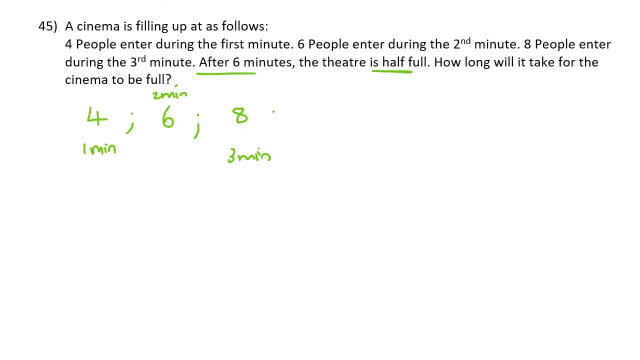 This is three minutes. We can clearly see an arithmetic pattern is taking place here, So we can actually just quickly fill it in. So six minutes would be here. All right, so check this out guys. How many people are they? Well, 14 people entered, but how many people have entered in total? 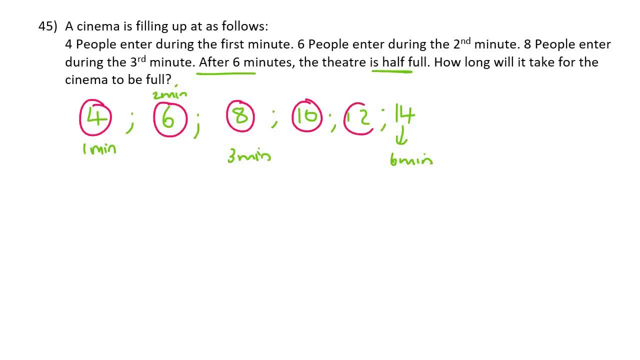 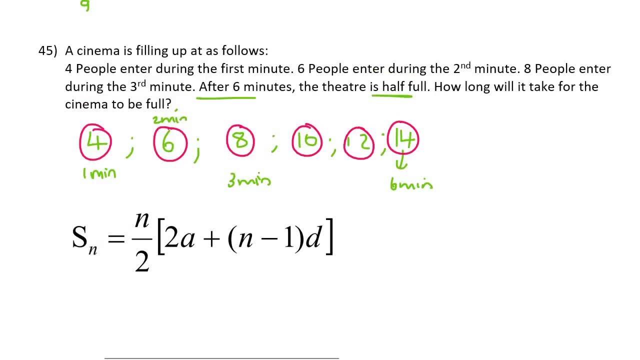 Well, you could go add these numbers together, or you could use the sum formula. I'm just going to be fancy and use the sum formula. So we know that there are six terms, so we can just find the sum of those first six, which is actually six minutes. 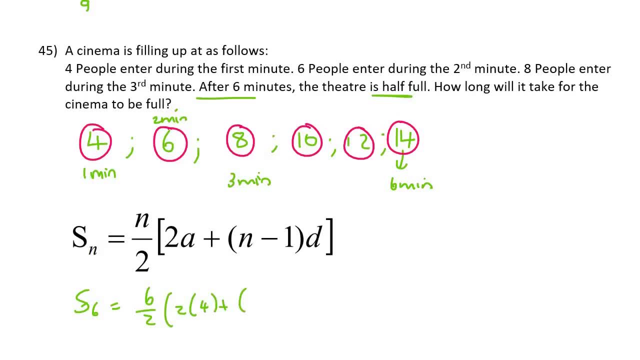 Now, a is your first term, which is four, And then the common difference is two. so we can go work that out And, as I said, you could have just added them yourself. It's probably faster, but I'm just being fancy, and that's 54.. 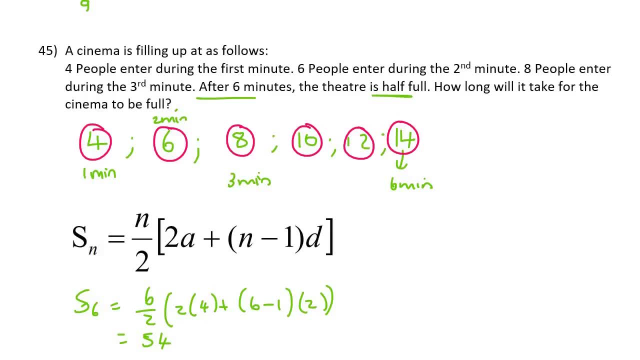 Okay, so there are 54 people who have entered During six minutes. They said that after six minutes the theater is half full, So then it means that this Cinema can hold a hundred and eight people, because it's double 54.. 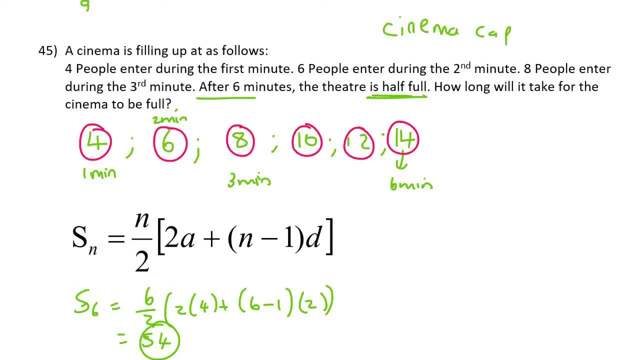 So let's say here, cinema capacity Is 108, so there can be a hundred and eight people in total. So it is: how long will it take for the cinema to be full? Well, we know that we need to get a hundred and eight. 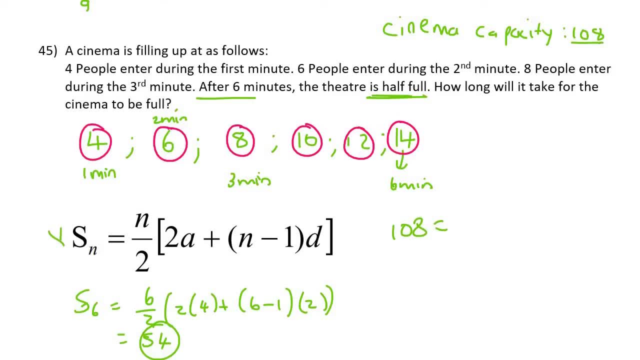 People in there all together. So I'm using this formula again, but now in I don't know the number of minutes, I don't know- a is still going to be four, And then the common difference is two. Now I take this to over, so it becomes 216, and then 8 plus 2n minus 2, and then I'm going to simplify these numbers here. 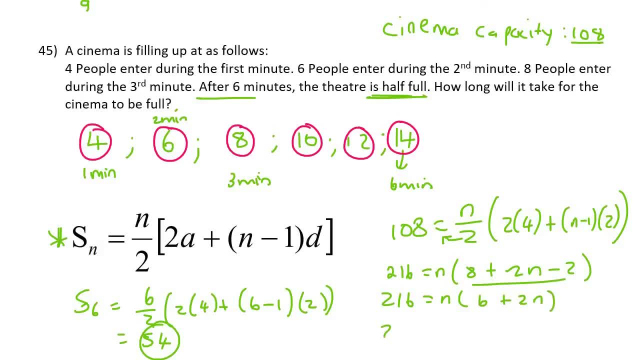 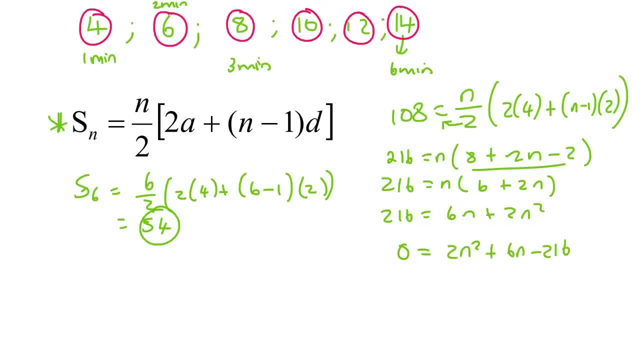 So it'll become 8 minus 2, which is 6.. I'm then going to multiply the end into the brackets And then it's a trinomial. So I'm going to keep the zero on the left and then I would use the quadratic formula to solve. 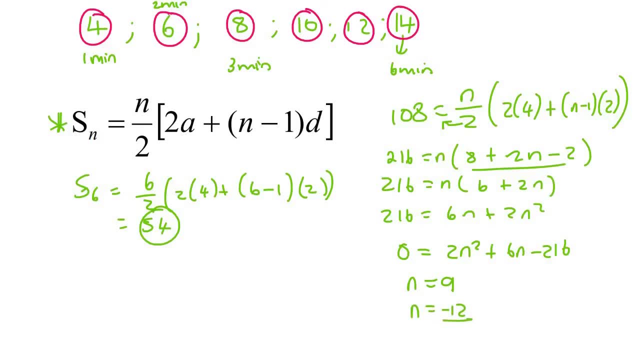 Would be nine or in would be negative 12.. But now you can't have a negative number as your position or as your minutes, So this one will be a no solution, And so the answer is going to be nine Minutes. That's how long it will take to fill up this entire cinema. 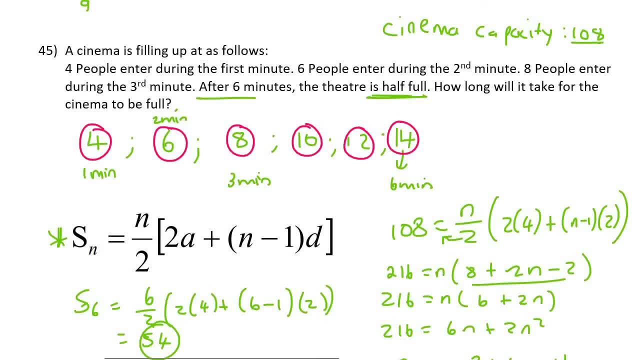 Some of you might be saying: but wait, If it takes six minutes to fill up halfway, Why wouldn't it be 12 minutes to fill up completely? Well, guys, as you can see, the people are filling up into the cinema faster and faster. in the first minute, for people walked into the door. in the second minute, six people have gone in, or six people went in. 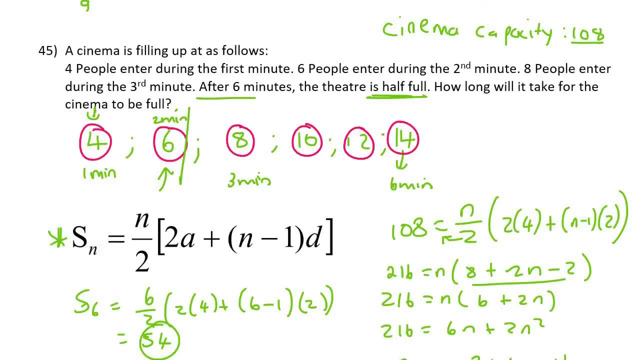 During that second minute. So now there's 10 people already. then in the third minute eight people walked in there. So there are more people Walking in as the minutes go by. in question 46. They tell us that this sequence is geometric. 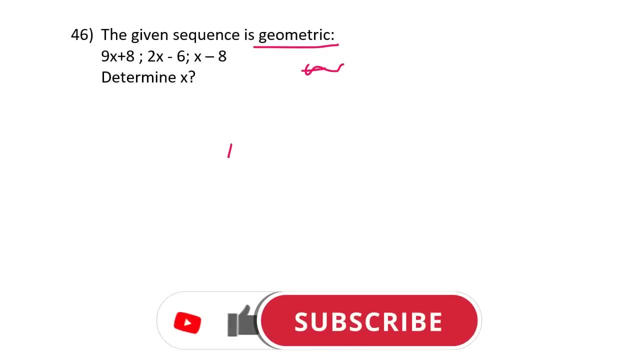 What that means is that we all. let me show you a normal geometric. Let's say we have 412 and 36.. That's geometric. Can we see? or let me show you that term 2, divided by term 1, is 12 over 4, which is 3. term 3, divided by term 2, is 36 divided by 12, which is 3.. 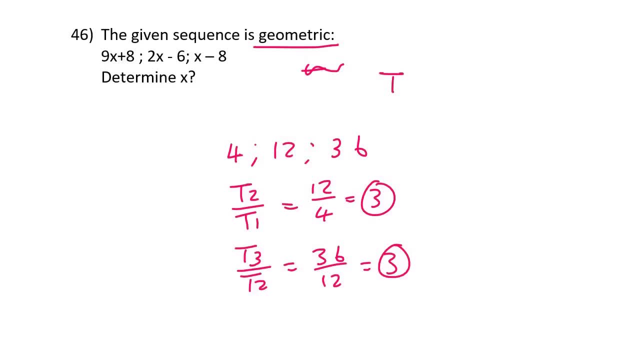 So it's the same. Remember that geometric patterns have a property that says term 3 over term 2 is the same as term 2 over term 1.. We just saw that happening now over here. So whenever something's geometric, this is true. 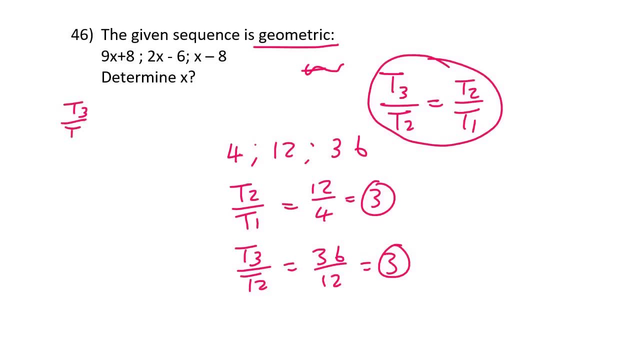 So we can say that over here. So we can say t3 over t2 must be the same as t2 over t1.. You can also switch this around, It doesn't really matter. You could have it the other way. You could say t2 over t1.. 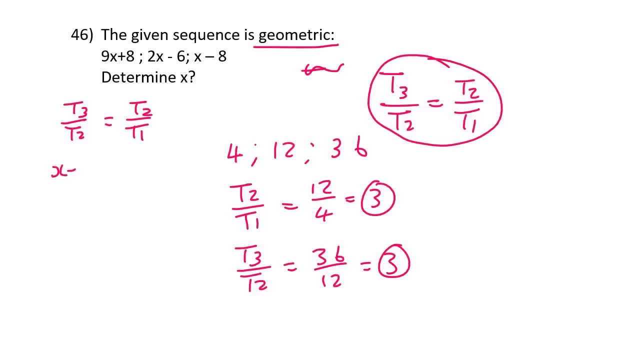 First: Okay. So now what we can say is: x minus 8 over 2x minus 6 equals to 2x minus 6 over 9x plus 8.. Now what we do is we cross multiply, So we'll end up with x minus 8 multiplied by 9x plus 8 equals to 2x minus 6 times by 2x minus 6.. 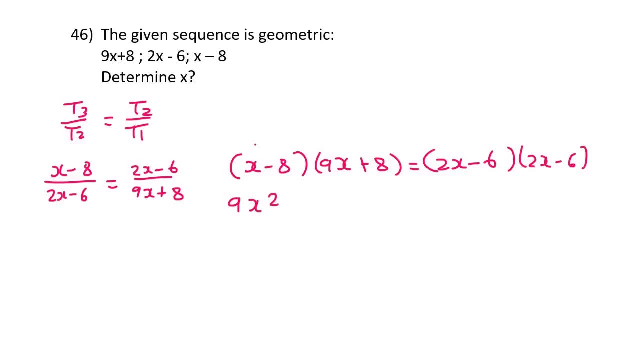 I'm now going to multiply out the left hand side, Which would eventually give a minus 64x in the middle. Of course there's two terms, but I've just put those together- and then minus 64. Then on the right hand side, you'll get 4x squared minus. 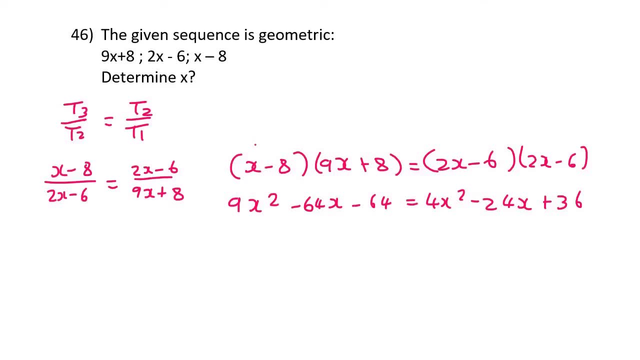 24x. I'm just doing everything in one step plus 36.. All right, I'm going to take everything to the left hand side. Then I'll use the quadratic formula, And so x would be 10.. Or x is negative 2.. 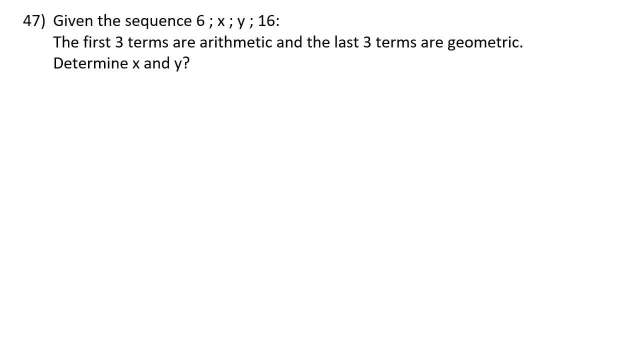 Question 47 is quite interesting because they give us. they said that the first three terms are arithmetic, So let's Do those. those are arithmetic. and then the last three terms, which is the x, the y and the 16.. Those are geometric. 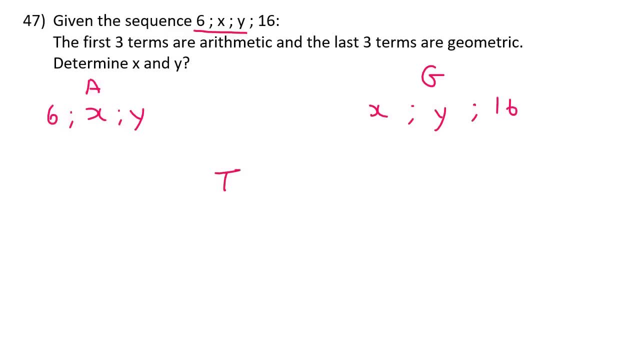 Now remember that when a sequence is arithmetic, you can say: t3 minus t2 equals to t2 minus t1.. Remember that is a property of arithmetic patterns. So here we can say: y minus X is the same as x minus 6.. 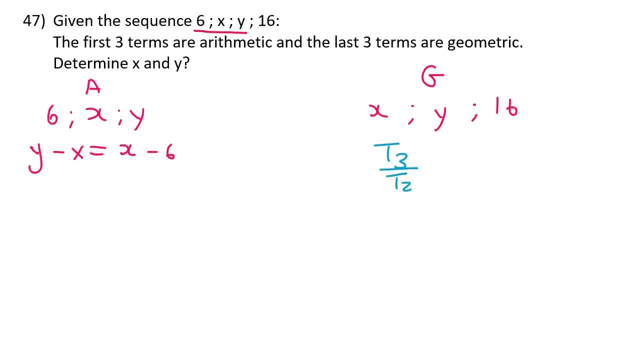 Then for geometric patterns, we can remember that t3 over t2 is always the same as t2 over t1. So we can say: 16 over y must be the same as y over x. Now what I'm going to do is I'm just going to try and neaten everything up. 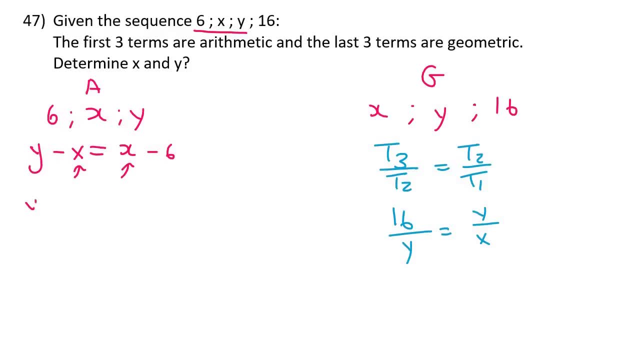 So these X's can go together. So we would actually get y equals to 2x minus 6.. And then on this side, over here I'm going to cross multiply So we'll get 16 x equals to y squared. Now we need to do some type of simultaneous equation. 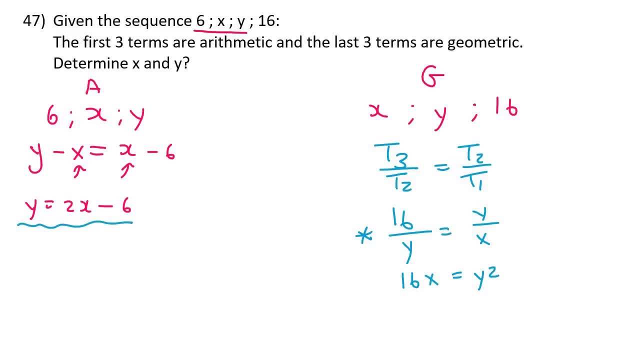 So I can see that y is 2x minus 6. So I'm going to put that over here. So we're going to get 16 x equals 2. And then this will become 2x minus 6.. Okay, so now I'm just going to multiply those two brackets out. 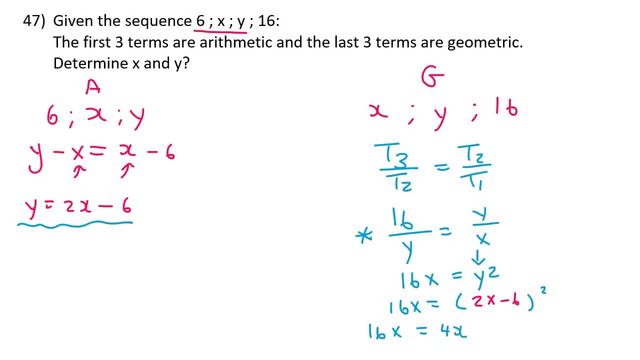 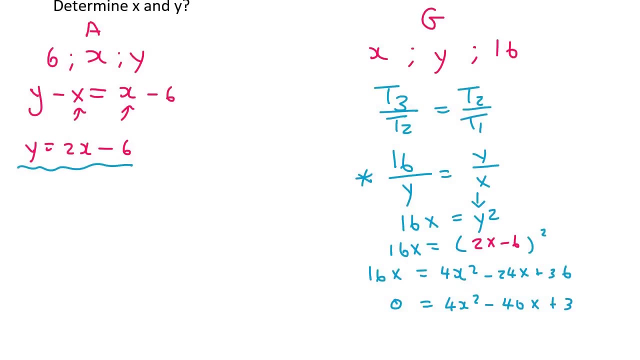 Remember that there's two brackets next to each other, So it'll become 4x squared minus 24x, after you've put all the terms together, plus 36.. Then I'm going to move everything to the right hand side, And so we're going to end up with minus 40x plus 36.. 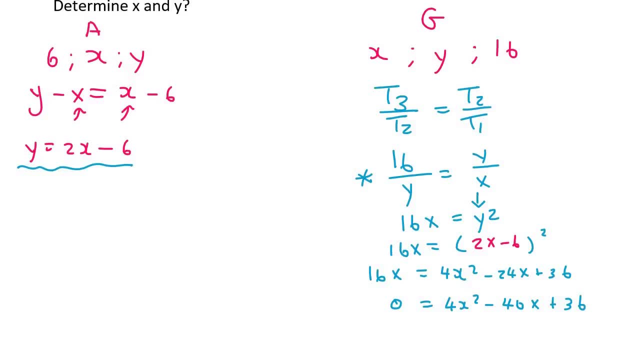 I'll use the quadratic formula there. You can try factorize if you want. I just usually go straight to the quadratic, And so X would be 9 or 1.. So now what we do is we come find the y values. So if x equals to 9,, then y would be equal to 2 times 9 minus 6, which is 12.. 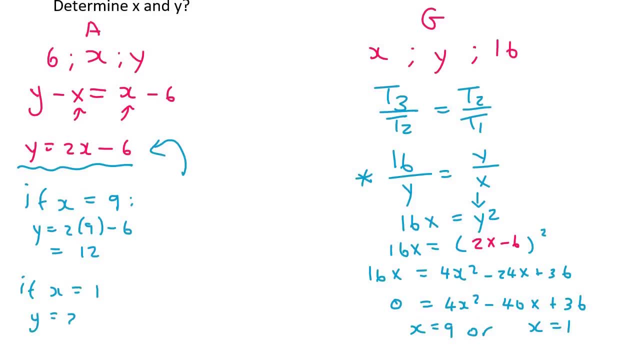 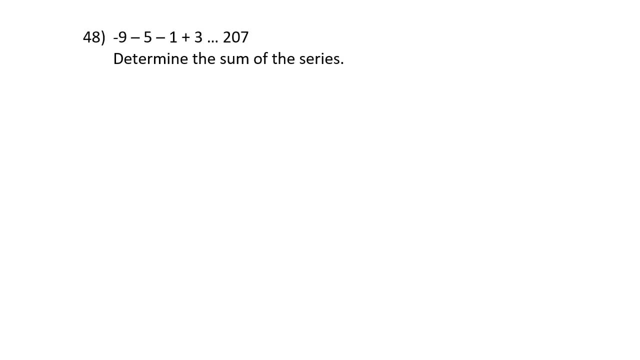 And then if x is equal to 1, then y would be 2 times 1 minus 6, which is negative 4.. In equation 48, we have an arithmetic sequence To go from minus 9 to minus 5,. you are adding 4.. 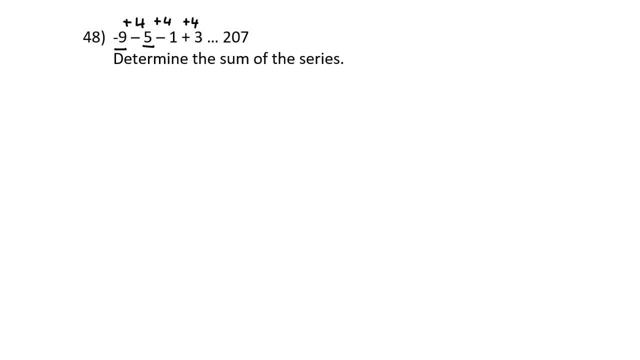 And then you keep adding 4.. Now it goes all the way up to 207.. So we need to find the sum formula of an arithmetic sequence, But the problem is we don't know how many terms we have. However, we do know that the last term is 207. 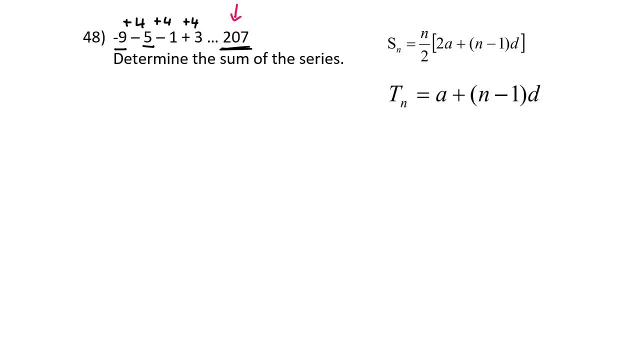 So we can use the TN formula, because that 207 is not a sum, It's an actual term. So we can say 207 is equal to a, which is minus 9.. Plus n, we don't know- And the common difference we said is positive 4.. 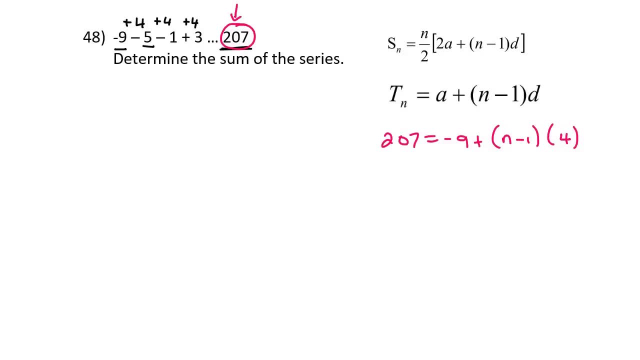 Then we can just solve this however you want. I'm going to take the 9 over Now. you could multiply the 4 in if you want, But I'm rather going to divide by 4. And so that's going to be 54 equals to n minus 1.. 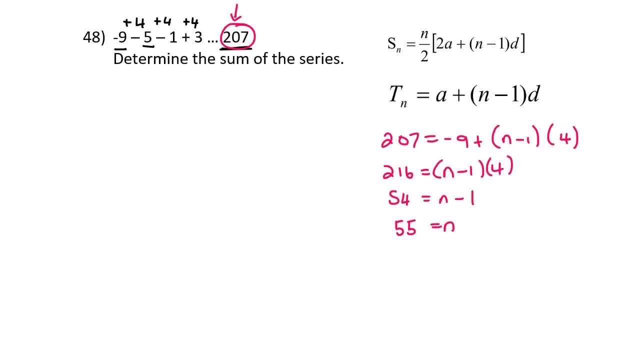 And so if you go solve, n is 55.. Now know that there are 55 terms, So then we can use this formula, And so that's going to be 55 over 2.. a is minus 9.. And the common difference is 4.. 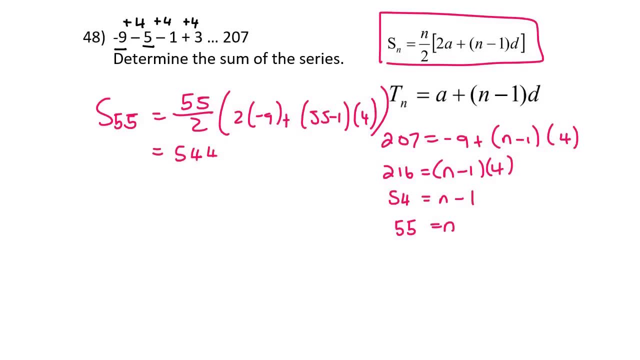 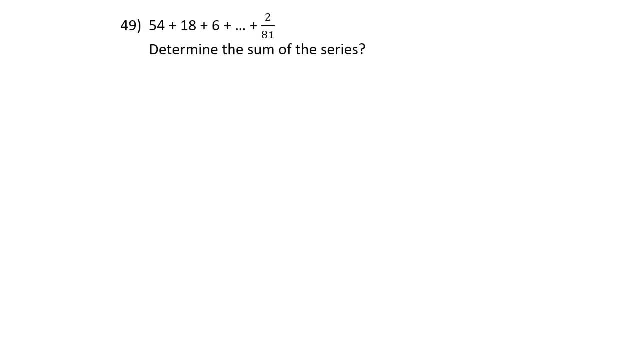 And so the sum of 55 terms is going to be 5,445.. If you look at question 49, it might be a bit difficult to determine if it's arithmetic or geometric, Because to get from 54 to 18, you're minus 36.. 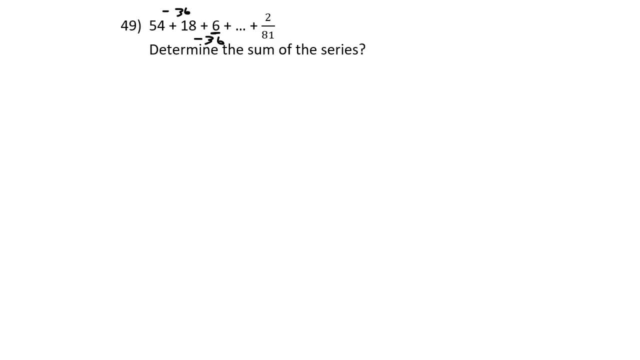 But then if you're minus 36 again, you're not going to get to 6.. So it's not arithmetic. So then what we could see is maybe it's geometric. To do that, we need to see the ratio And we have to see if the ratio stays constant. 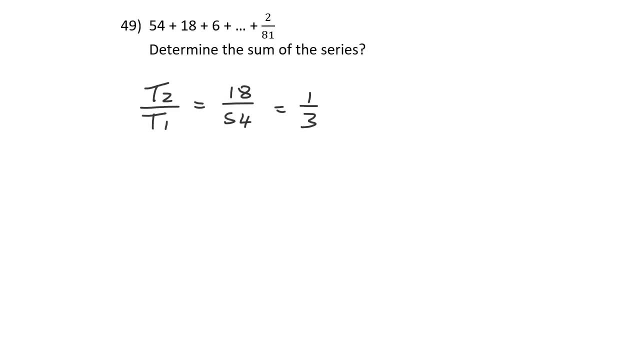 So we say 18 divided by 54, which is a third. Then we see if t3 over t2 is also a third. So we say 6 over 18.. And it is a third. So it's geometric where the ratio is a third. 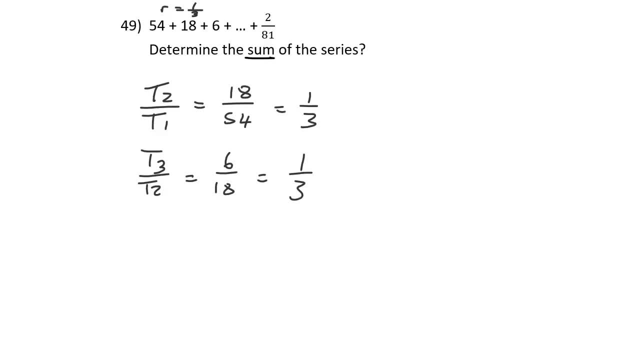 So it should be quite easy then, because we can just use the sum formula for a geometric pattern. However, we do not know how many terms there are. We do know that the last term is 2 over 81. So we can use the term formula. 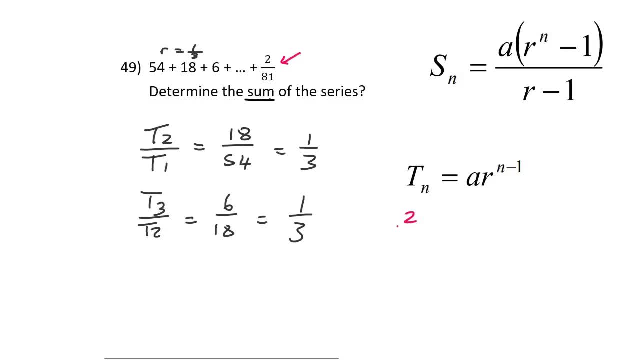 We know what the value of the term is: It's 2 over 81. But we don't know what term number it is. But if we could find that, then we know how many terms our sequence has. Now our ratio is a third. 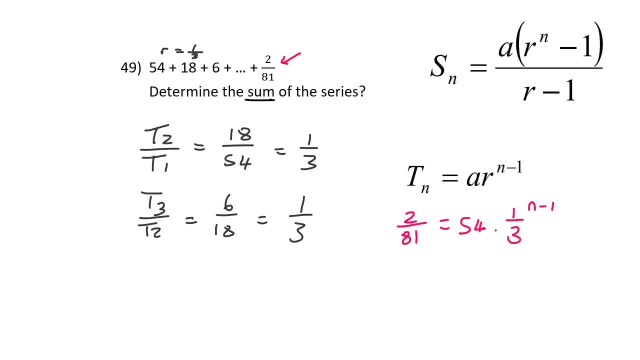 So we will just subtract that. So we subtract that. Now we know that if we do that, then we can get n minus 1.. To the n minus 1. Like that. Okay, So how do we solve this now? Well, what you do is you need to take this 54 over to that side by dividing. 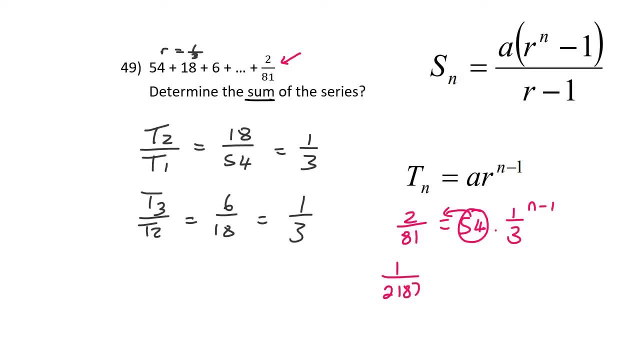 So it's going to be 2 over 81 divided by 54. Which is, 1 over 2187 equals to a third n minus 1.. Now, there's many ways that you can do this from this step, But I'm just going to use logs. 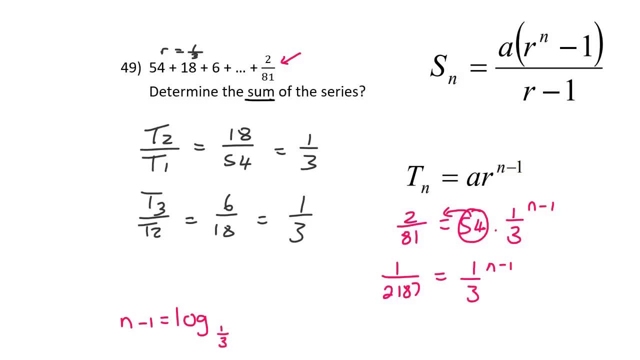 equals to log of a third, and then 1 over 2, 1,, 8,, 7.. So I'm going to type all of this on the calculator now, and that's 7.. So we can say that n minus 1 is equal to 7, therefore n must be 8.. 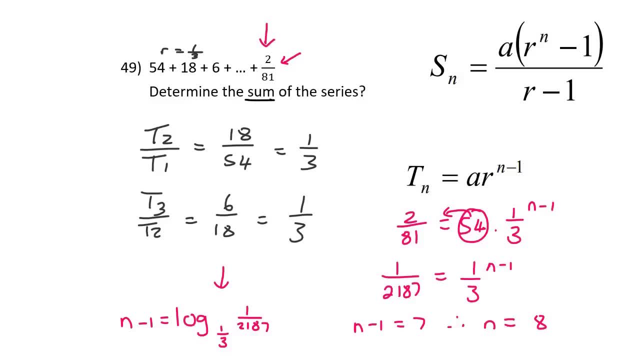 Okay, so we now know that this is term 8, but because it's the last term, it also tells us how many terms we have. So now we can come use this formula again. I'm going to use a different color now. So the sum of the first 8,. why do I use infinity? for that would be a. what did we say? 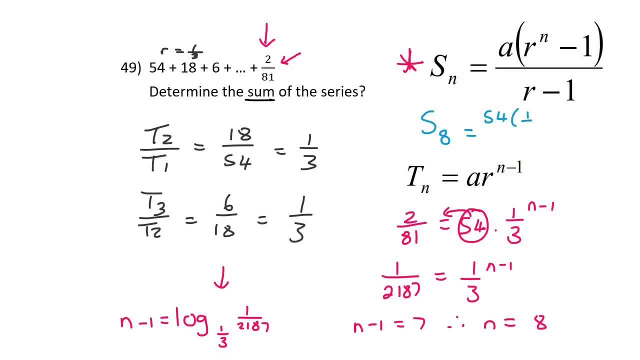 a was: Oh, it's 54. The ratio is a third. we have 8 terms, and then you just type it on the calculator, And so the final answer is going to be 80 comma 9,, 9, if you round to two decimal places. 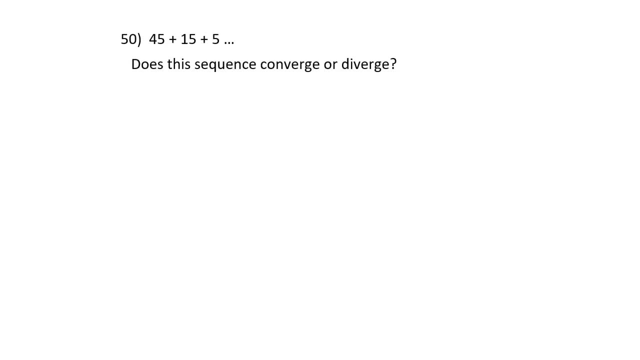 Question number 50. Does this sequence converge or diverge? Now, a converging sequence is one that eventually reaches zero. Now, for something to converge, it has to be geometric and the ratio must be between minus 1 and 1.. So, first of all, let's make 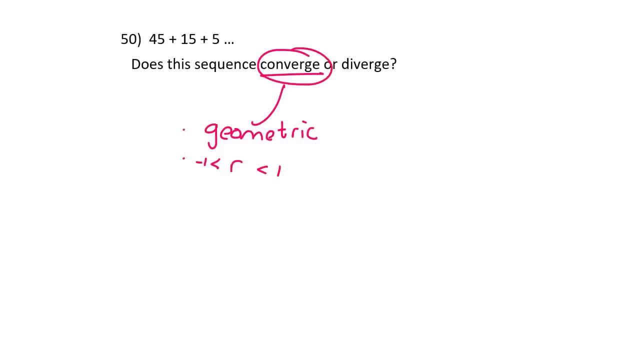 sure, if it's geometric, So you could minus 30 over here, but then if you minus 30 again, it's not going to work. So it looks like it's going to converge, but it's not going to converge, So you 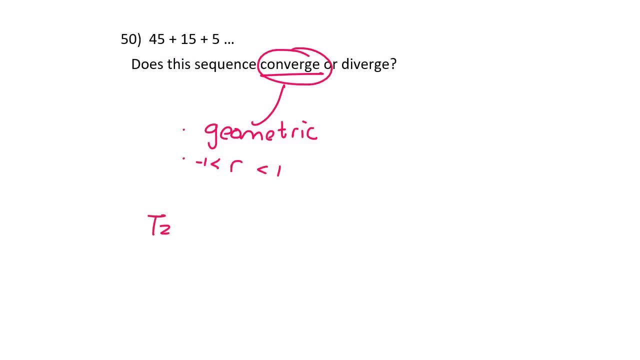 like it's geometric, but let's make sure, Let's see. what is T2 divided by T1? Well, that's 15 over 45, which is a third. Now, what is T3 divided by T2? Well, that's 5 over 15, and that's a third. 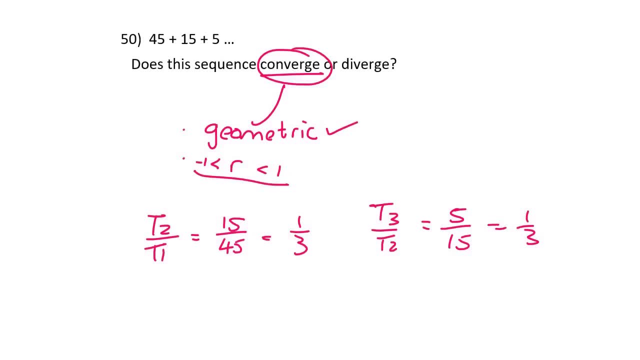 Okay, so it's geometric and the ratio is between minus 1 and 1, because it's a third, So this will converge. So, yes, it will converge, Verge.